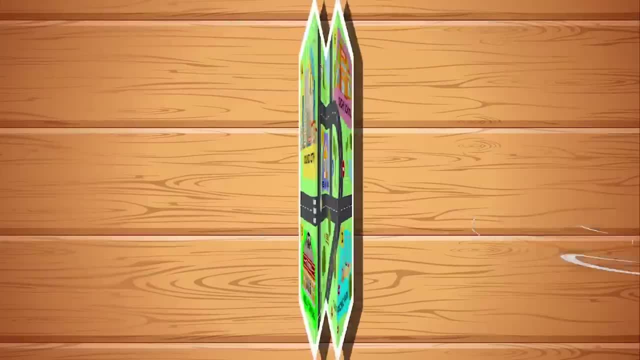 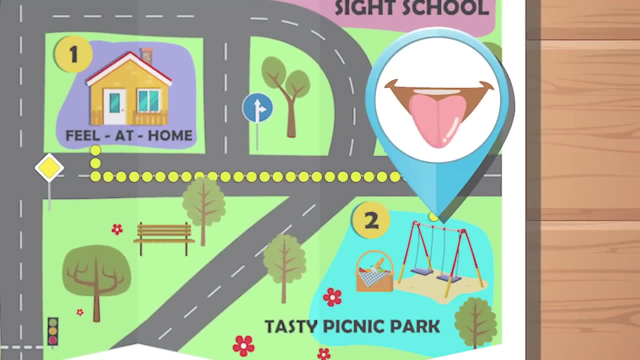 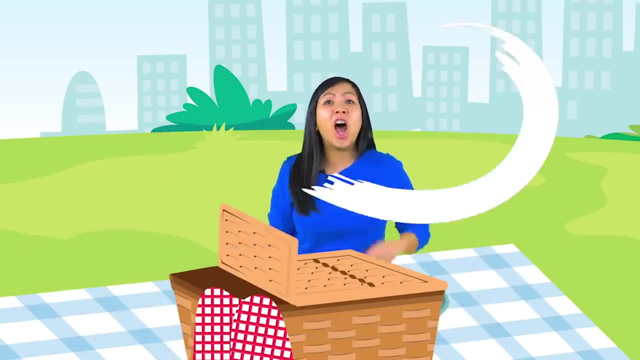 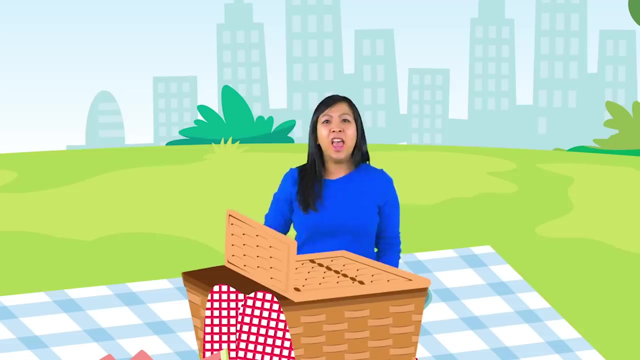 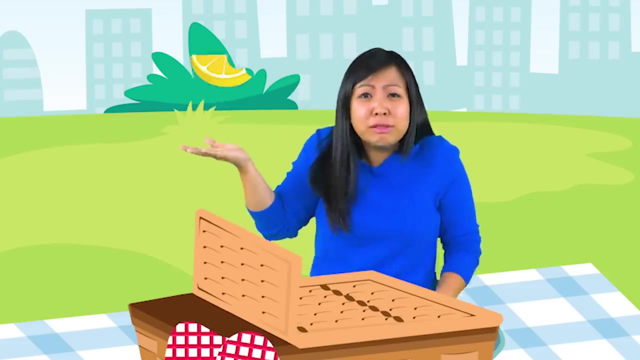 Whoa Oops For our next basic sense. how about we go on a tasty picnic? Our sense of taste allowed us to taste flavors. For instance, chocolate tastes sweet. Ooh, Lemons taste sour- Look so sour. And chips. 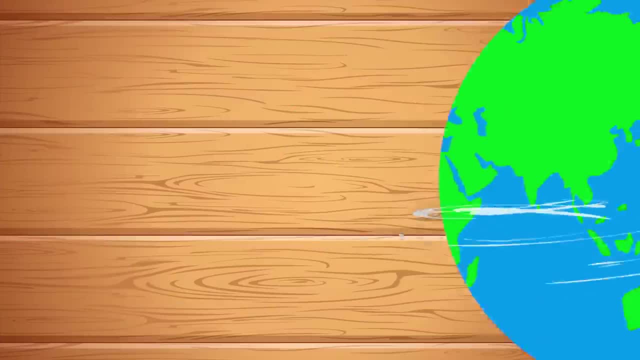 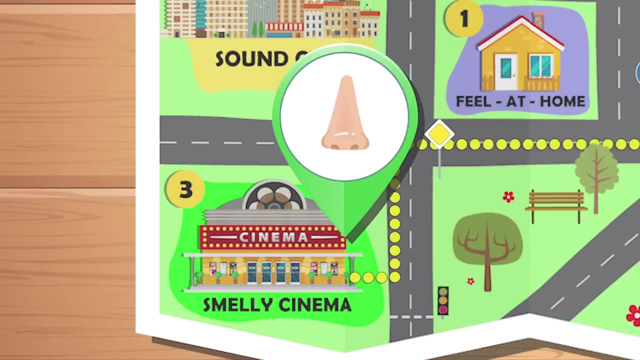 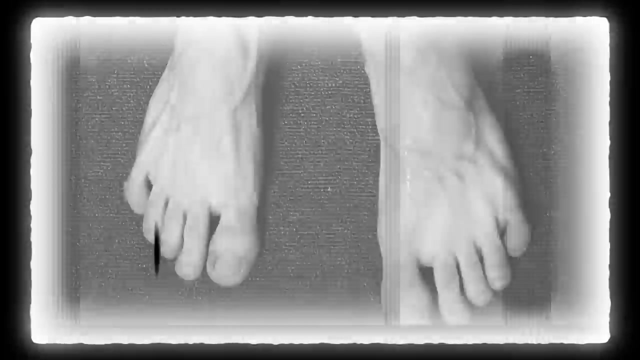 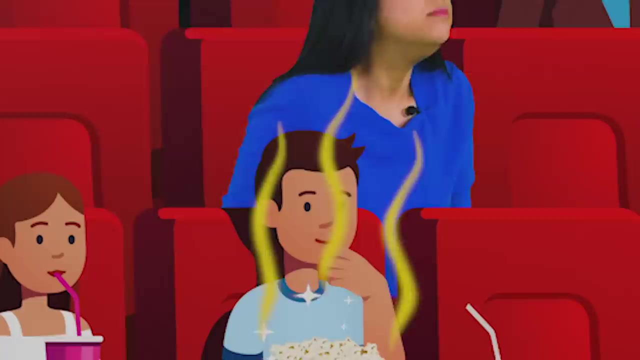 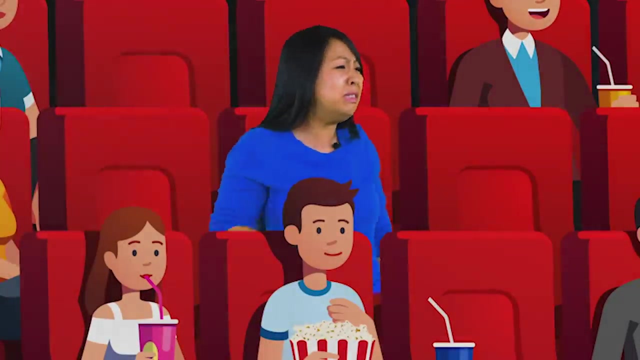 taste salty. Now let's check out a movie at the Smelly Cinema. Our sense of smell allows us to tell if there is good or bad. older, We can smell some mmm- delicious popcorn, And you can also smell someone stinking. 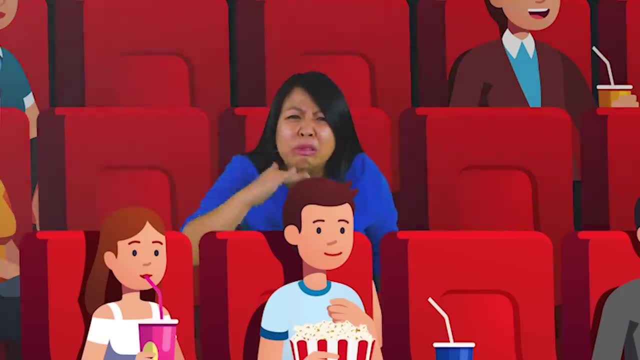 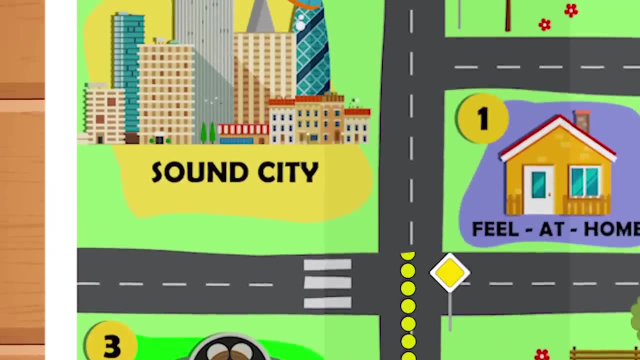 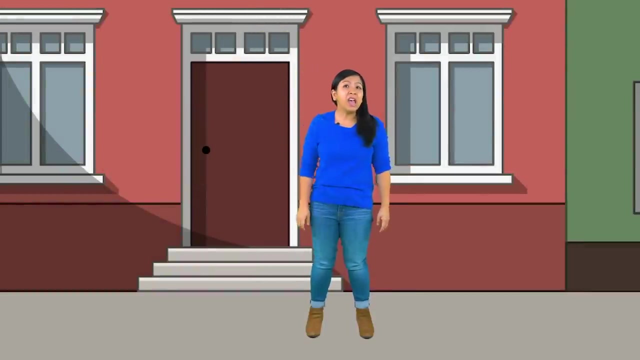 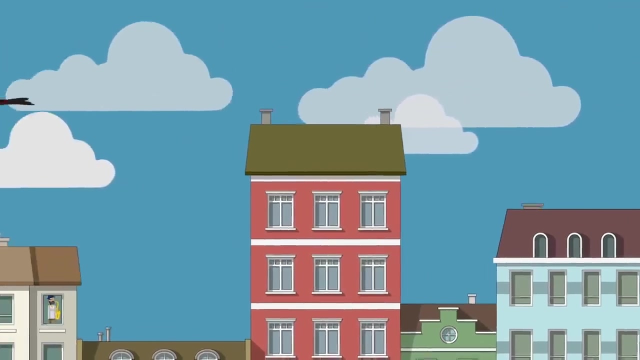 Stinky shoe: Ooh ew. I think we have smelled enough Time to head into Sound City. Our sense of hearing allows us to hear different sounds. If you hear chirping, a bird can be close by. You can also hear. 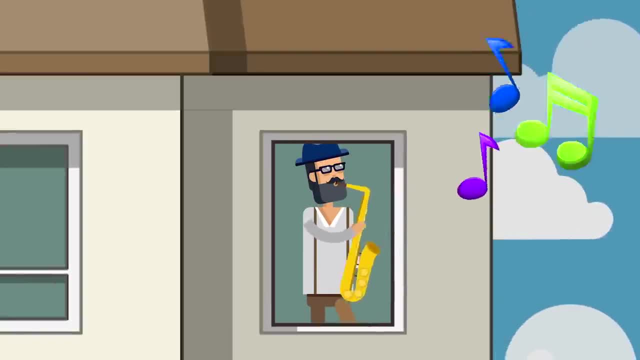 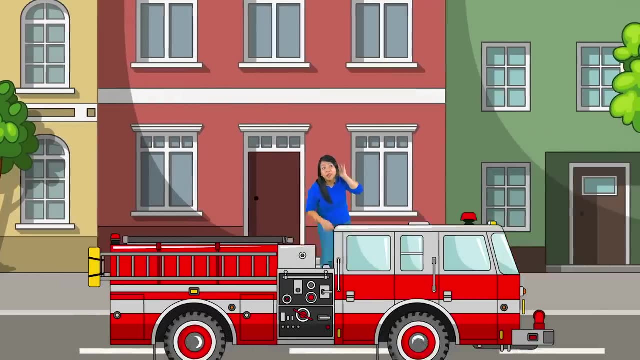 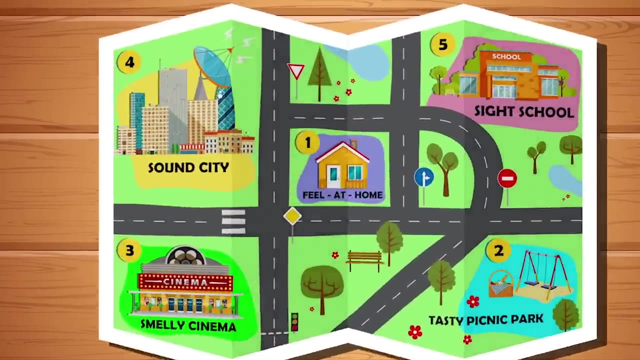 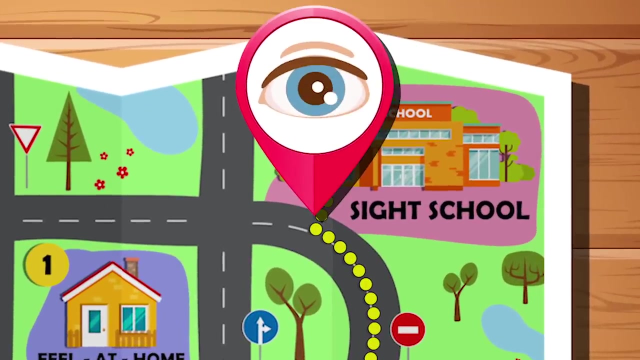 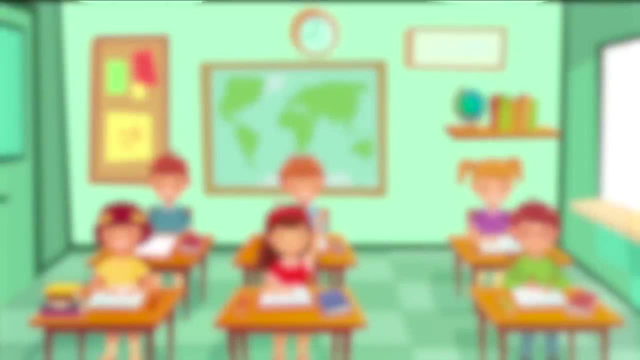 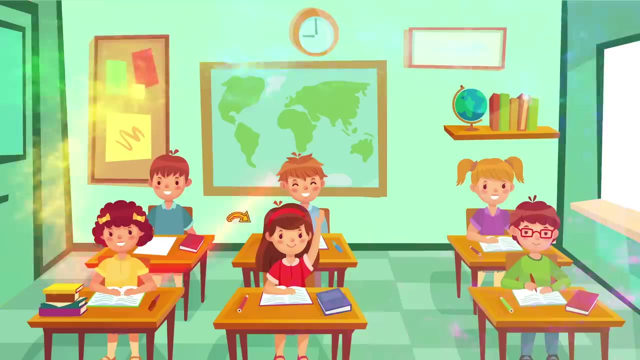 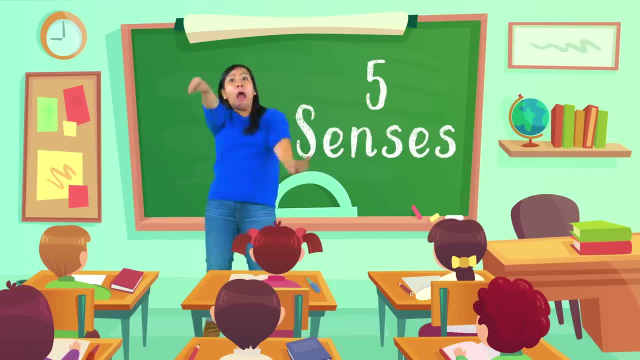 We can also see motion. We can also see motion, Like if someone tossed an apple to us. We can see when it's close enough to catch it. We can see when it's close enough to catch it. I caught it, I caught it. 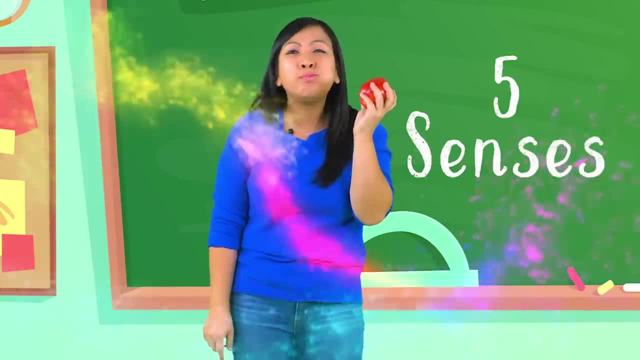 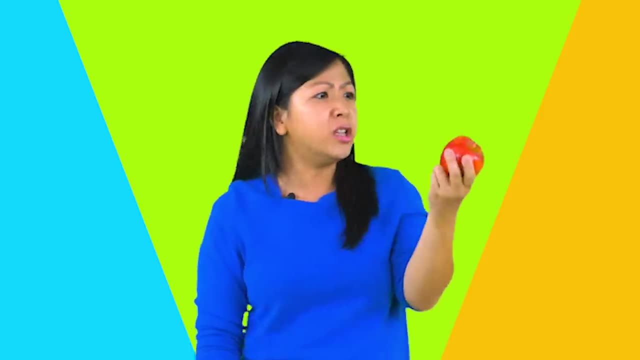 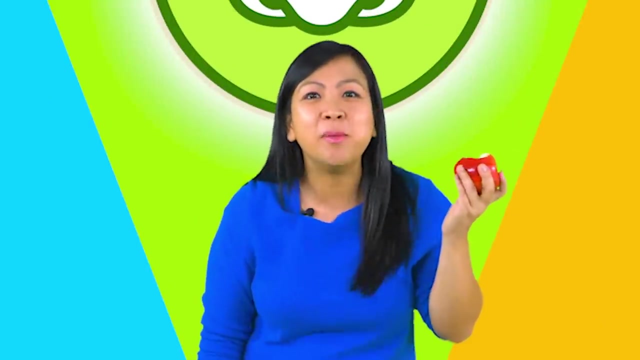 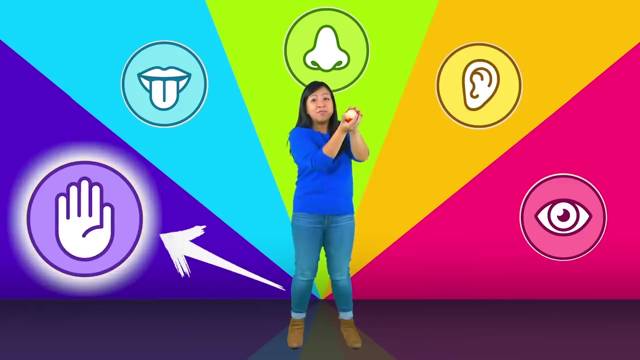 I caught it. Mmmm, Mmm. I use my sense of sight to see the apple. I can also see that it's red. My sense of smell is telling me that this apple smells so sweet. With my sense of touch, I can tell you. 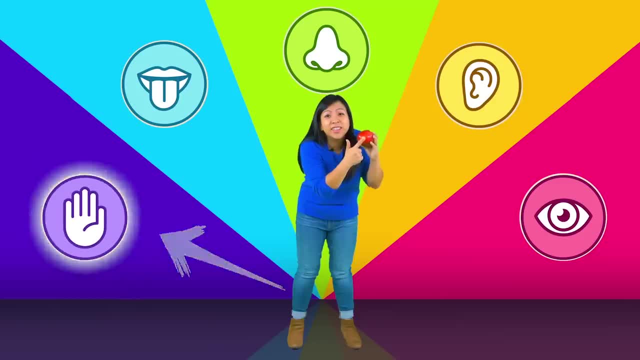 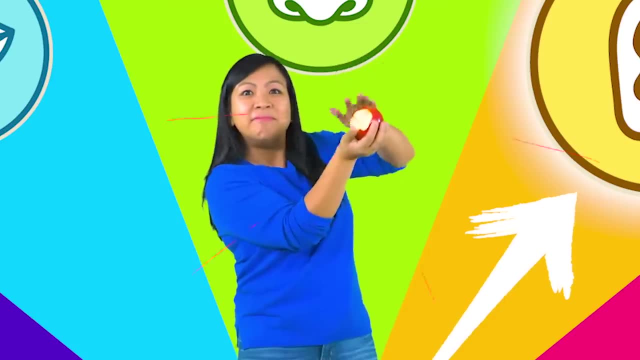 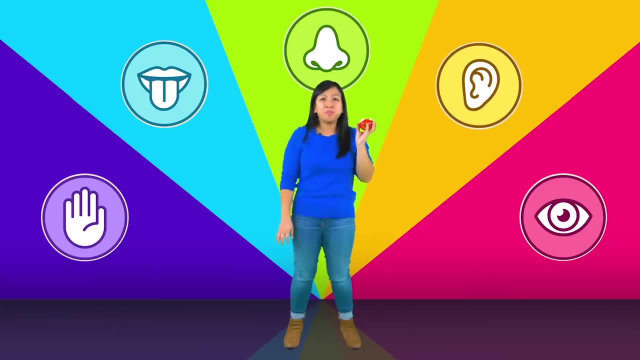 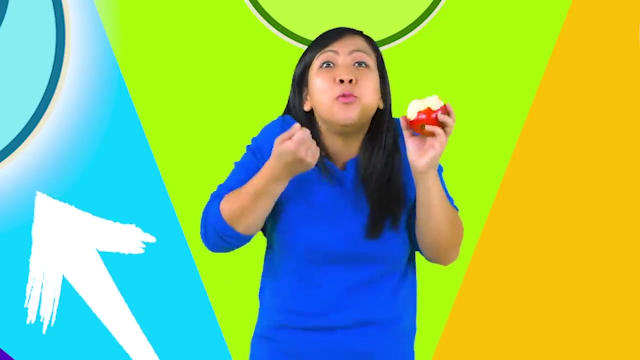 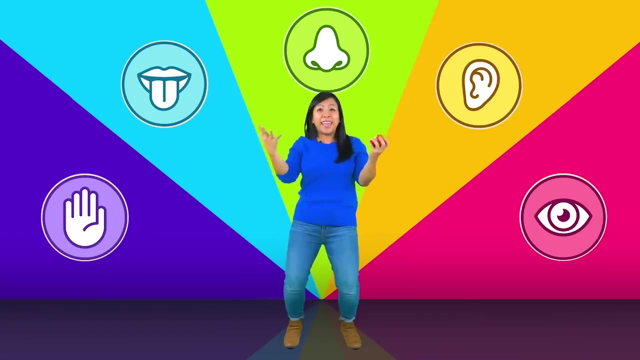 that the texture is smooth. It doesn't make any sound itself, but if I were to pat it it gives me a soft tapping sounds and with my sense of taste I can say that it tastes sweet. now let's put all our senses to a test with what's in the box challenge. let's go. I'm ready to test out my five. 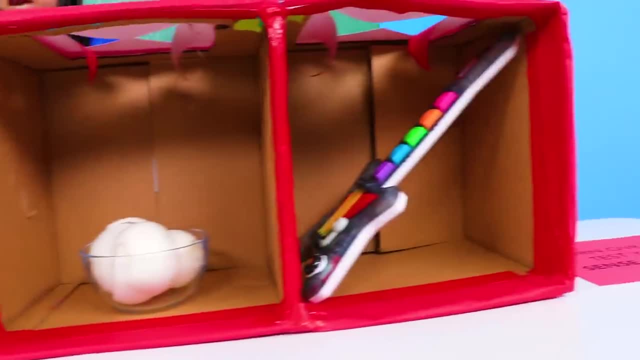 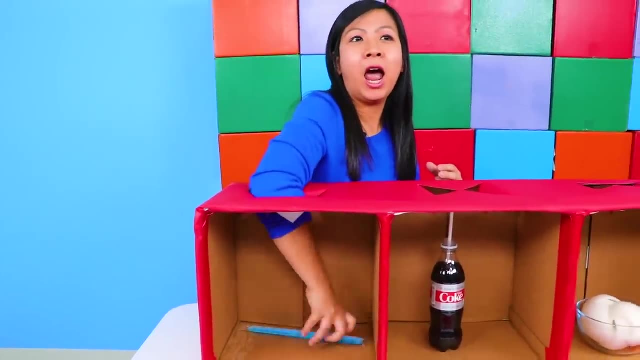 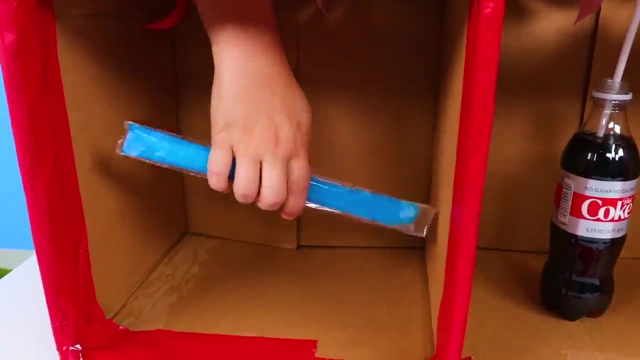 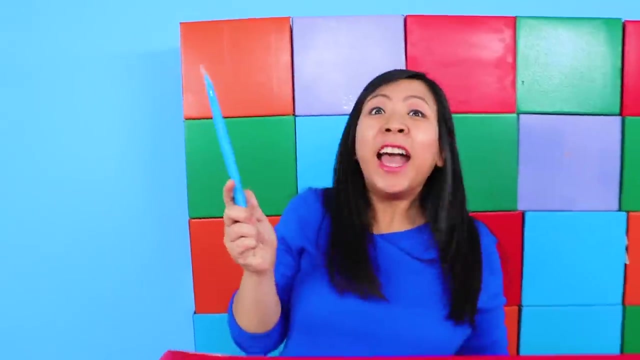 senses with what's-in-the-box challenge. let's get started, okay. whoa, it's cold and it's long. hmm, I think my sense of touch is telling me that it's a popsicle, am I right? all right, let's move on to the next challenge. 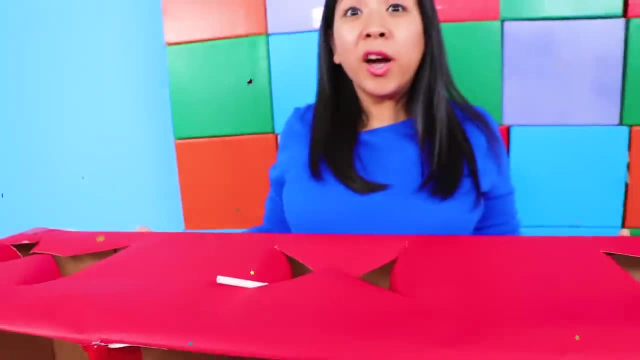 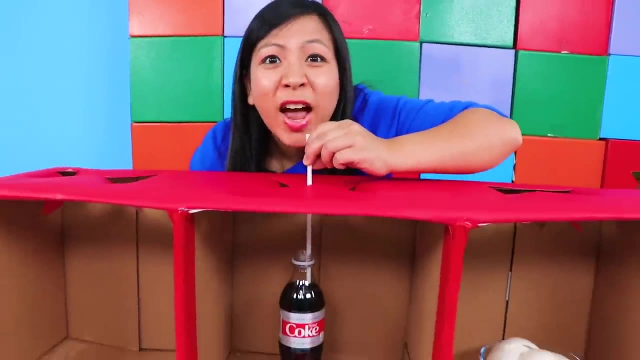 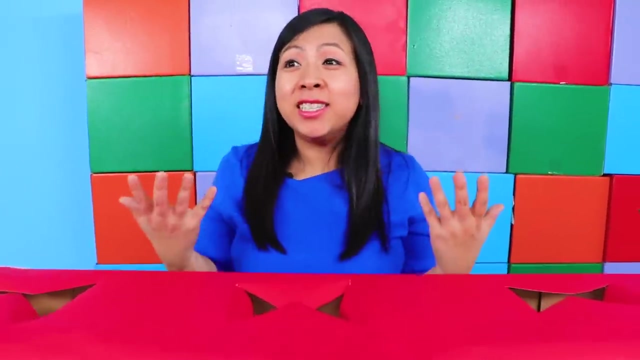 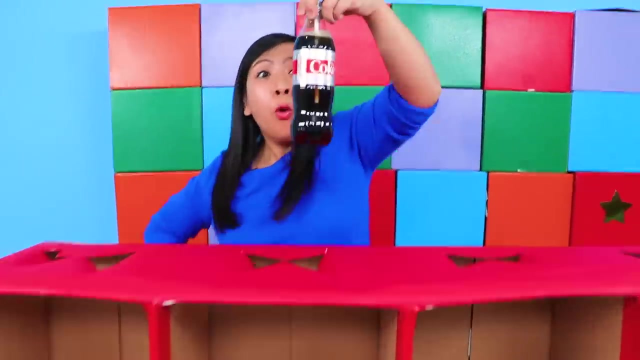 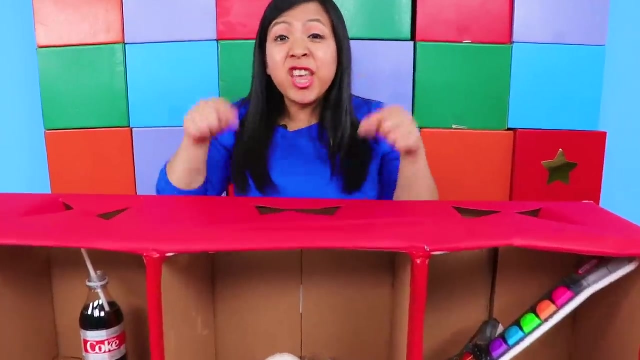 oh, it's a straw, so I guess this is testing my sense of taste. okay, let's try this. oh, my sense of taste is telling me that it must be Diet Coke. am i right? let's see? well, I am right. yeah, another point for me. so I'm thinking this one is testing my sense of smell. something very strong, I. 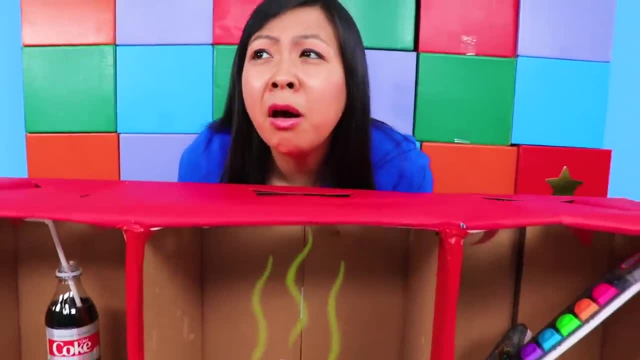 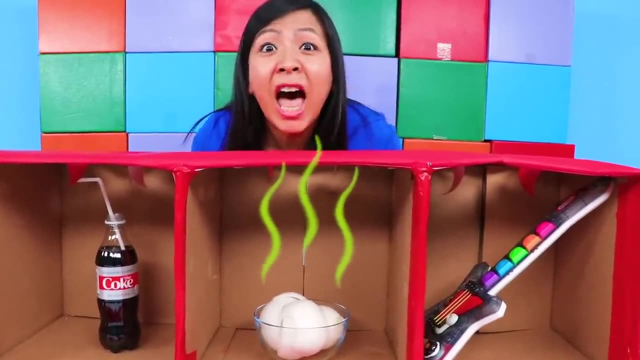 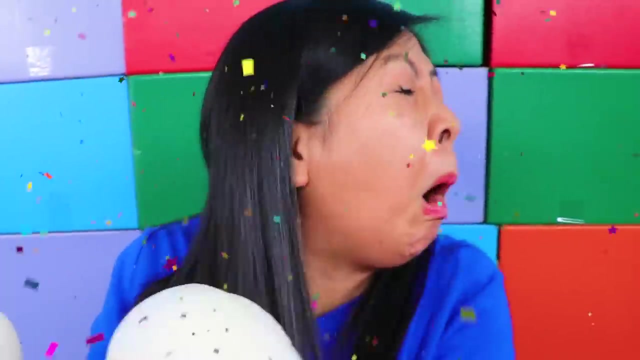 can smell it, let's see. um, definitely not broccoli. I think it is onion. am i right? it is onion? okay, let's see what's in this box here. oh, there's so many buttons. okay, let's see what's in this box here. oh, there's so many buttons. 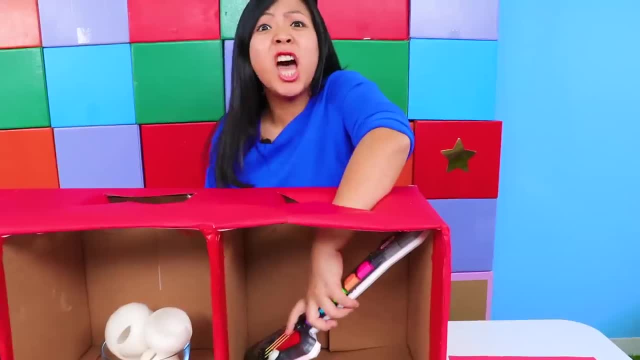 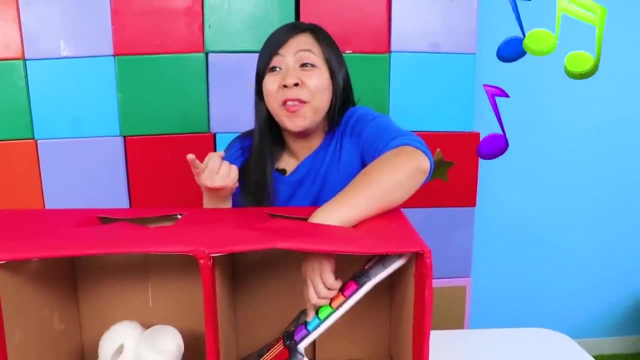 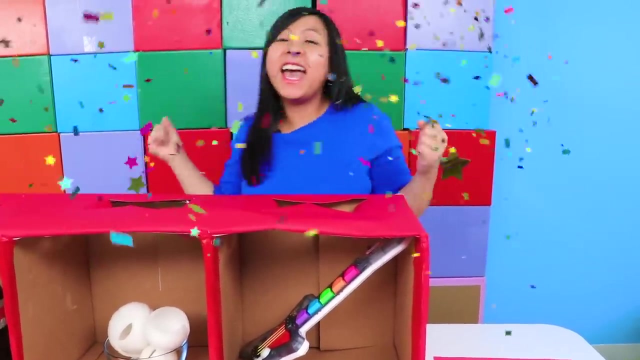 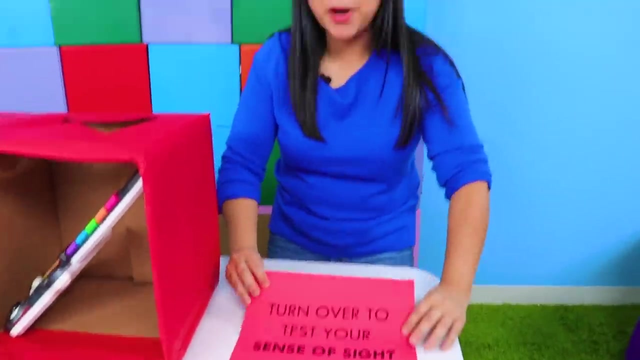 oh, there's so many buttons, buttons. maybe it's testing my sense of touch. all right, let's press a button and see, i know this one, it's a nursery rhyme. do you guys know this one? it's old mcdonald had a farm. okay, last one, i'm finally able to flip it over. oh, i think this is testing our sense of. 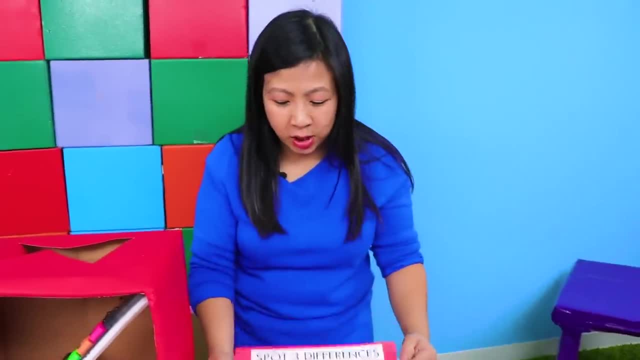 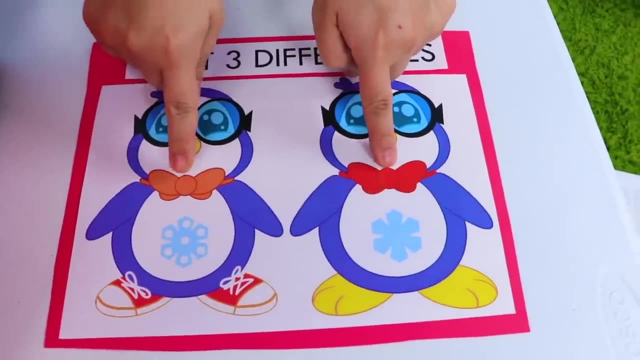 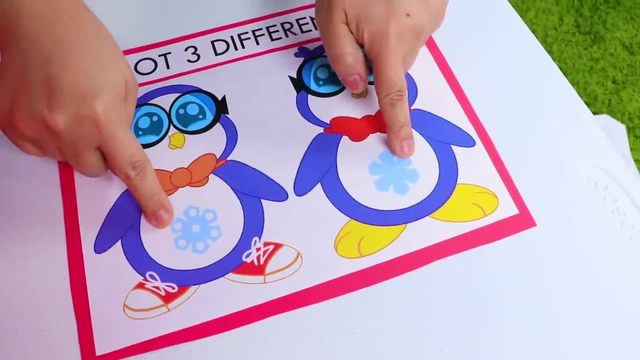 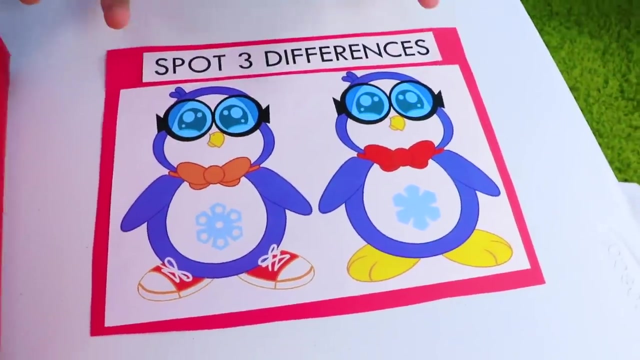 sight. it says: spots the difference. okay, do you guys see anything different? look his bow tie. they're different color. one is orange and one is red, anything else. his snowflakes, they're different too. one is a solid and one has circles in them, anything else? oh, look his shoe. one pic has no shoe and the 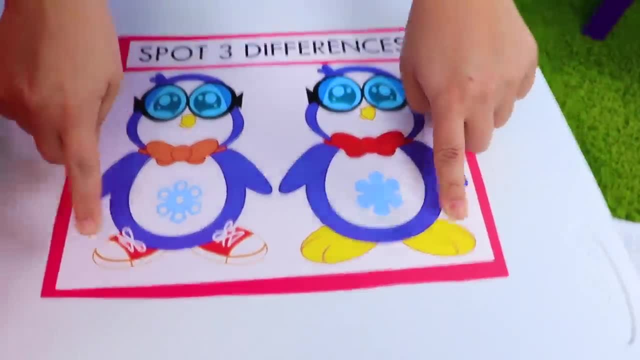 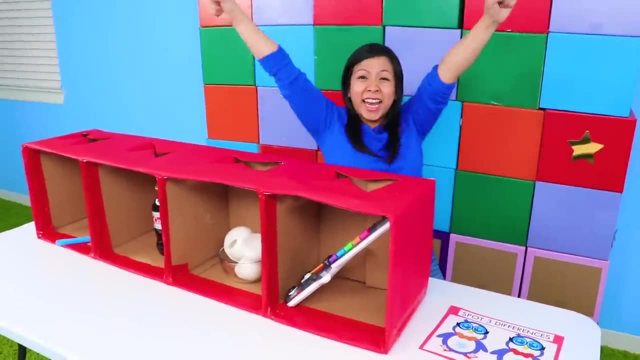 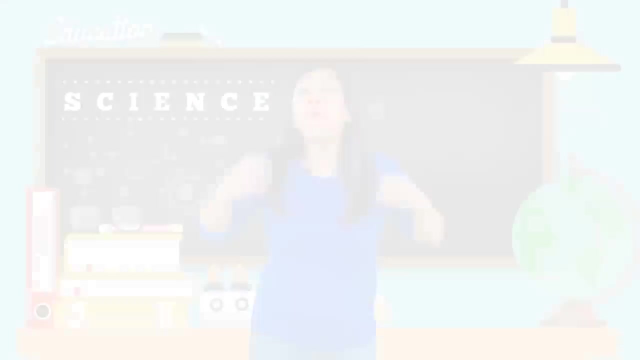 The other one has cool sneaker shoes. Well, we did it, you guys. We used our five senses to complete the What's in the Box challenge. Now that we know all about our five senses, let's do a pop quiz. Question number one: 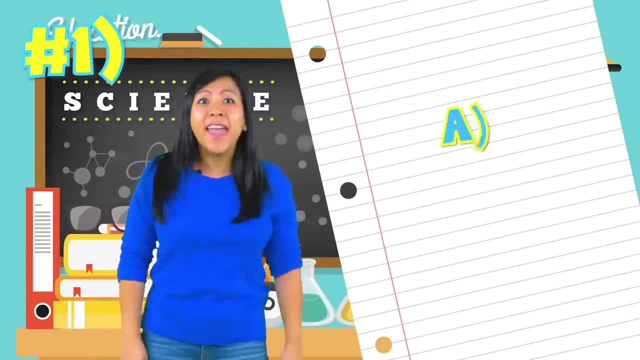 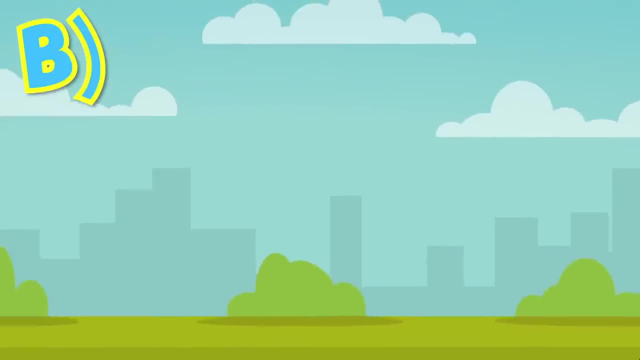 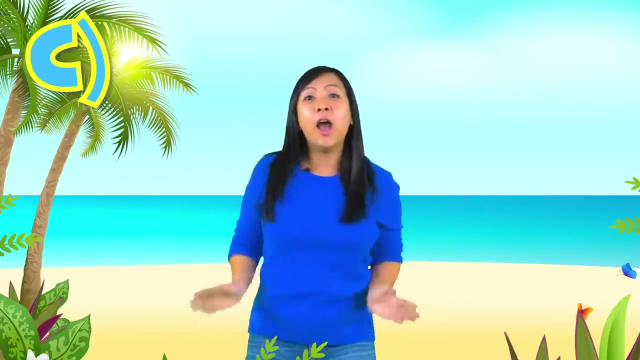 Why do we have basic senses? Is it because of A- to experience the world around us. Or is it because of B- to ride a bike? Or is it because of C- to go on vacation- Hawaii. Did you get the answer? 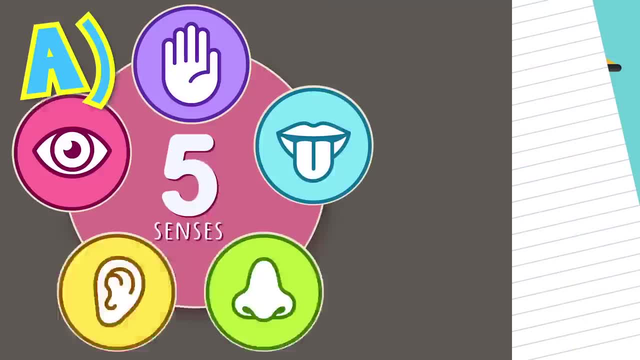 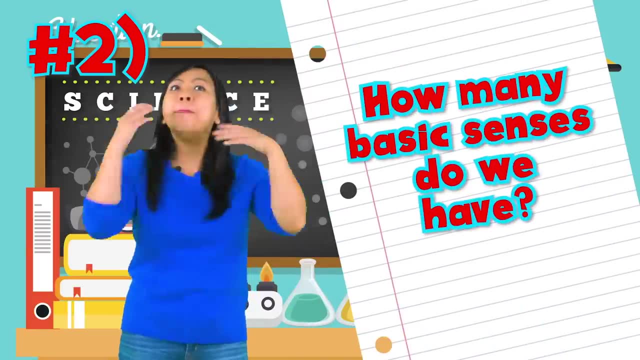 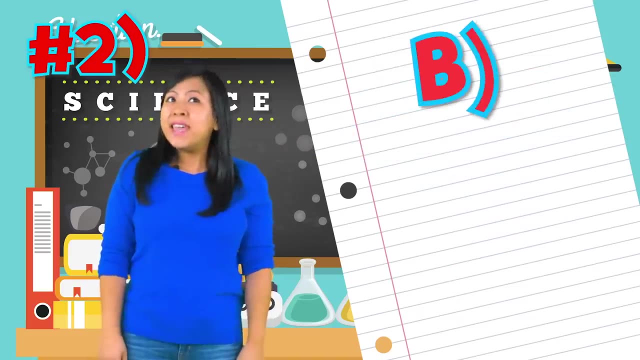 It is A. We have basic senses so we can experience and enjoy the world around us. Question number two: How many basic senses do we have? Is it A- 50? Or is it B- five senses, Or is it C- a hundred senses? 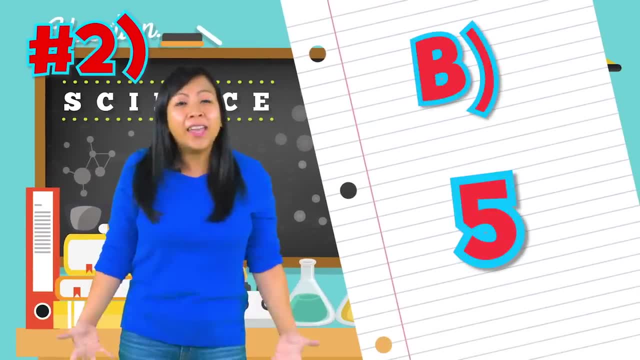 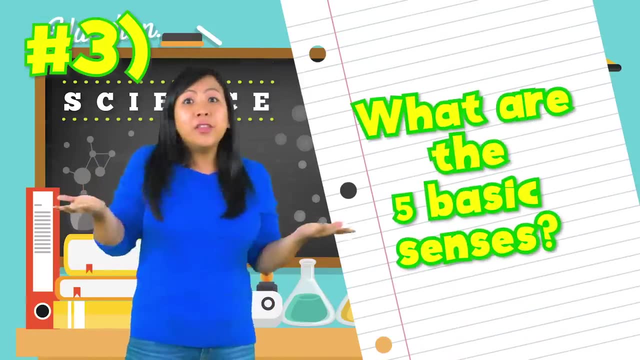 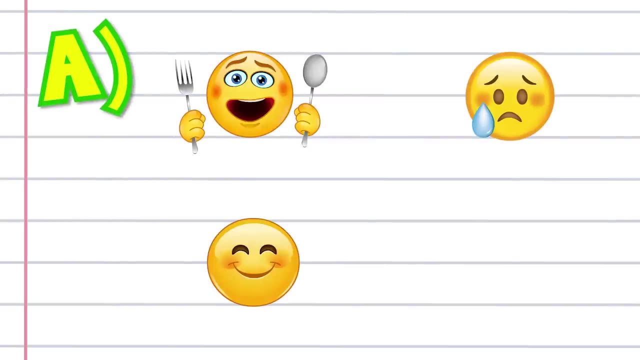 Did you know the answer? It is B five. We have five basic senses. Question number three: What are the five basic senses? Is it A hungry, Bad, Happy, Sneezy, Grumpy, Or is it B touch? 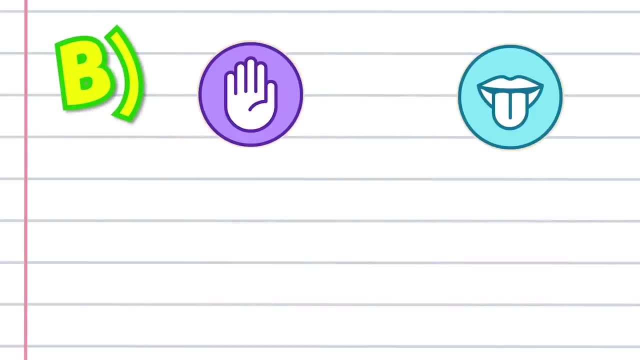 Taste Smell, Hearing And sight. Or is it because of C, math, science, reading, gym and history? Did you get the answer? What are the five basic senses? It is B: touch, Taste Smell. 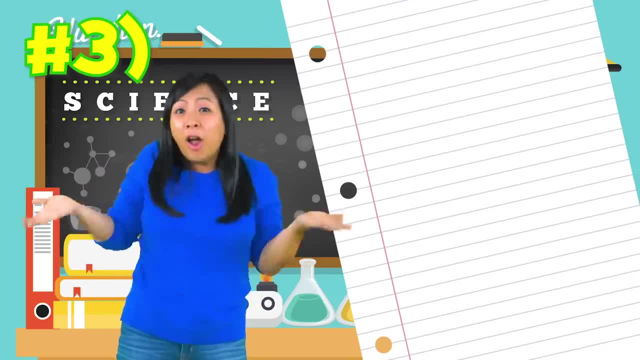 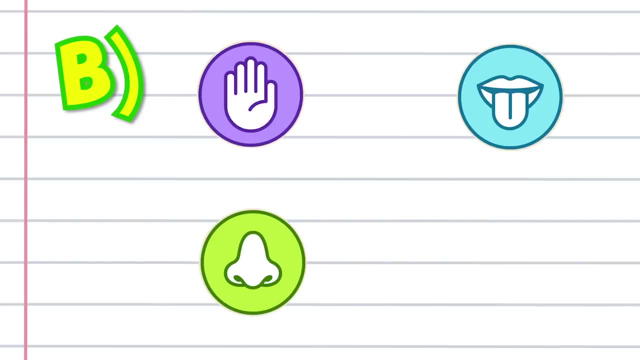 Hearing And sight, Or is it because of C, Math, Science, Reading, Gym And history? Did you get the answer? What are the five basic senses? It is B, Touch, Taste, Smell, All right, there, it is our pop quiz. 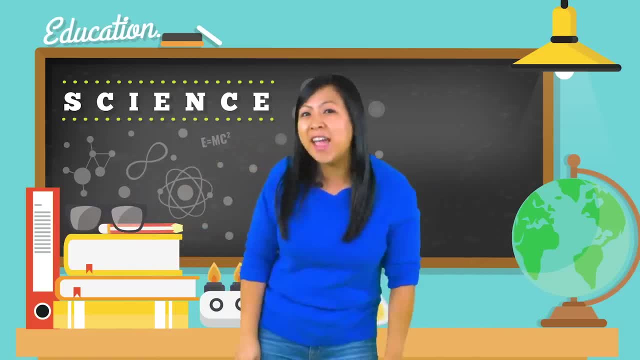 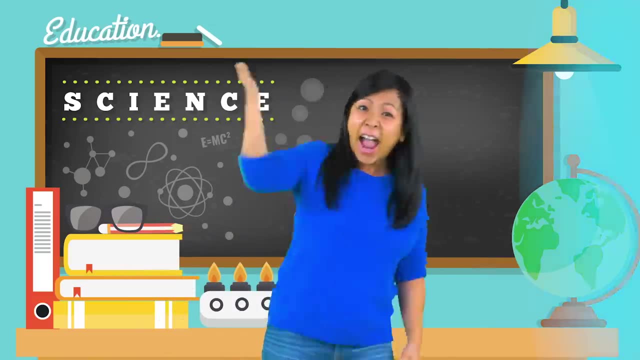 Good job if you get it right, and if you didn't, it's okay, You can try again next time. For now, let's go tell Ryan about everything that we learned about our five senses. Let's go. So, Ryan, those are your five senses. 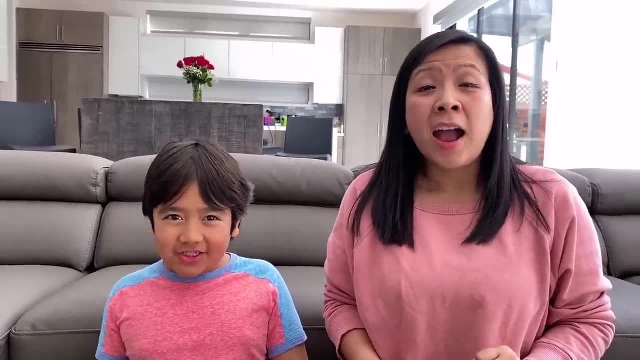 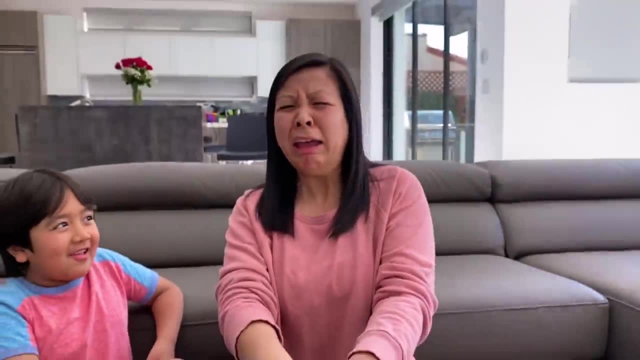 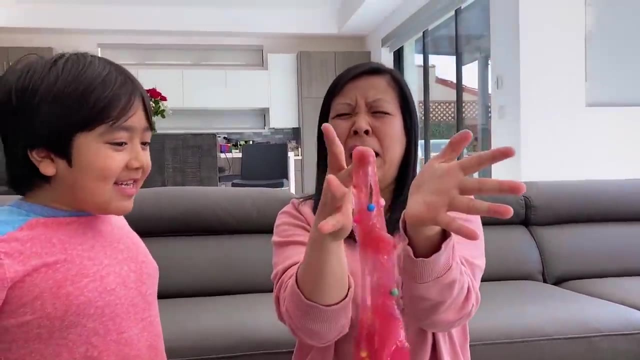 Mommy, it's your turn to use your sense of touch. Close your eyes, Okay, okay, Okay, gotcha. Oh, what is this? It's so cold, It's slimy. You're correct, it's slime. 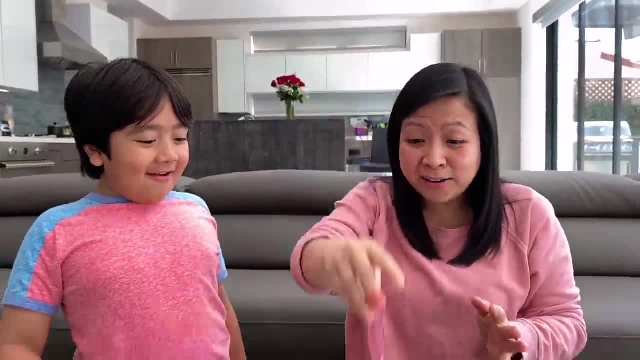 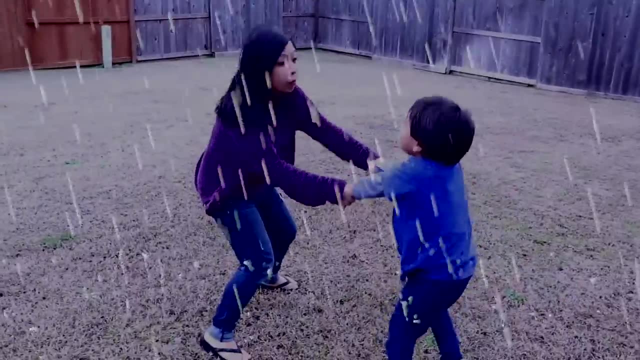 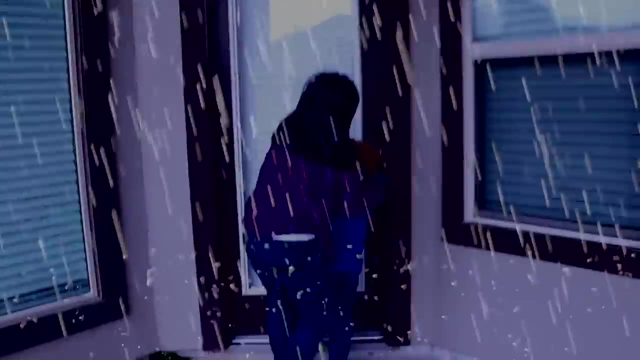 Oh, I was right. Whoa, Okay, guys, thank you so much for watching Ryan's World Video. Ah, Mommy, it's raining. Oh, no, it's raining. Mommy, we gotta get out. Ah, Ah, it's raining. 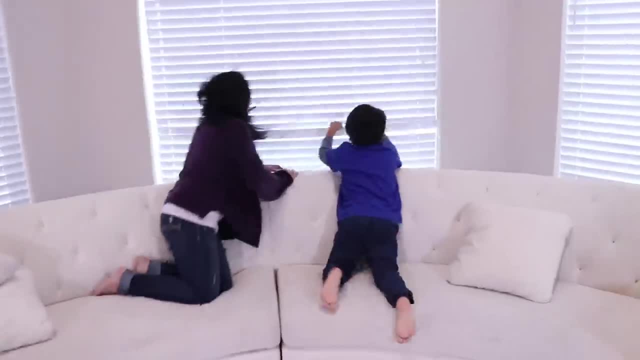 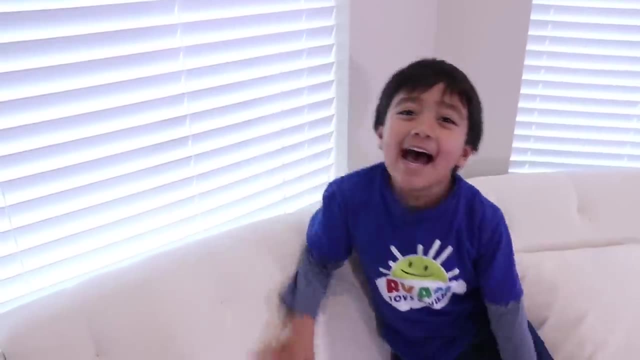 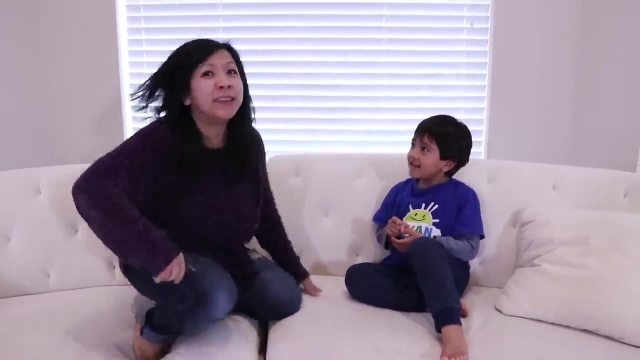 Oh, Oh, Mommy, it's raining a lot, Yeah, but do you know what happened after the rain? A rainbow, But Mommy, how does a rainbow form? Ah, good question, I'm right back, Whoop. 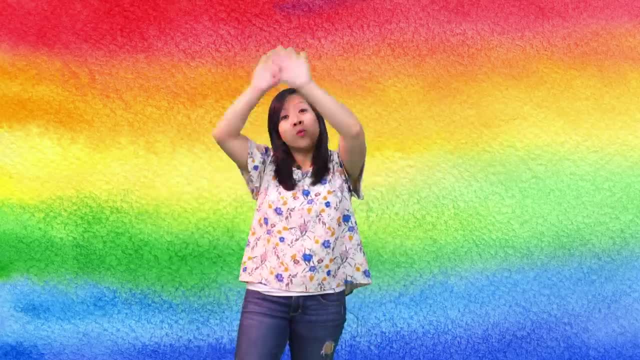 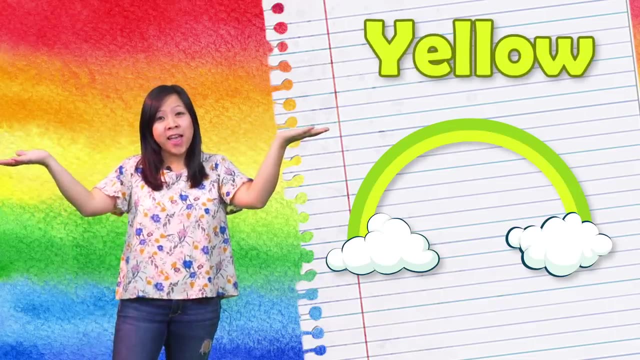 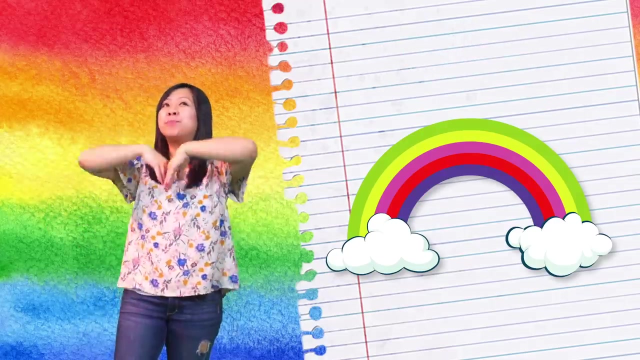 Where did Mommy go? Did you know that rainbows have seven colors? There's green, there's yellow, there's violet, there's red, there's indigo, there's blue and orange. Wow, that's a lot of colors. 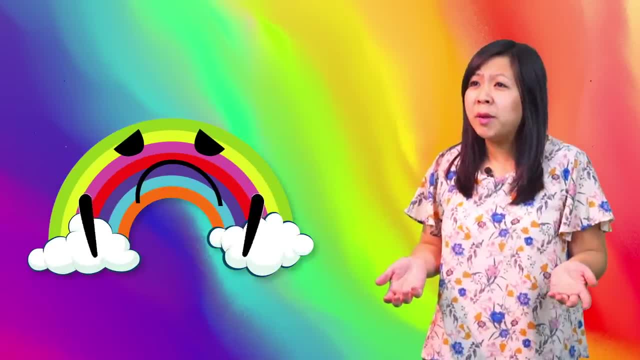 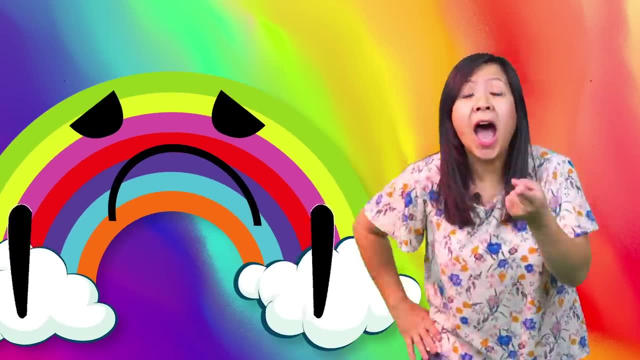 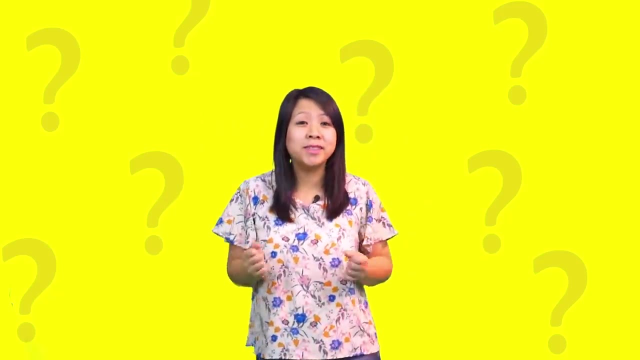 Seven Wha. what's wrong? rainbow- Oh, the rainbow doesn't look too happy. Wait a minute. Something doesn't look right with the rainbow. I know order. did you know that the colors of the rainbow are always in the same order? 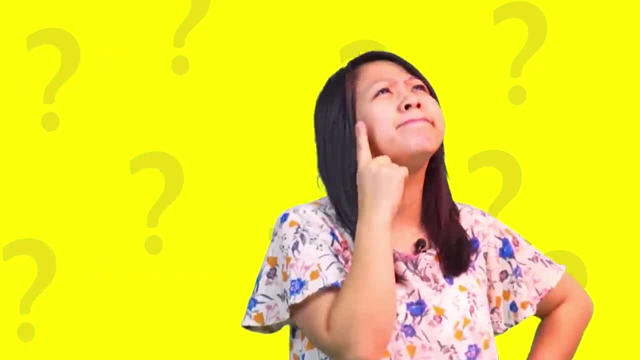 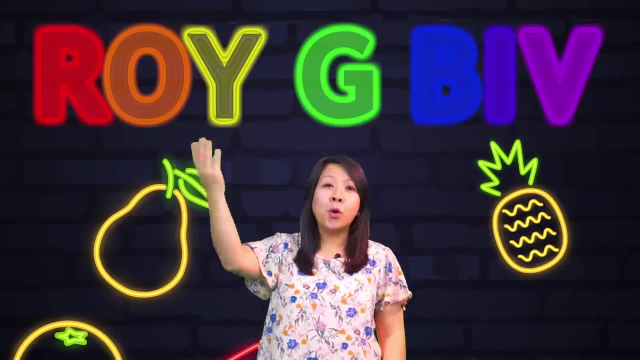 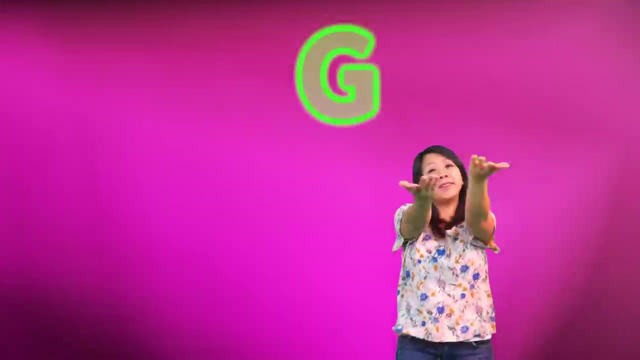 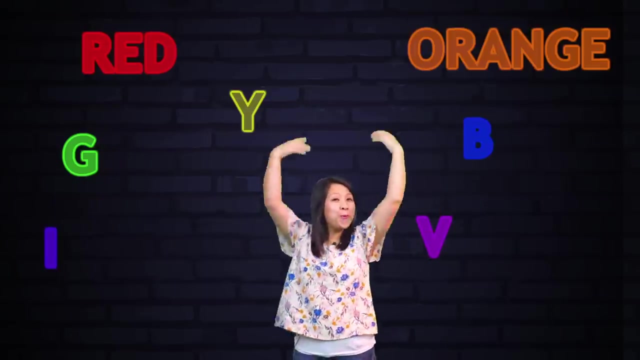 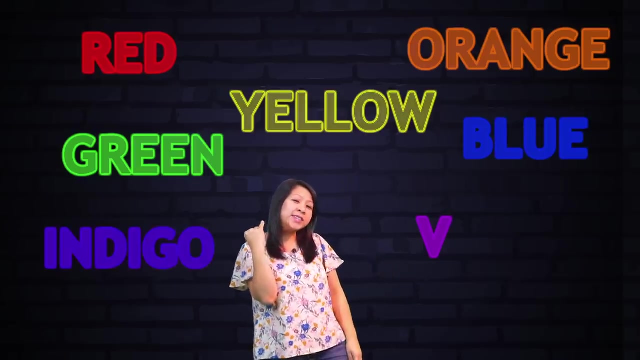 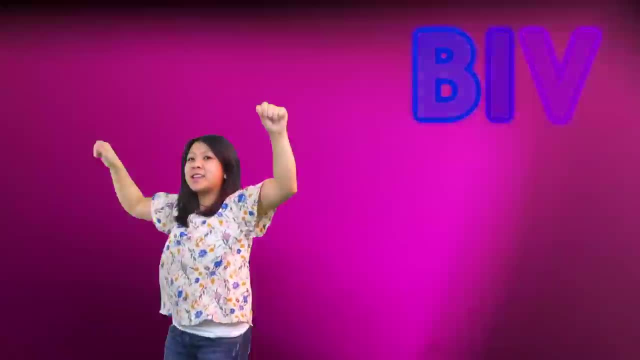 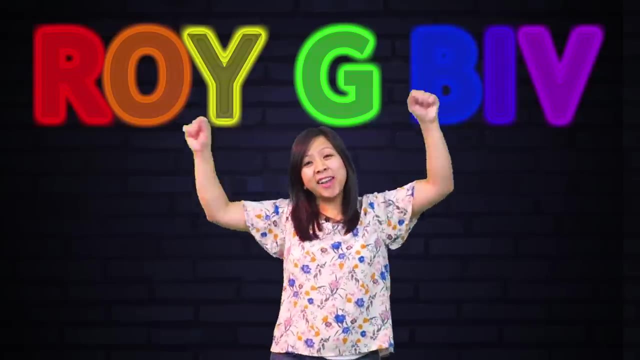 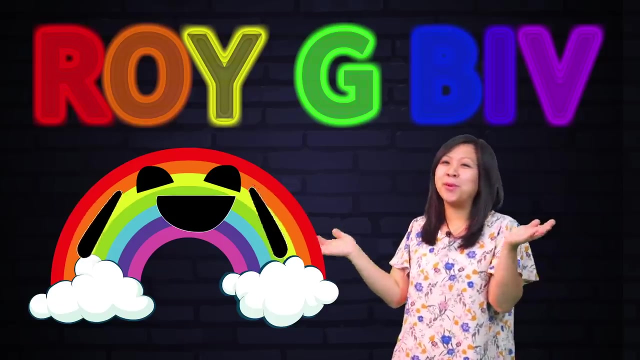 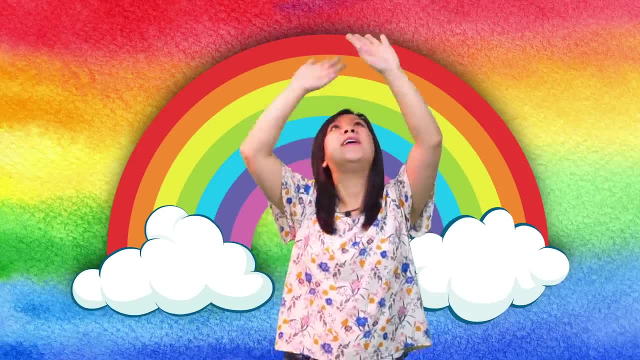 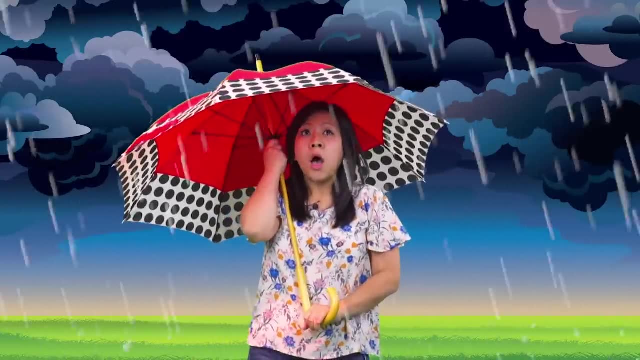 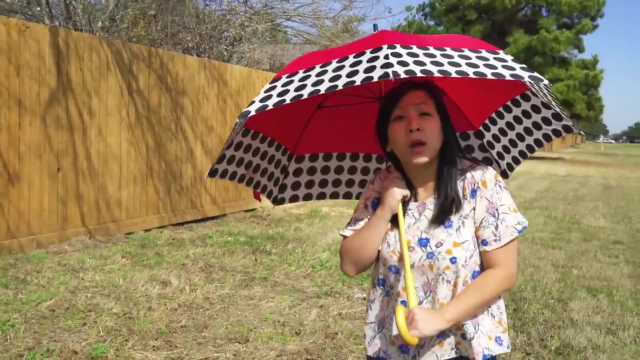 but why did the rainbow appear after the big storm? Oh no, I think a storm is coming. I better use my umbrella. Oh, I better run inside the house. I'll be right back. Is the storm over? Oh yeah, it is, yay. 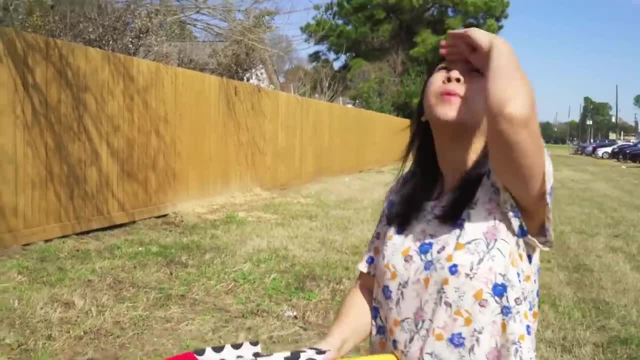 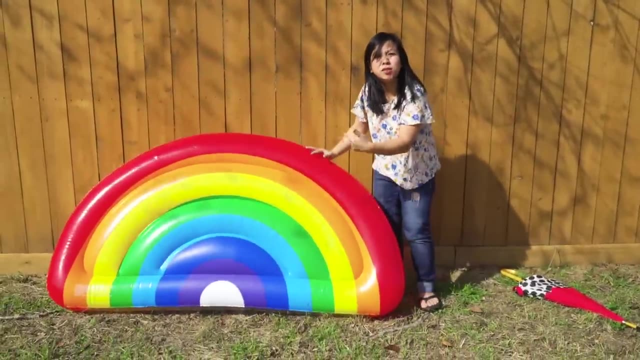 Now let's see if we can find that rainbow. Where is the rainbow? Ah, there it is rainbow. yay, look at this. Oh wait a minute, this is not a real rainbow, This is just a pool float. Let's test it out. 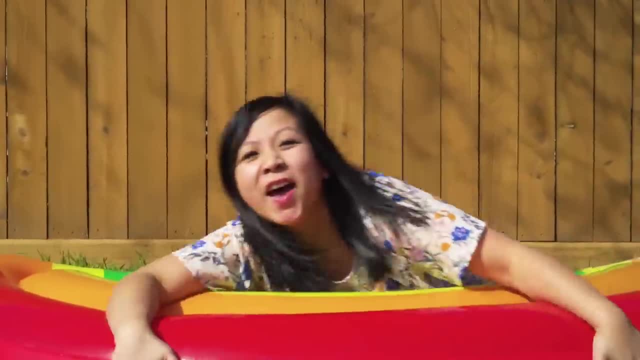 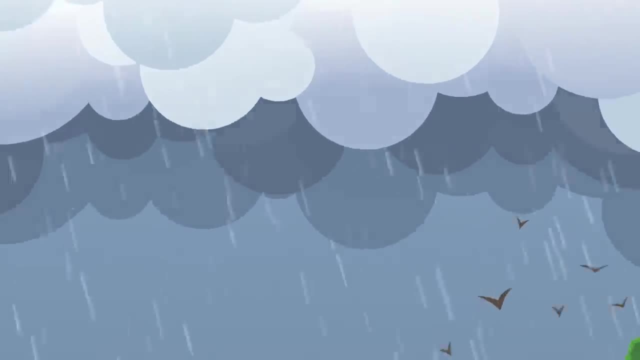 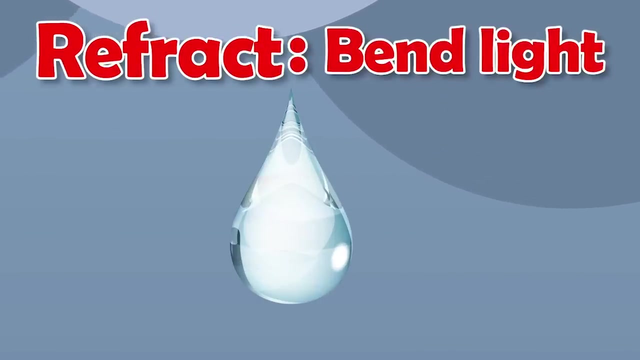 Whee, This will be so much fun in the pool. So when a storm comes and it rains really hard, it leaves water droplets in the sky. These droplets refract, which means bend. So when the sun shines, white light on, the water droplet. 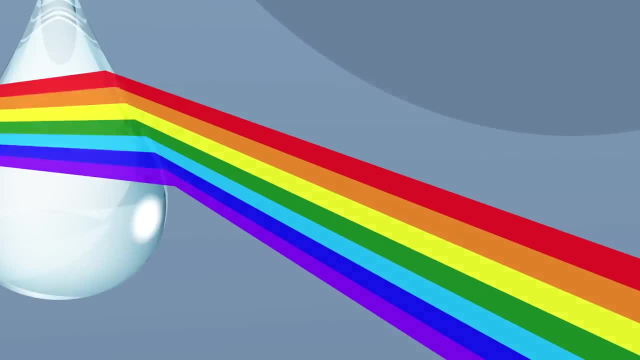 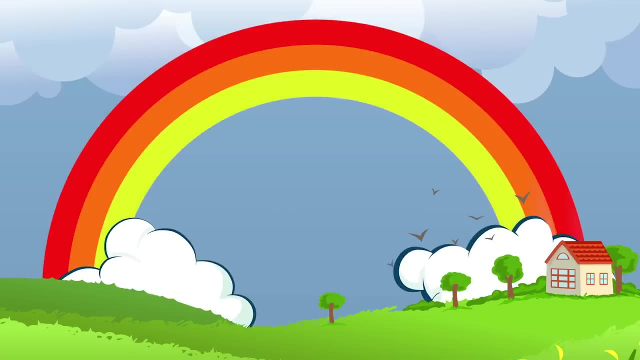 the light bends And we see all seven colors because they bend at different angles. Red is first, orange is second, yellow is third, green is fourth, blue is fifth, indigo is sixth and violet is seventh, Rory G fifth. 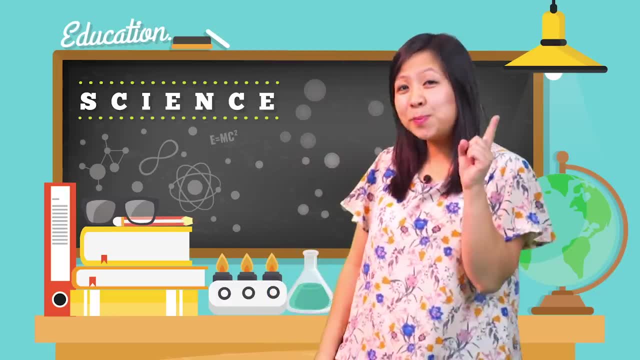 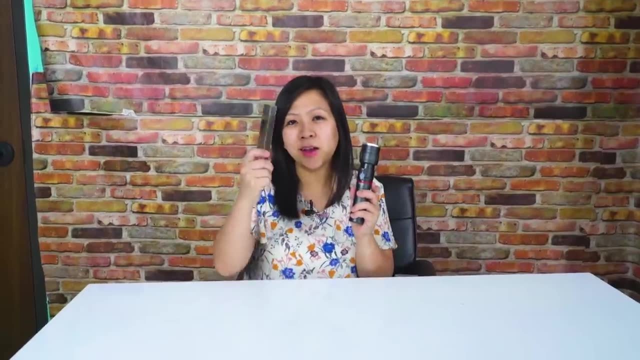 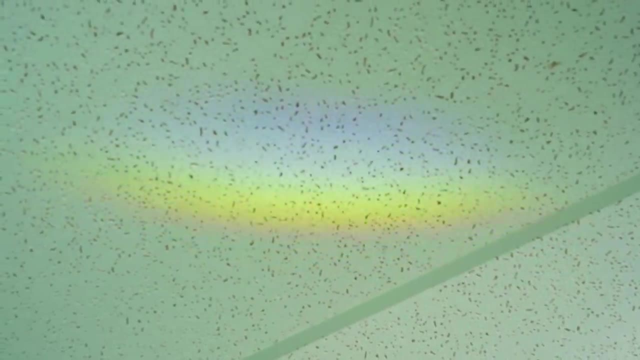 So seven colors total. Oh, the first person who discovered how a rainbow works was Sir Isaac Newton. He shines a white light on a prism like this. I'm gonna use a flashlight, Let's test it out. Do you guys see the rainbow right there? 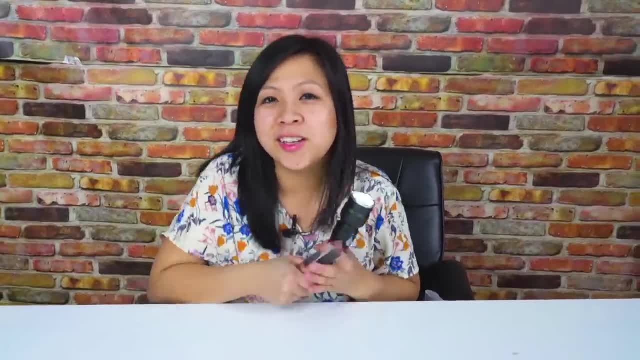 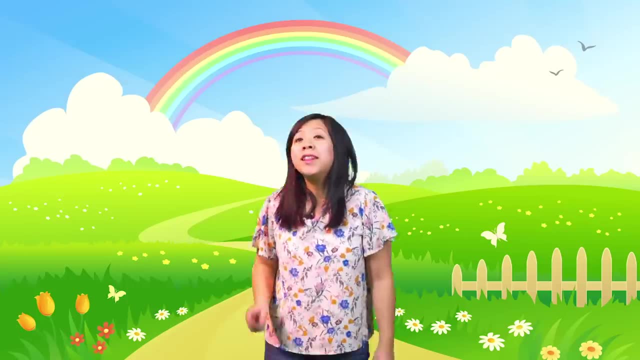 Isn't it neat. I also heard there is a pot of gold at the end of the rainbow. So let's go catch that rainbow. let's go Look, there's a rainbow over there. Let's see if we can find the treasure at the end of the rainbow. 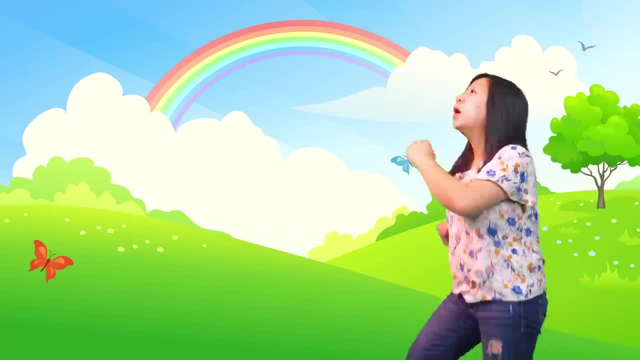 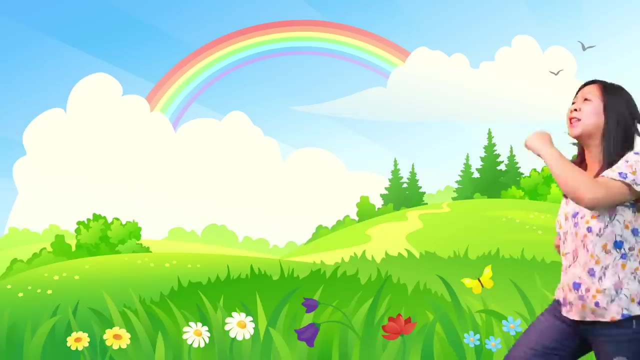 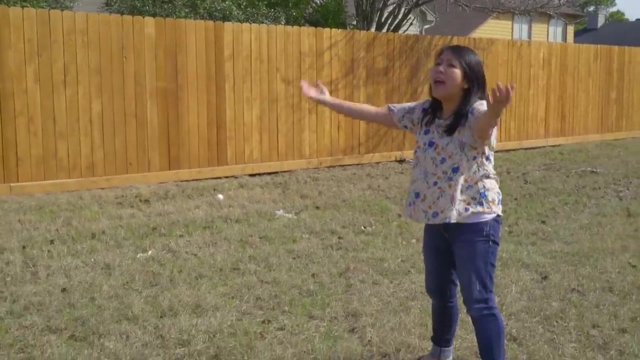 Hurry, let's go Now. we can do this. we can do this. Come on, Oh, are we getting any closer? you guys, are we? The rainbow is so far away I don't think I can ever reach the rainbow. 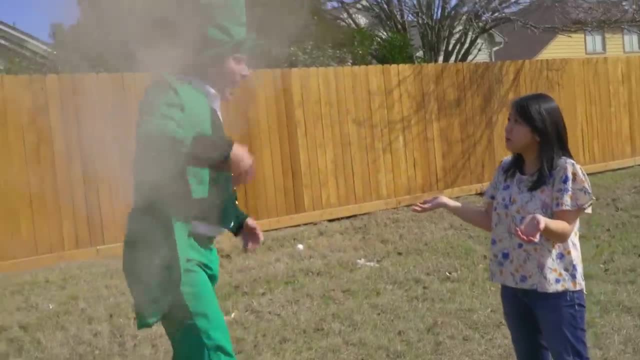 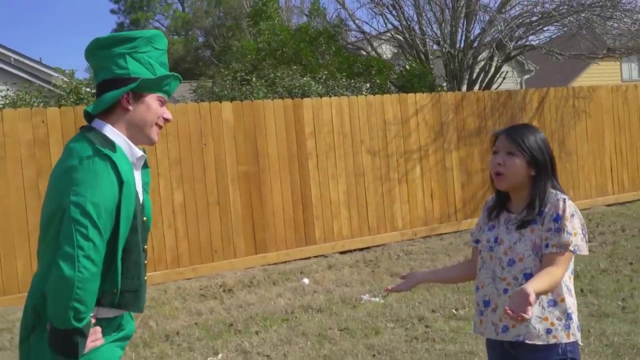 What should I do? Who are you? Hello, I'm a leprechaun. Are you trying to get a hold of me? pot of gold? I was trying was trying to get to the rainbow, but no matter how fast i run, i don't think i can ever get to. 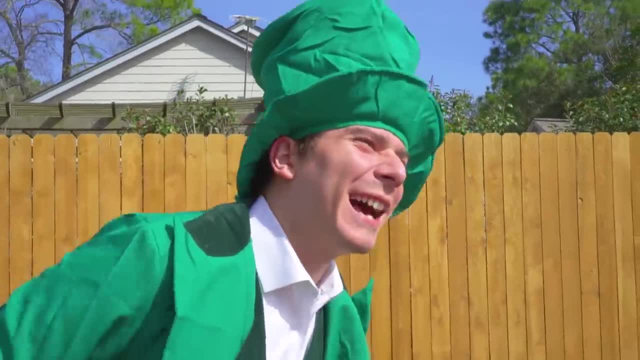 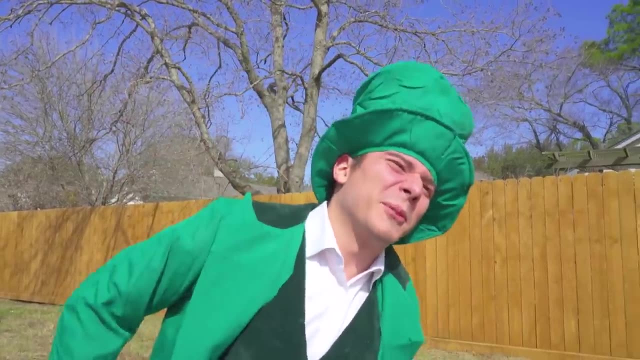 the rainbow. that's because the rainbow never really ends. as long as the water droplets are in the sky, the sunlight will make the colors appear at the same distance away from you. so if i keep running, i'll never get to the rainbow. no dearie, oh man. but then how do you know where? 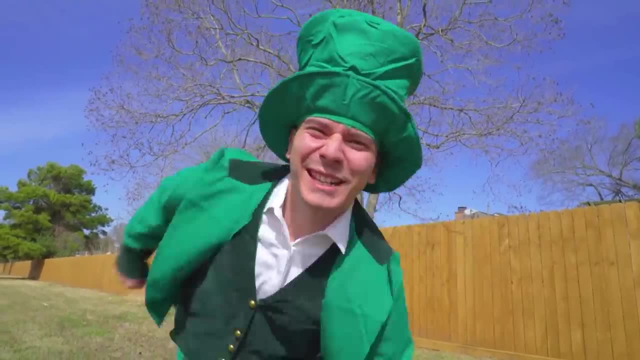 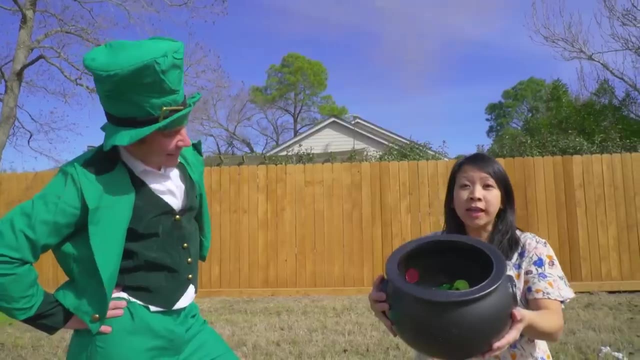 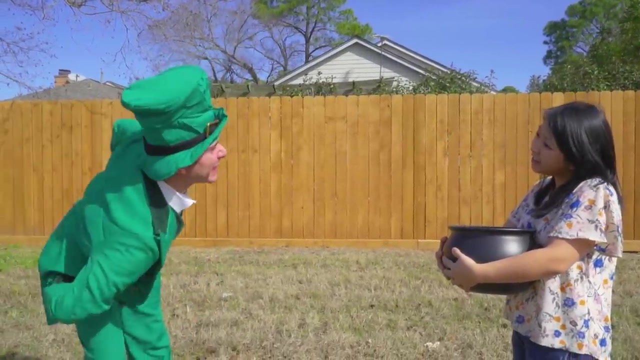 your pot of gold is. that's me little secret, but i can share some with you if you want. yes, please. wow, look at all the gold. thank you so much, mr leprechaun. you're welcome. don't spend it all at once. i will try my best, but these look so delicious, so thank you. 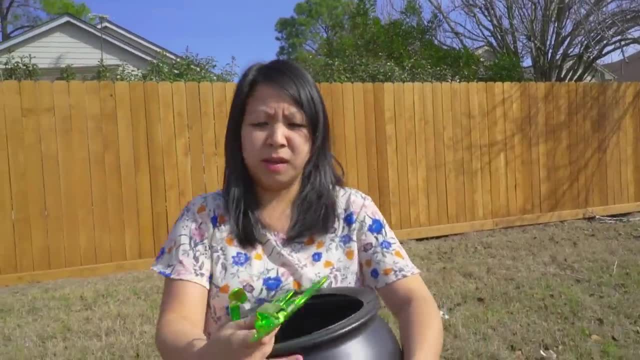 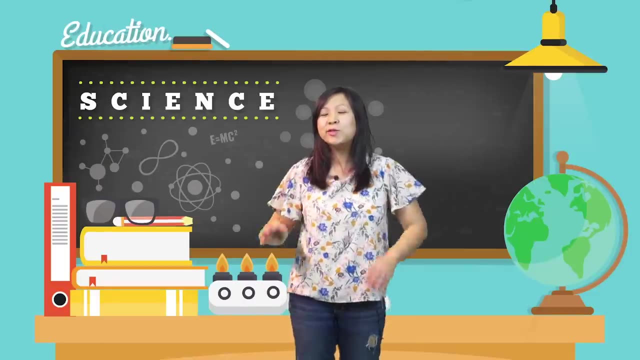 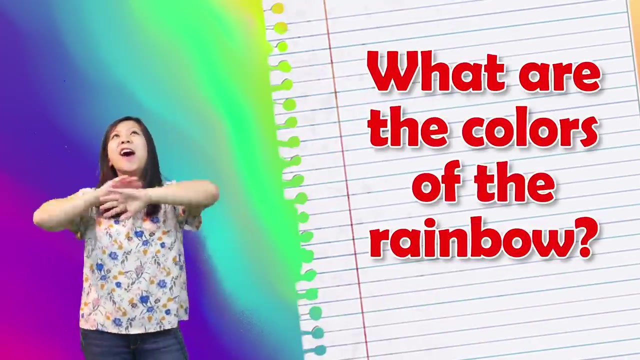 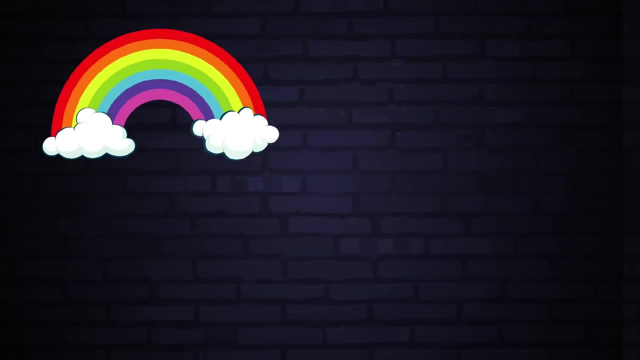 yay, what. what is this? oh, this is some awesome glasses. what'd you guys think? now that we know so much about rainbow, let's take a quiz. question number one: what are the colors of the rainbow? red, orange, yellow, green, blue, indigo, violet, or is it pink, green, gray, turquoise? 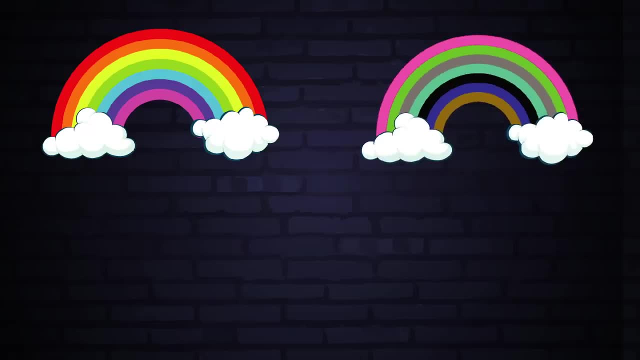 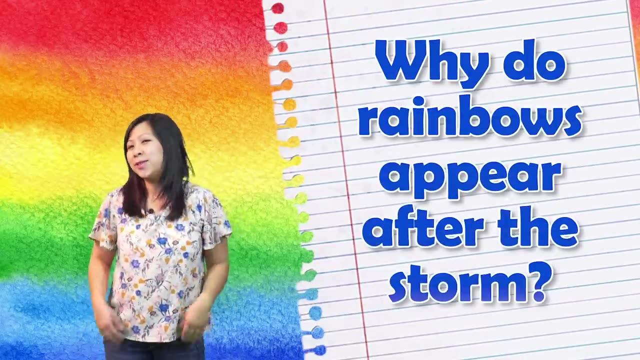 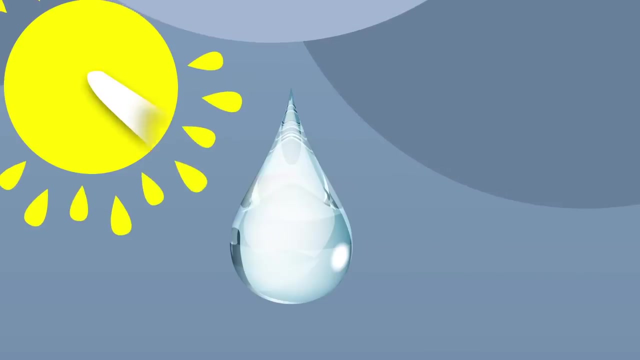 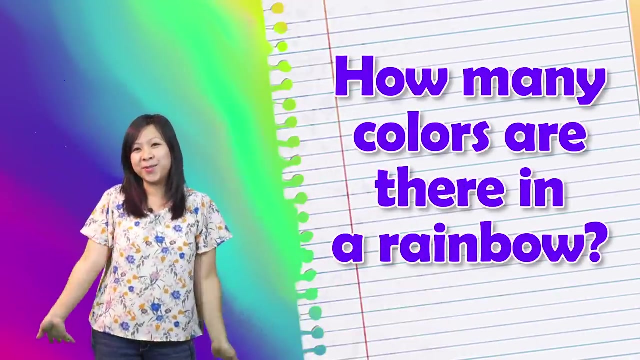 black, blue and tan, or is it white? question number two: why do rainbow appear after the storm? so leprechaun can hide their gold? sunlight shines on water droplets and they refract lights. or is it hot outside? question number three: how many colors are there in a rainbow? 50, 1 or 7? great job, i have so much fun learning about the rainbow. 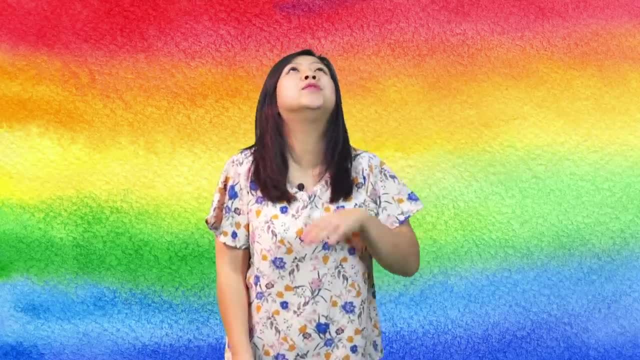 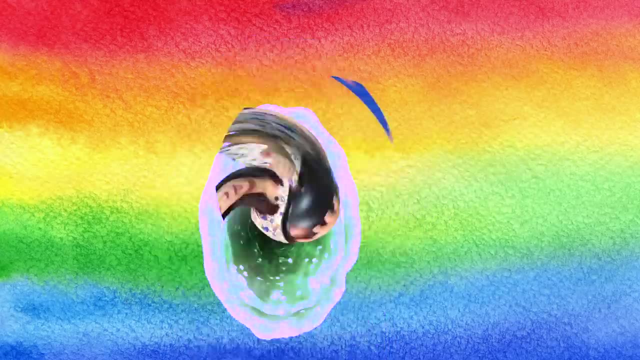 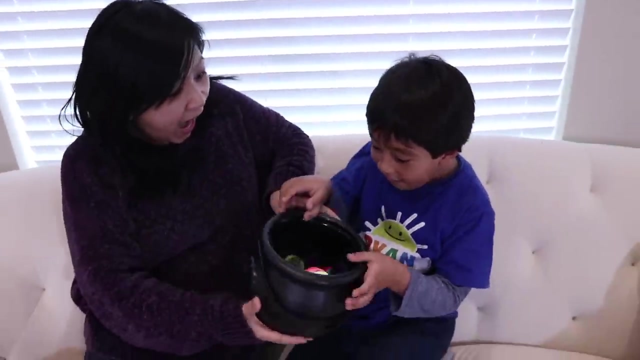 what do we know? what color is the rainbow? green and white? or what color is the rainbow in the sky- blue and white rainbows. with you Now, let's share this pot of treasure with Ryan. Let's go, And that's how a rainbow is formed, And look what I brought for you. What is that? 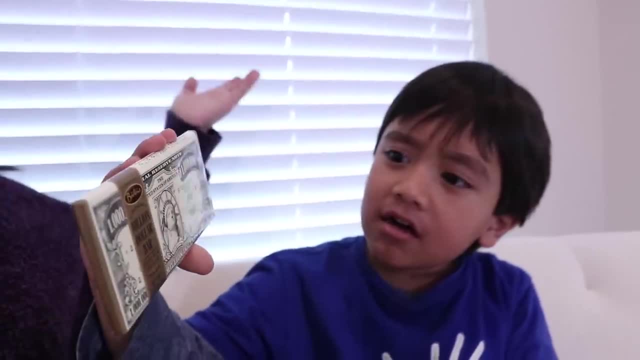 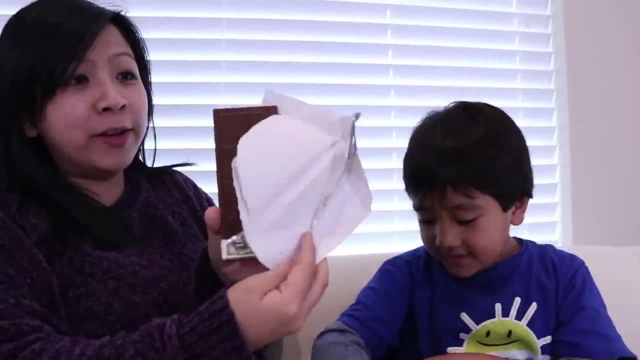 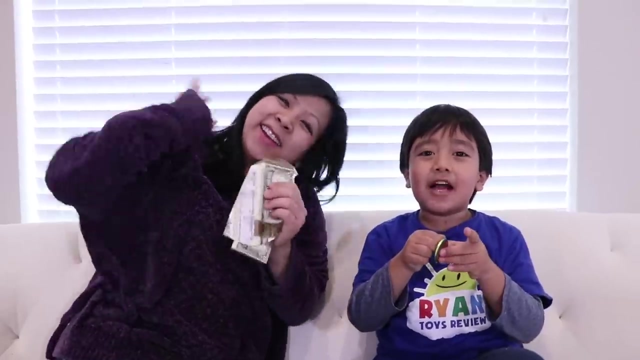 A one million dollar. What I didn't even know that was in there. Wow, Oh, they're just chocolate. Chocolate million dollars- Oh, wow, it's huge. Yes, Yeah, And chocolate coins- Wow, Thank you for watching our rainbow video. Bye, Well, I enjoy my chocolate. 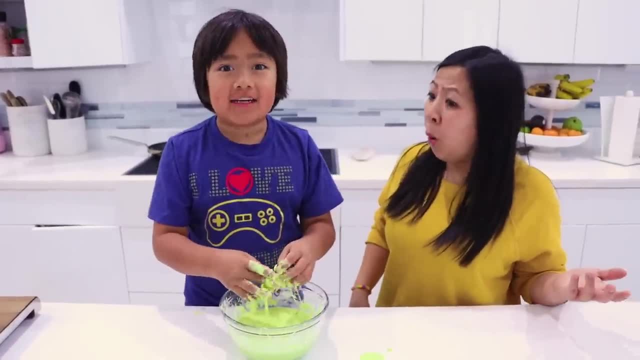 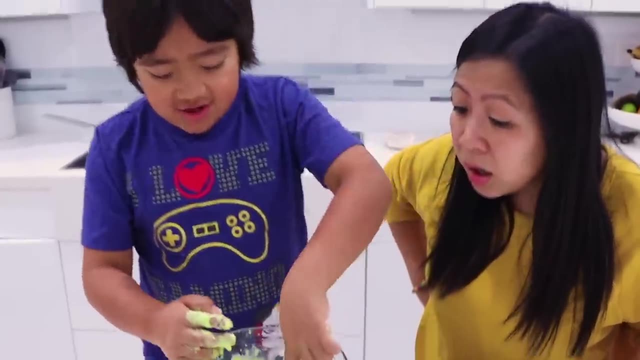 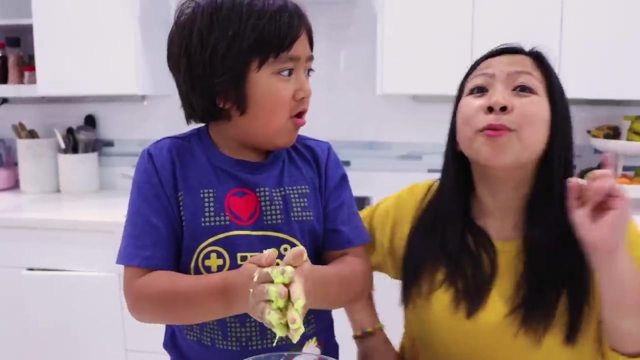 Ryan, what are you doing? Oh, I'm playing with oobleck. But, mommy, is oobleck a solid or a liquid? Why do you ask? Because it drips like a liquid, But when I punch it it acts like a solid. Ryan, oobleck is actually a liquid and a solid at the same time. 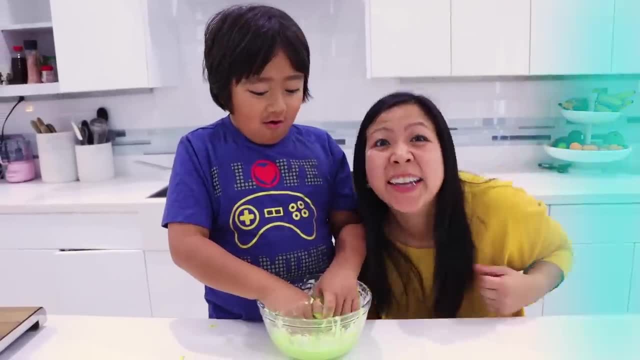 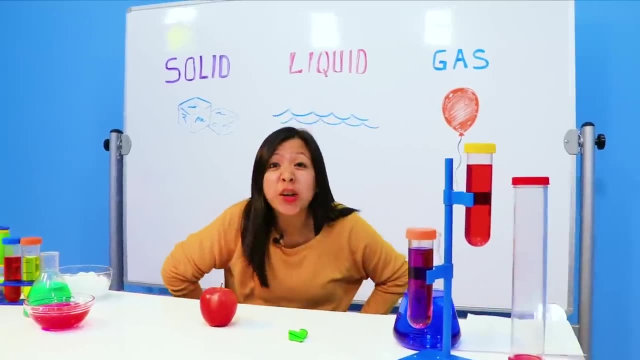 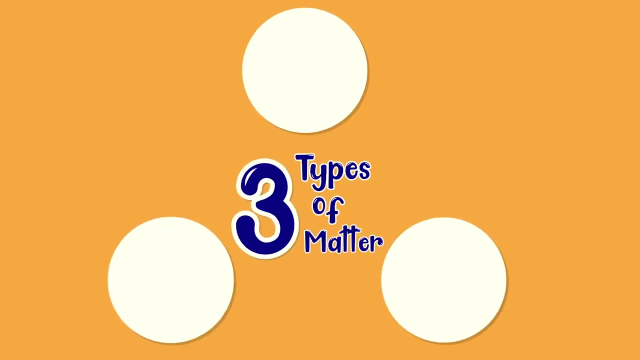 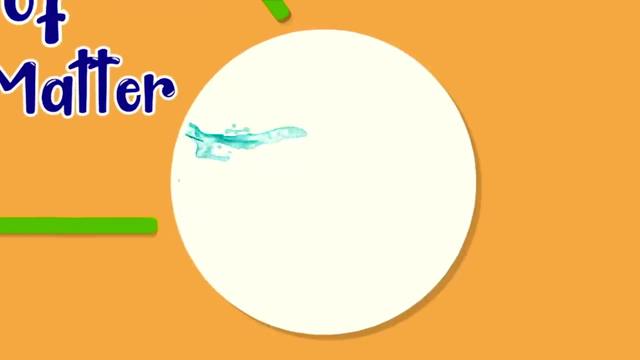 Whoa, Let me show you guys why. Mommy, Did you know that matter is anything with a mass and occupied space? So I'm a matter and you're a matter too. And there are three types of matter: Solid, like this ice, Oh, cold, cold. Liquid like this water color. 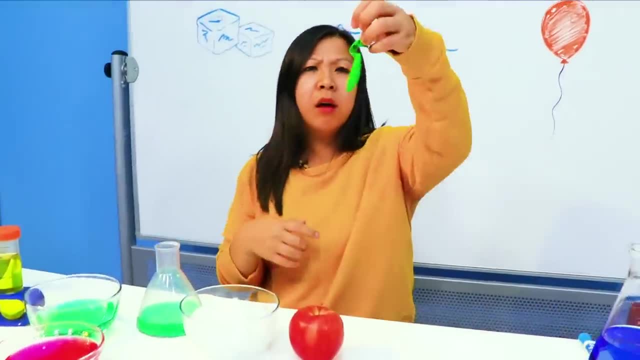 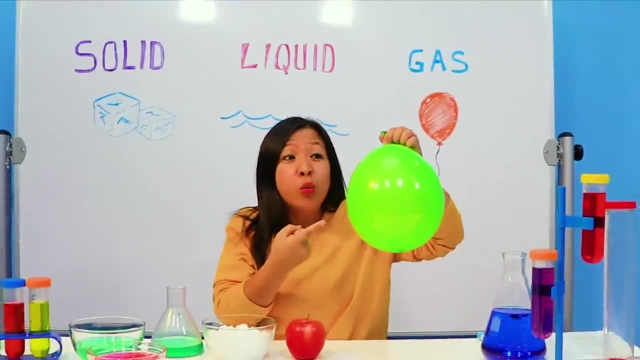 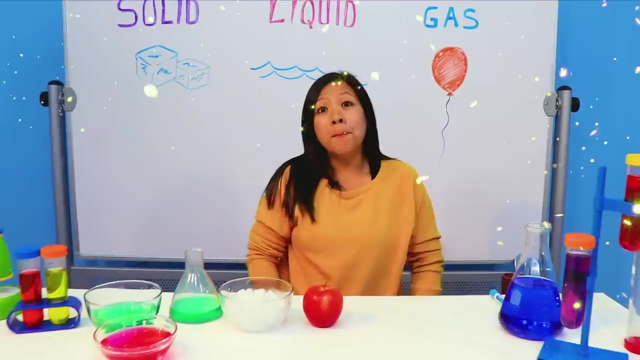 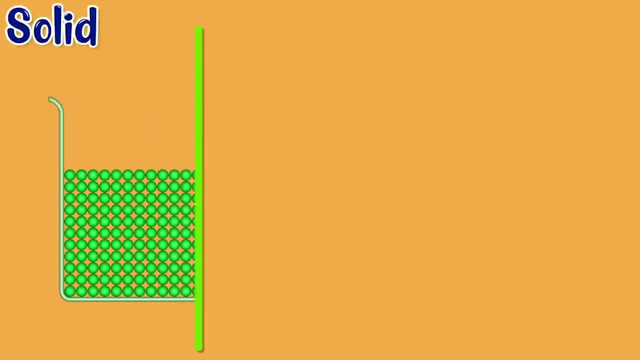 Or gas. Oh hold on, There we go. Now the balloon is full of air, which is gas, inside. Look. But why are there three states of matter? Well, it's because the particles in solid liquid and gas are all different. 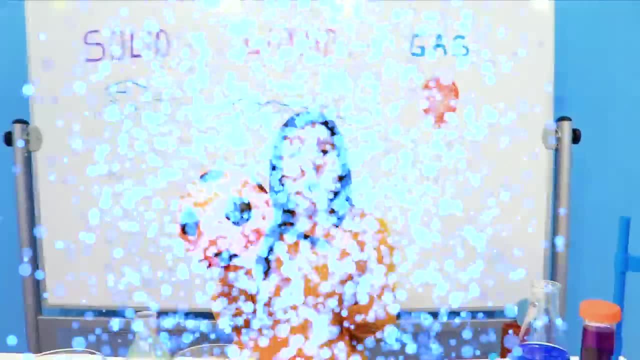 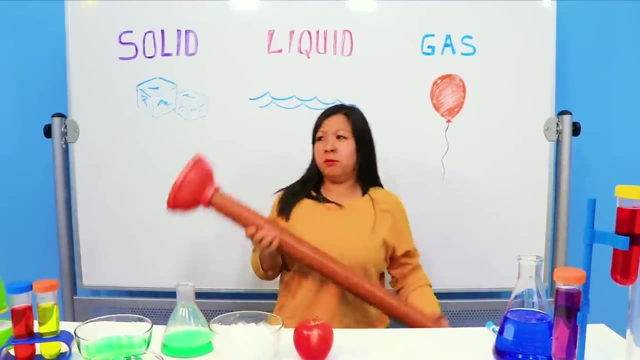 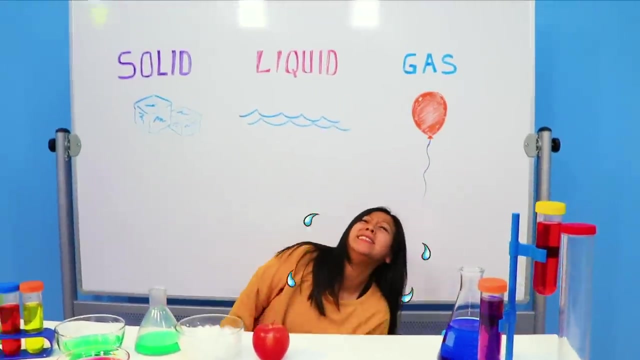 For example, solid like this ball has particles that keep its shape and volume. This is also a solid Right. Keeps its shape and volume. Okay, And this is also a solid Right. Keeps its shape and volume. This is also a solid. 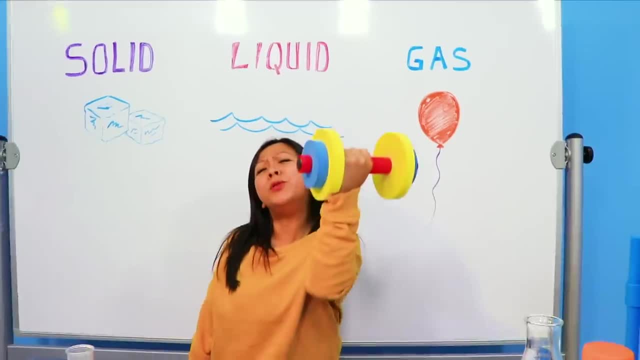 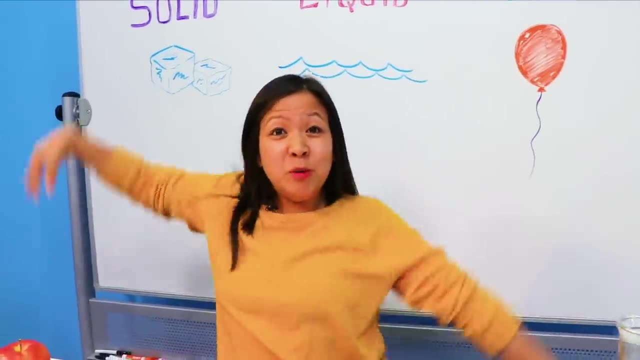 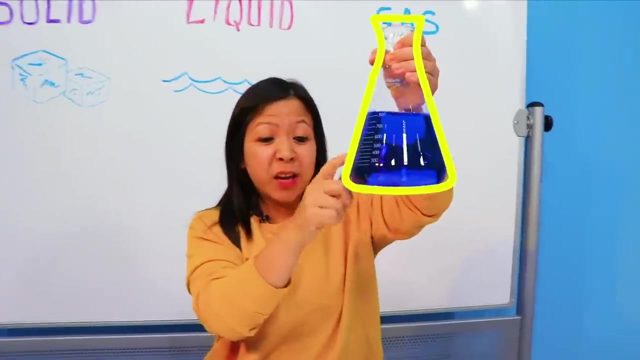 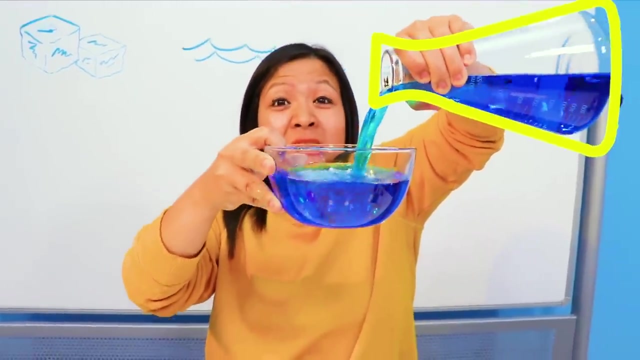 Keeping same shape and volume, I'm okay. Liquids, however, have particles that are free to move around. It keeps the same volume but different shape. For example, this liquid here. Look what happened. See, it keeps the shape of the container. 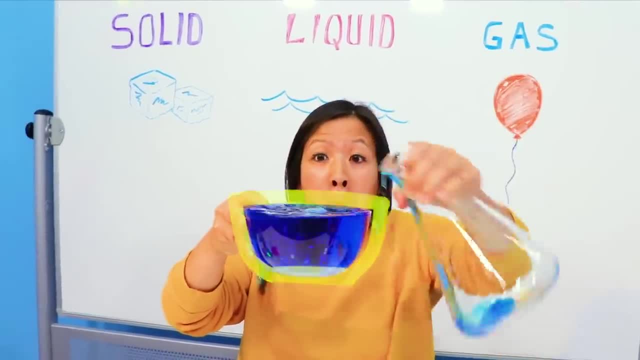 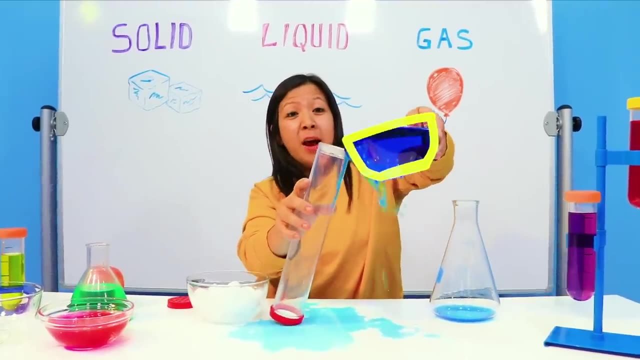 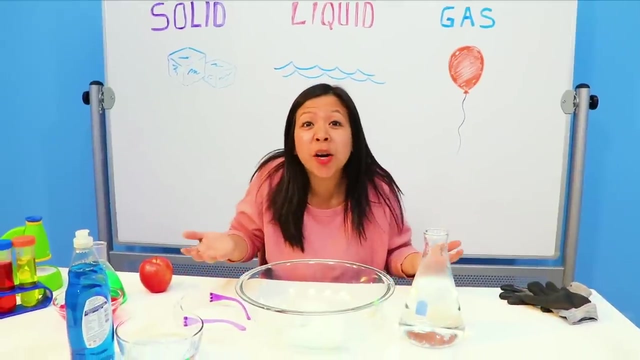 But it's the same amount of volume. Now let's put the liquid into a different shape container. This is the shape of a ball, And now this is the shape of this cylinder. Gas have particles that are so loose they have no definite shape or volume. 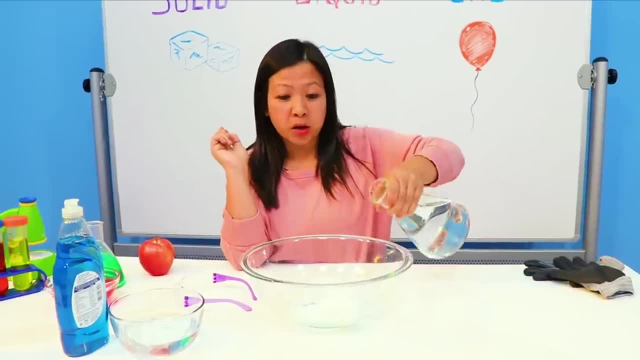 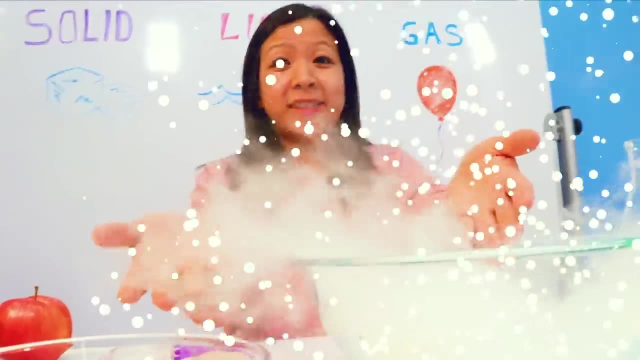 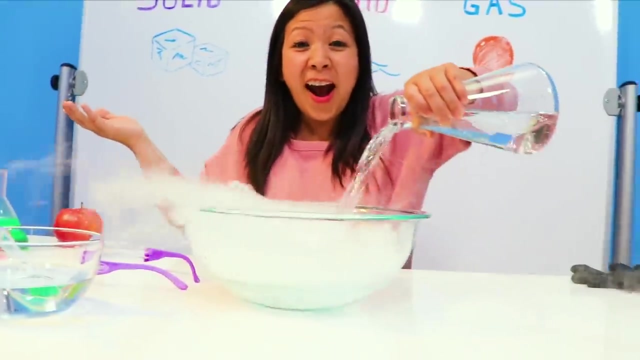 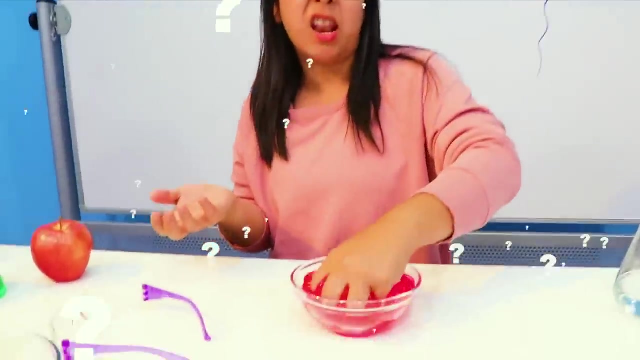 So this will have dry ice And I'm going to mix it in with water And look, it produces carbon dioxide gas. It just goes everywhere filling up the whole room. Whoa, Look at the gas flow. But what happens with things like slime? 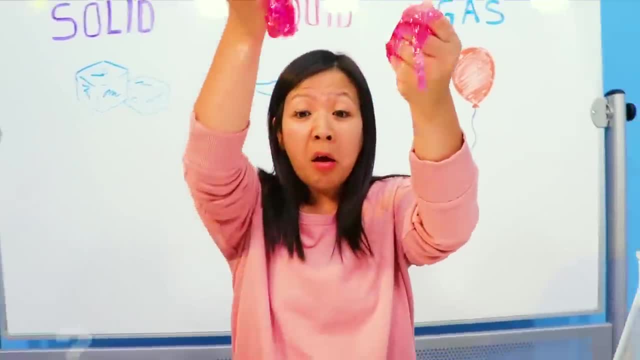 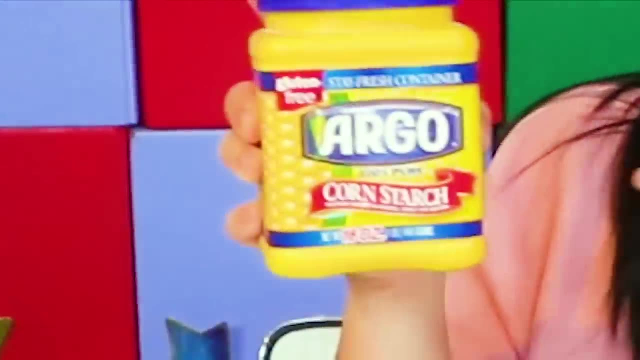 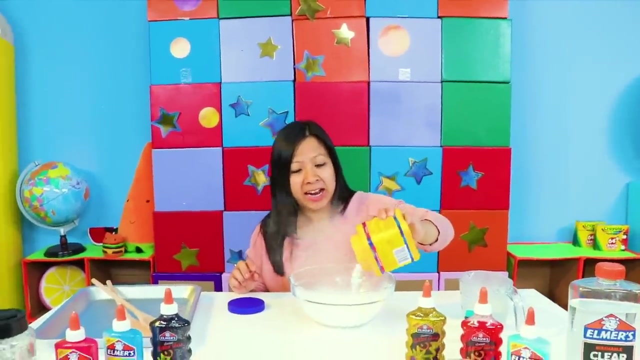 Is this a solid or is it a liquid? Before we explain what is slime, let's make our own special kind called oobleck. All you need is cornstarch, a spoon of coloring and water. Pour it inside a bowl. 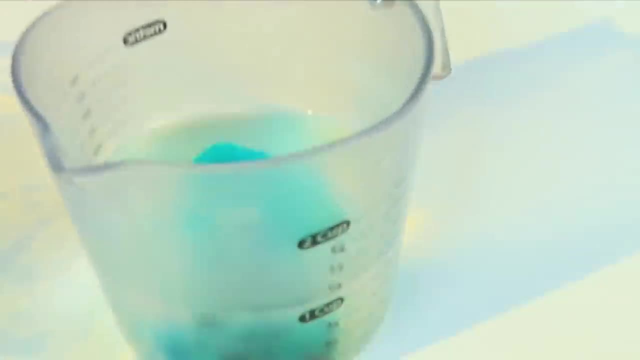 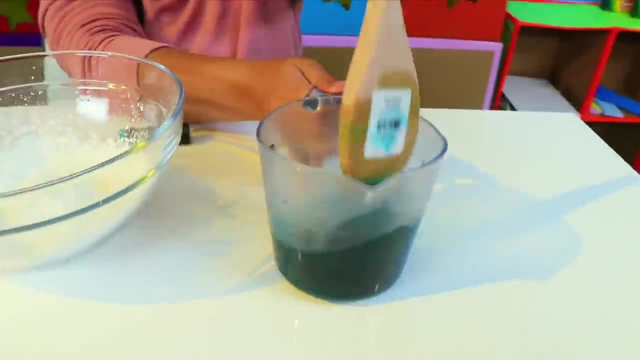 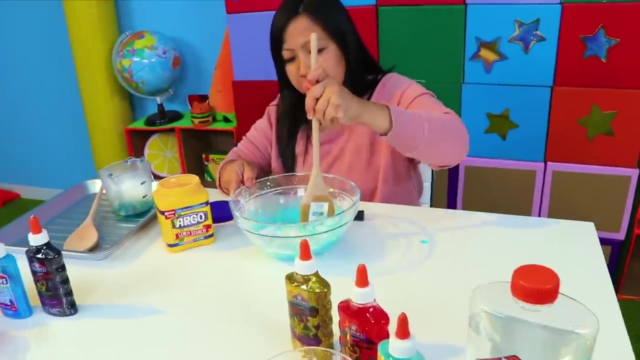 Let's make our water color green. Ooh, that's pretty. Get a spoon, agitate it, Then pour it into our cornstarch, Mix it up. Now this is really cool, Because look, if you pick it up. 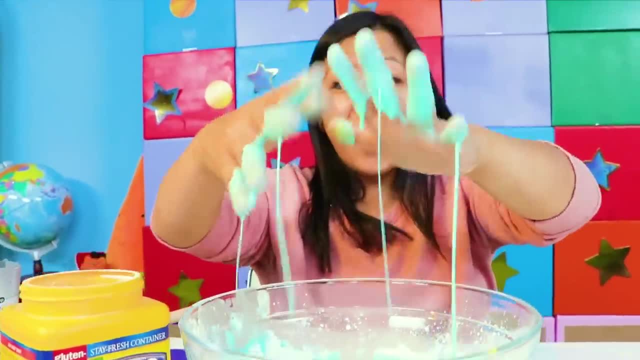 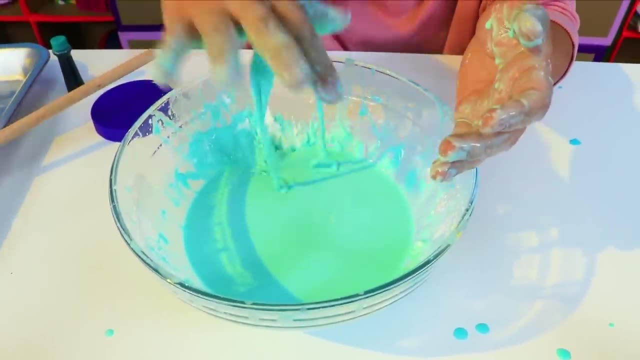 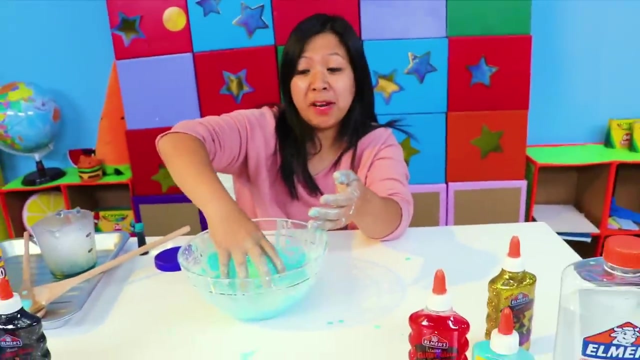 it looks like a liquid, See Liquid. But what happens if you tap it like this? Whoa, It was hard like cement, And again One, two, three, Wah. But if I do it slowly it's a liquid. 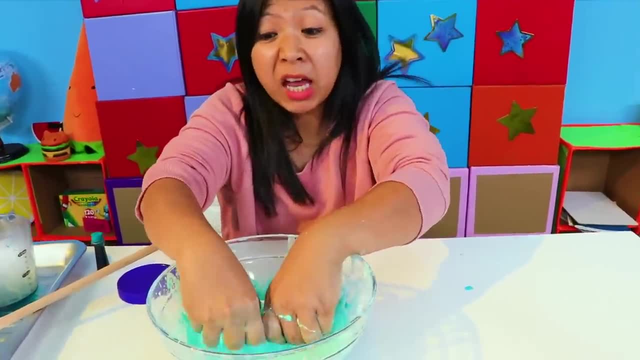 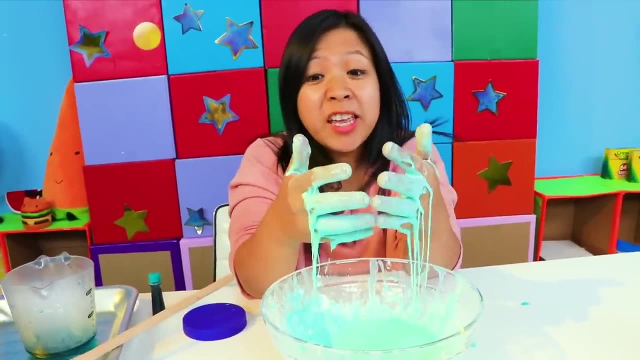 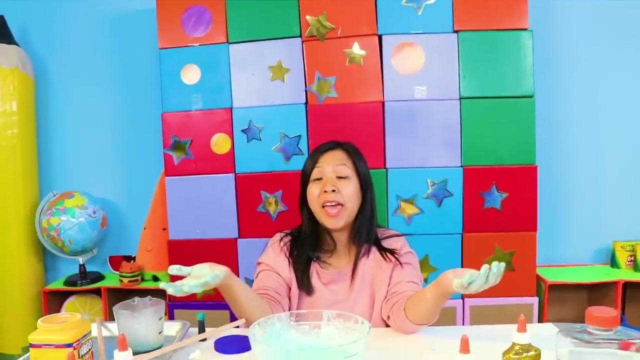 What's going on So is slime like oobleck. Is this a solid or a liquid? Well, this is a special kind. It's called non-newtonium liquid. But what is a non-newtonium liquid? Well, it can behave as a solid. 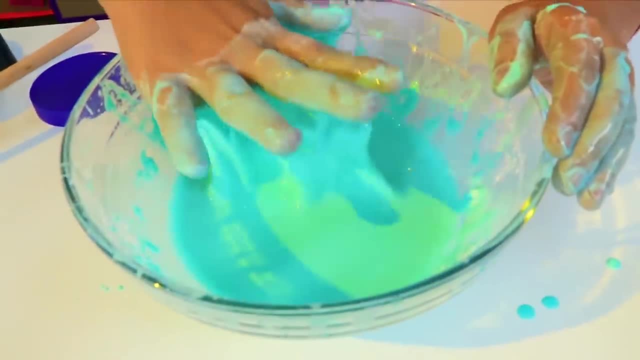 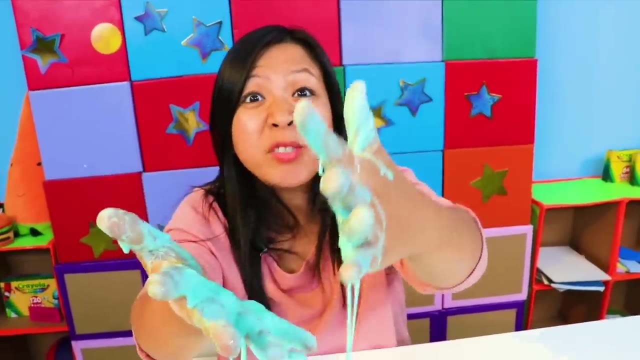 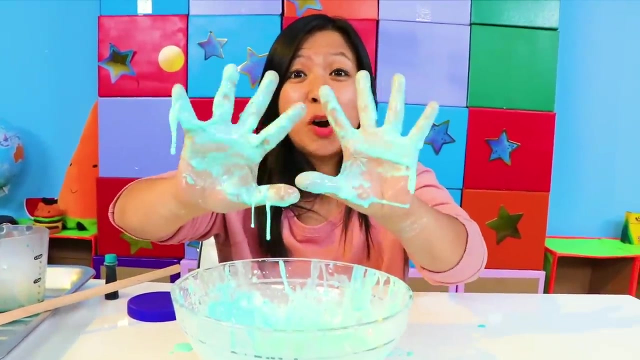 when pressure is applied, like this. Or it could behave like a liquid when pressure is not applied. Pretty cool stuff, huh, I have an idea. Why don't we mix it up and add glitter and other things to our oobleck Wah? 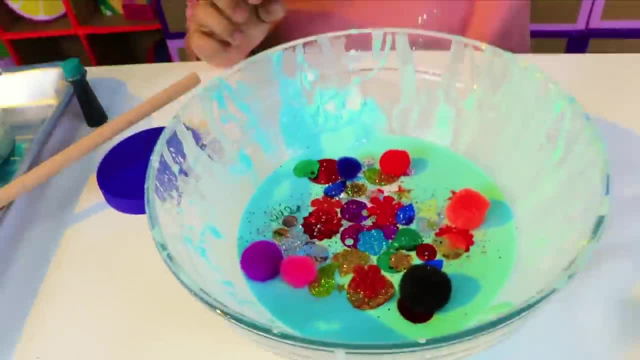 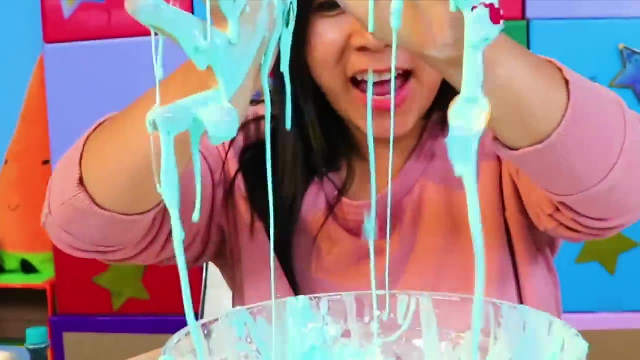 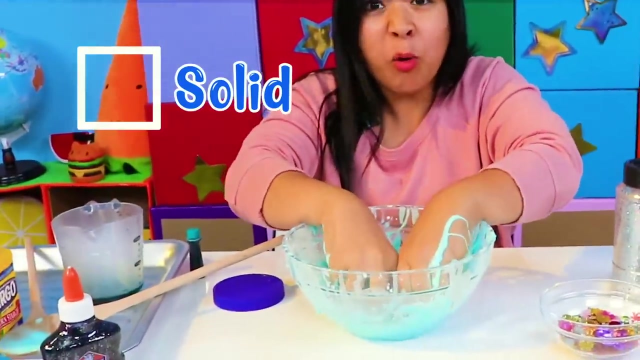 Some pom-poms And some glitter There, Let's mix it up. Whoa, look how cool this looks. Wow, There it is Your own non-newtonium liquid. Is it a solid Or is it a liquid? 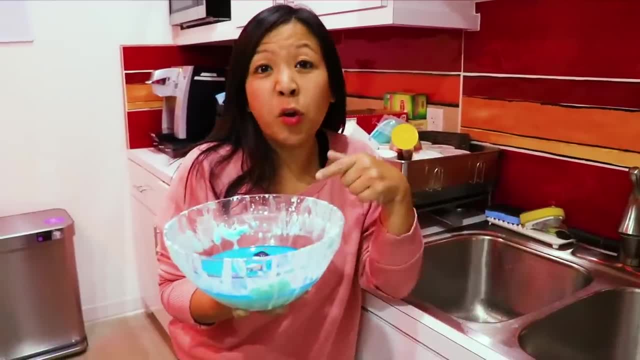 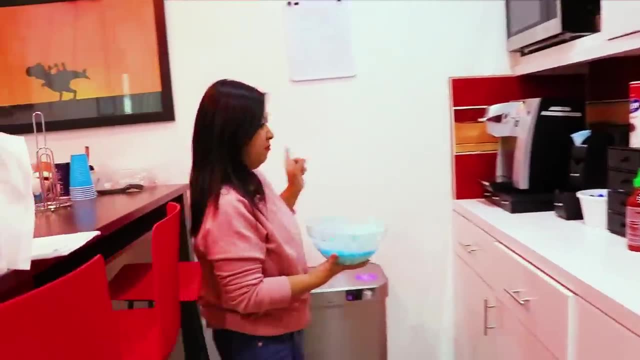 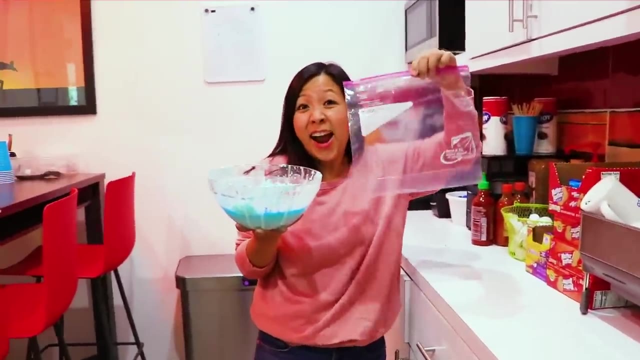 Both. When you're done playing with your oobleck, do not pour it down the sink or else it might clog the sink. You can either pour it in the trash or you can save it in a Ziploc bag so you can play with it for later. 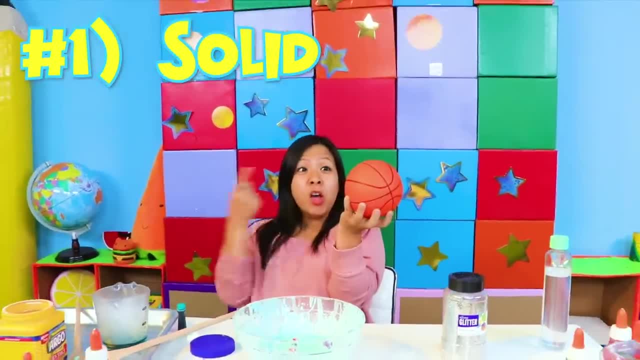 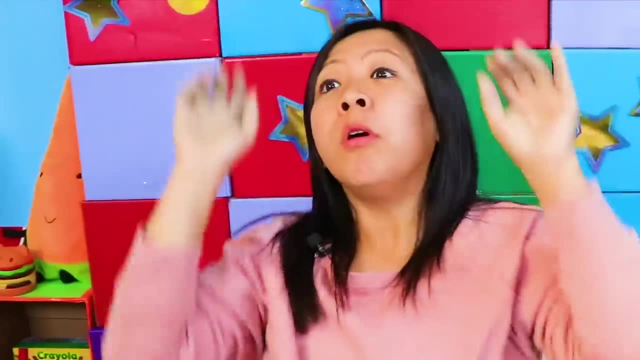 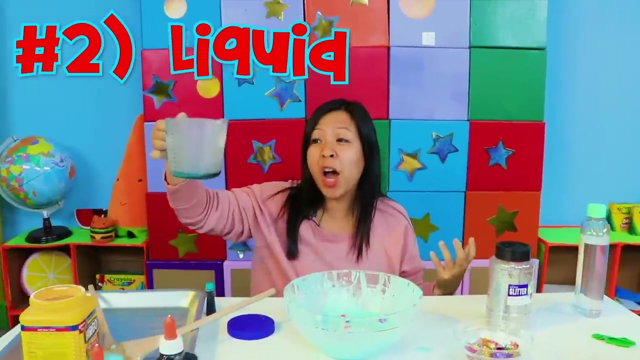 So, to recap, the three states of matter are solid, which has a definite volume and a definite shape, like this ball is a circle, Oh sorry, Gus. Second is a liquid, like this water here A definite volume but not a definite shape. 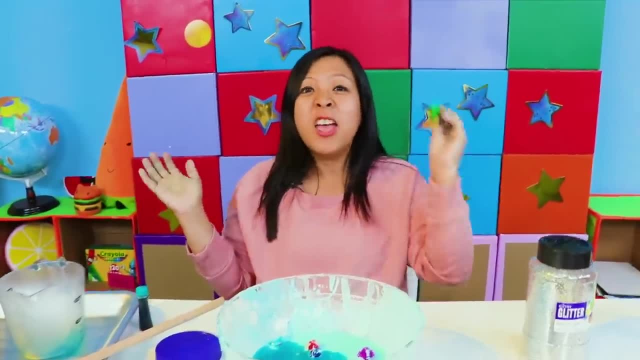 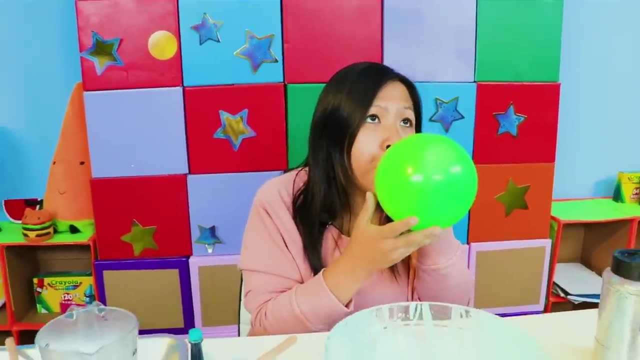 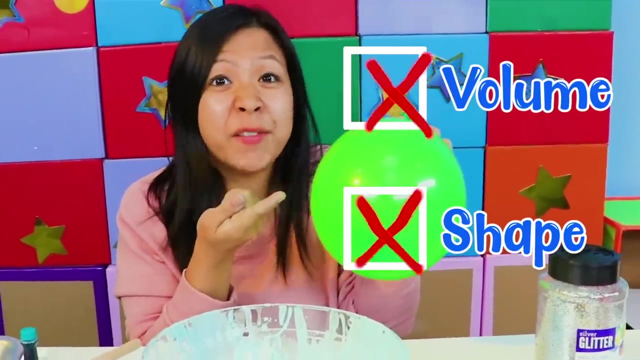 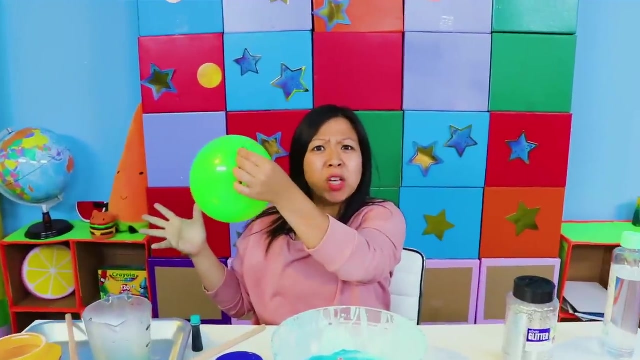 And the third type of matter is a gas. The gas in this balloon does not have a definite volume and does not have a definite shape. The gas that was in my mouth now is inside this balloon. Let the gas in the balloon go, And now the gas will spread. 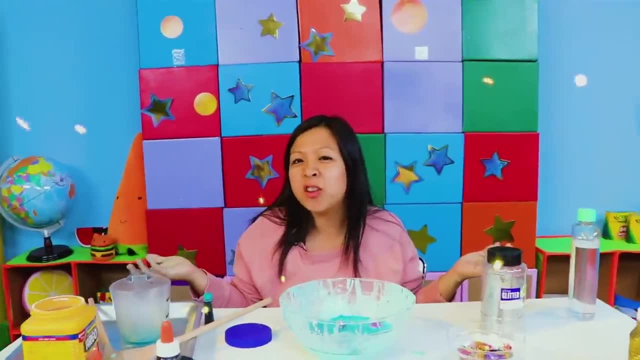 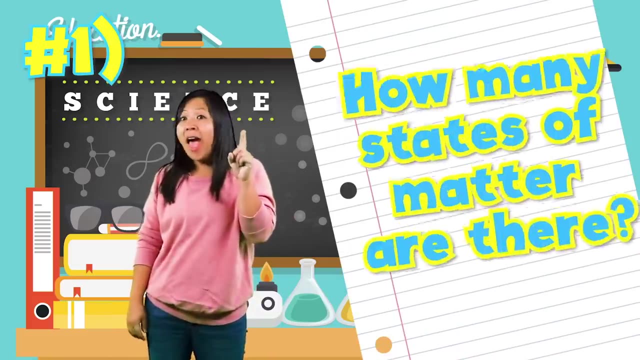 and take the shape of a room. So now that we've learned all about solid liquid and gas, how about we take a test? Question number one: How many states of matter are there? Is it A one state of matter? 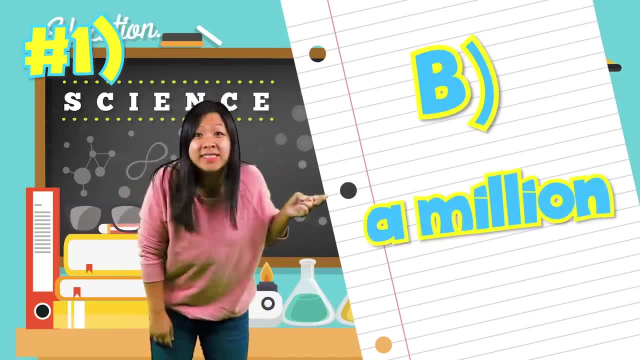 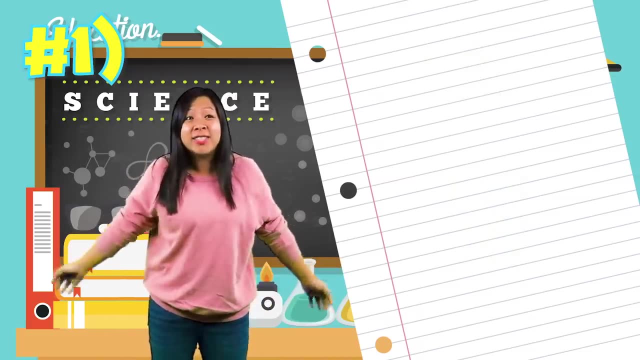 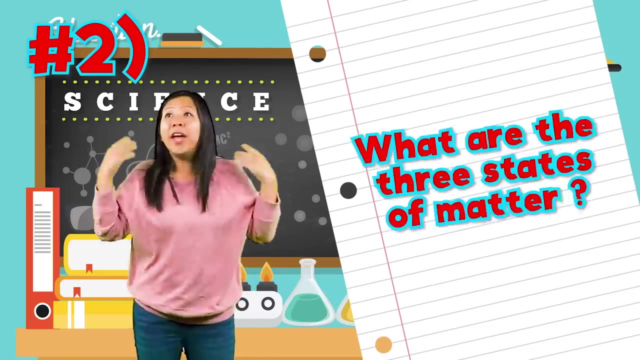 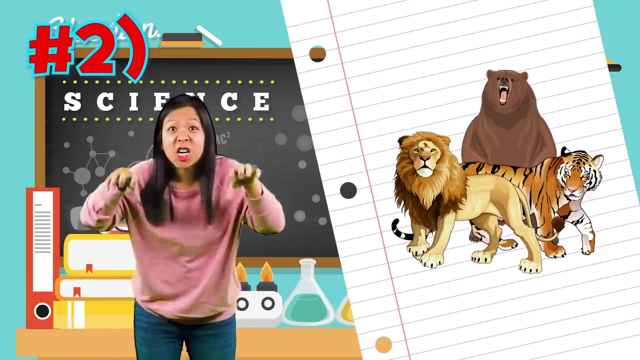 Or is it B- a million states of matter? Or is it C? three states of matter? That's right. The answer is C. There are three states of matter. Question number two: What are the three states of matter? Is it A? lions, bears and tigers? 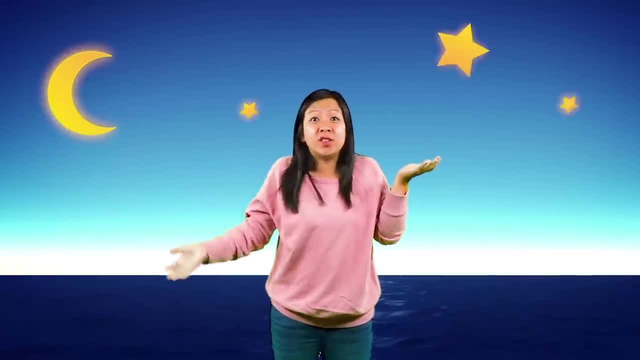 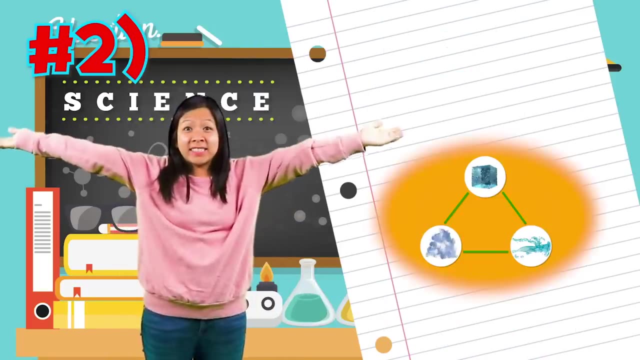 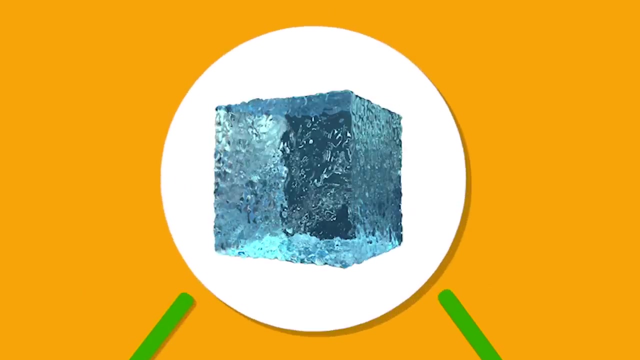 Or is it B- sun, moon and stars- Or is it C- solid, liquid and gas? Well, that's right, It is C. The three states of matter are solid, liquid and gas. Question number three: 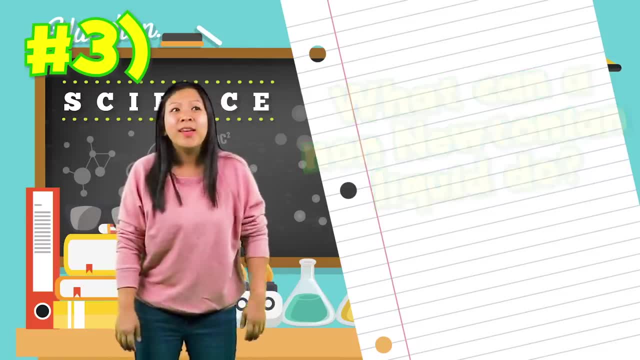 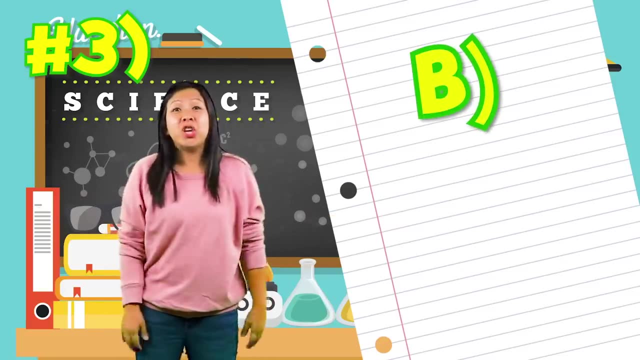 What can a non-Newtonian liquid do? Is it A, it can change color, Or is it B- it can change its viscosity if a strong force is applied. Or is it C- it can sing? Did you guys guess the answer? 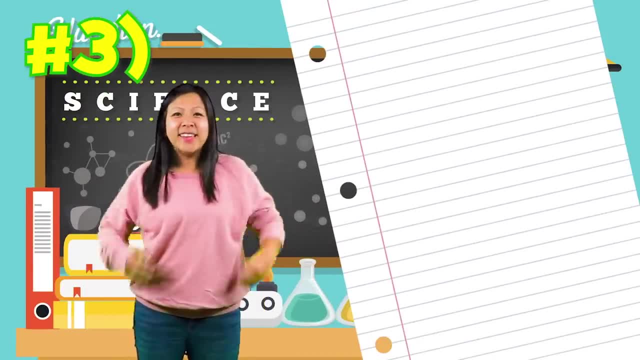 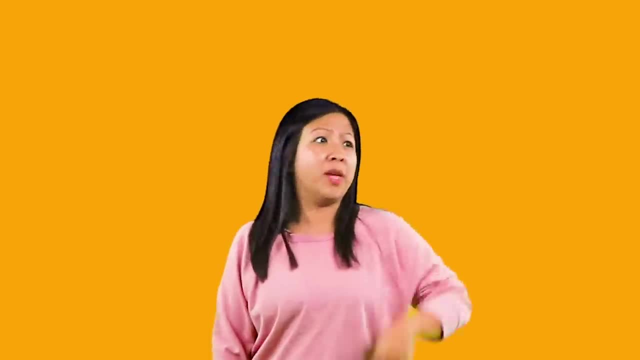 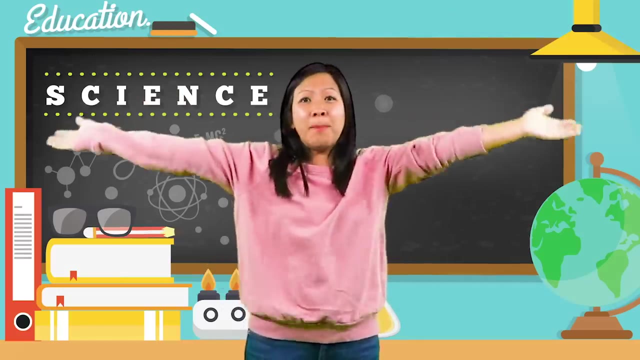 That's right. A non-Newtonian liquid is C. It can change its viscosity if a force is applied. So sometime it could be a liquid or sometime it could be a solid. So now that we learned so much about solid liquid and gas, 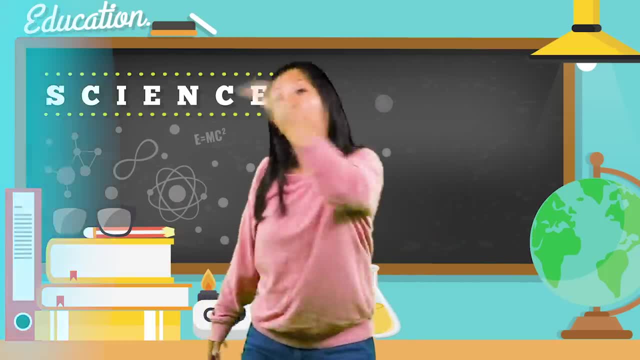 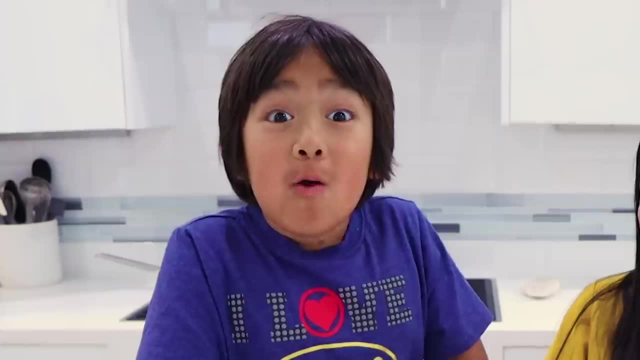 let's go back and tell Ryan Let's go. So there it is. That's why oobleck is a liquid and a solid at the same time. Wow, that's so cool. I didn't know it could be a liquid and a solid. 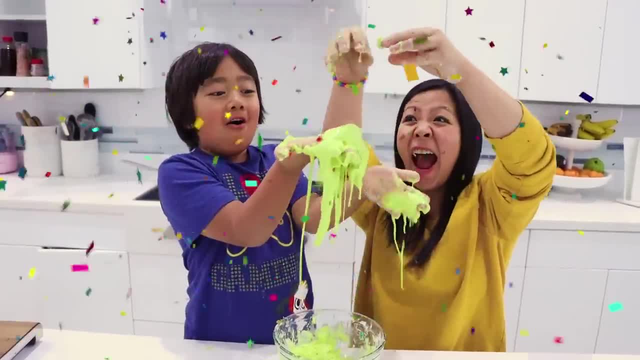 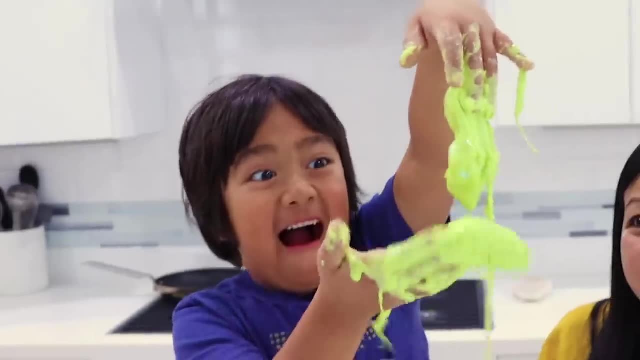 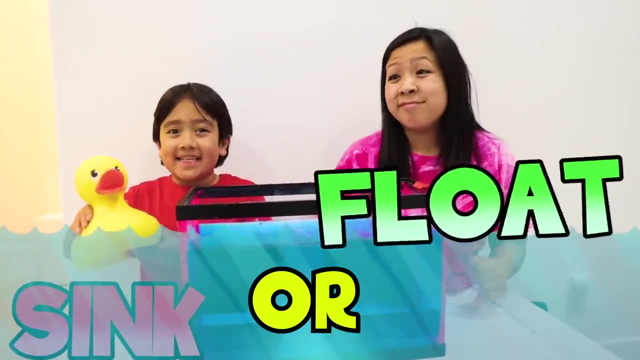 Non-Newtonian. Whoa Bye, Thank you for watching. Remember always: stay happy and rise up. Bye, Bye. Hey guys, do you think this rubber ducky is going to sink or float? I think it's going to float. 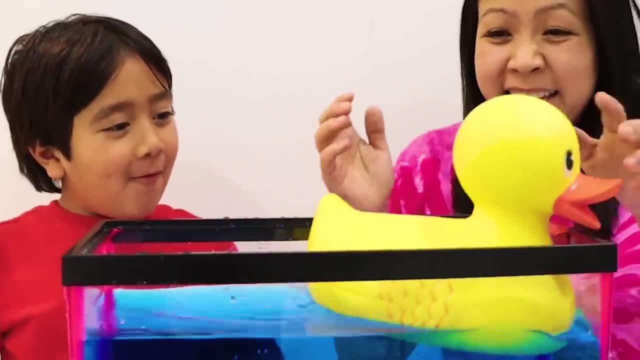 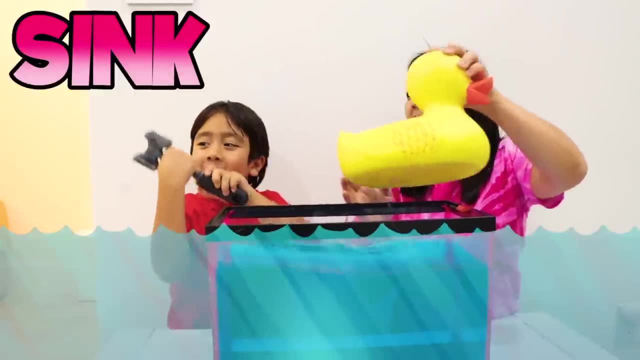 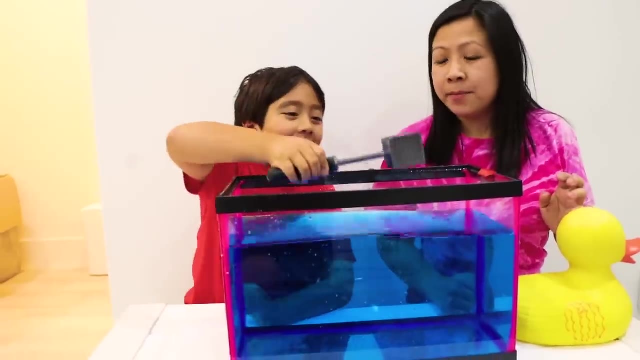 Whoa, it's floating. Whee, Good job, Ryan. Now what about this mallet? Do you think it's going to sink or float? I think it's going to sink. Let's see It's sink, Good job. 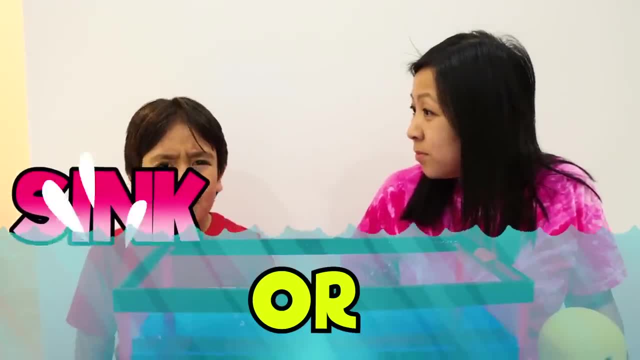 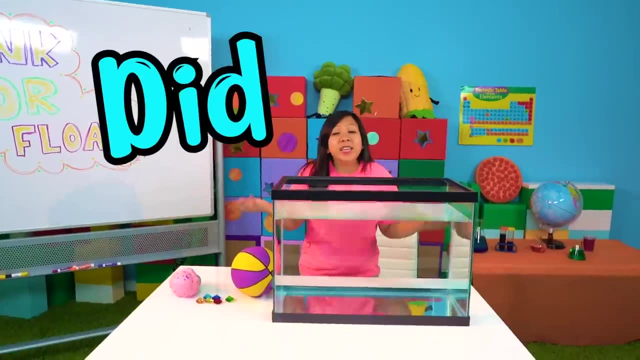 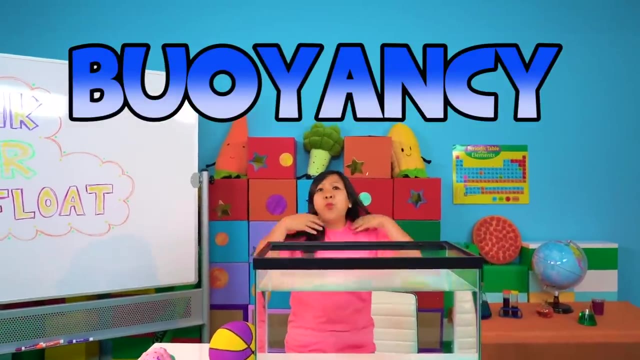 But, mommy, why do you think sink or float? Good question, Ryan, I'll show you. Come on, guys, Where'd mommy go? Did you know an object's ability to sink or float is called buoyancy? But why does an object sink or float? 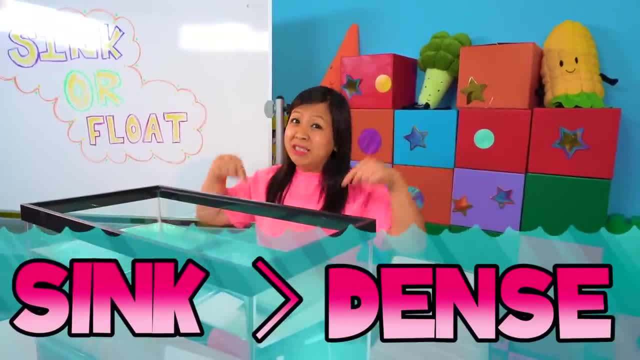 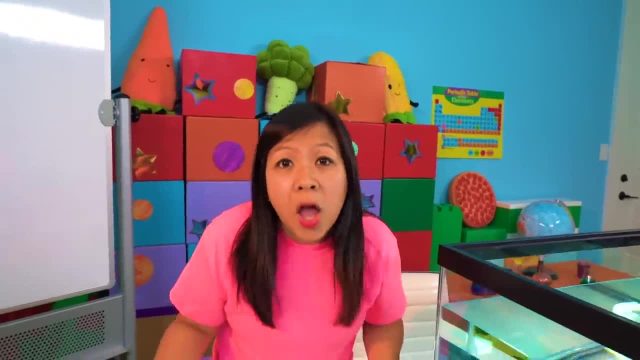 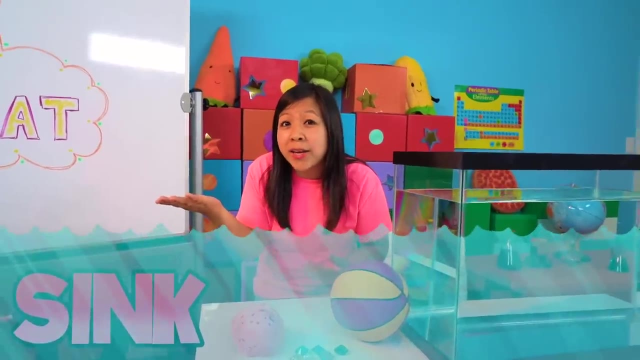 Object will sink if they're more dense than water. An object will float if they're less dense than water. So let's try putting these objects in water to see which one will sink and which one will float. Let's see what we have here. 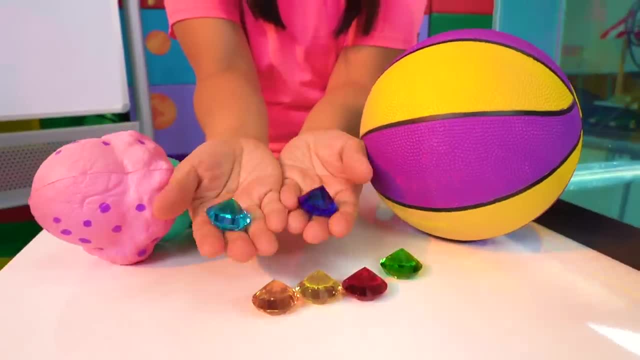 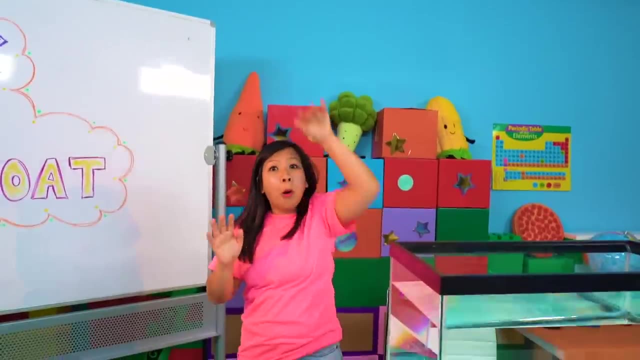 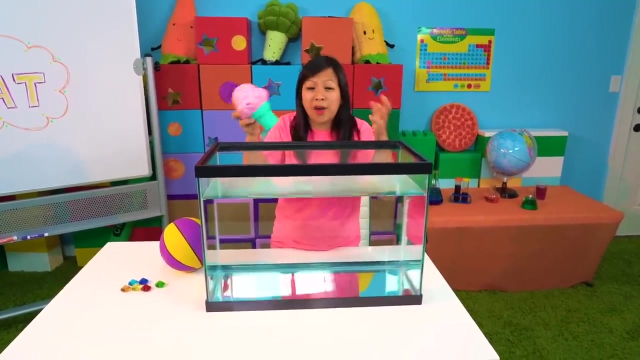 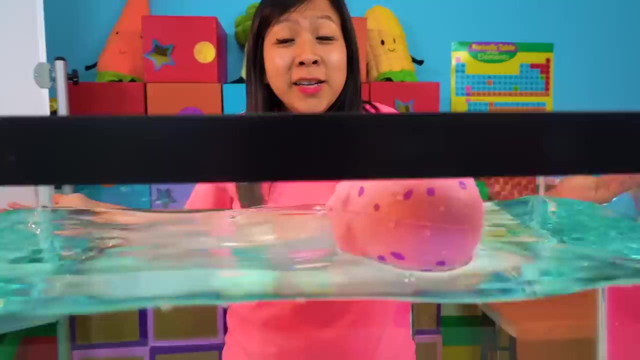 Squishy Some diamond jewels And a basketball. Get that back. Come back The squishy toys. feels light, but let's see if they'll float in water. All right, One, two, three, Wow, The squishy toy float in water. 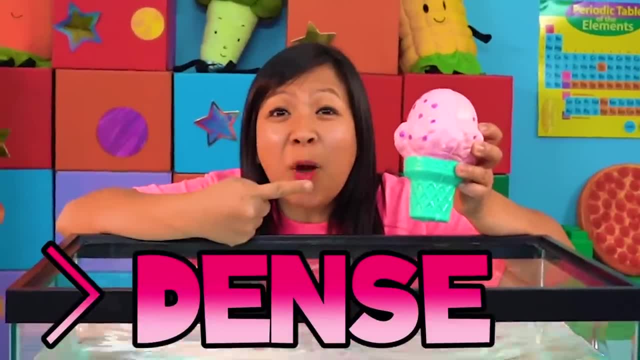 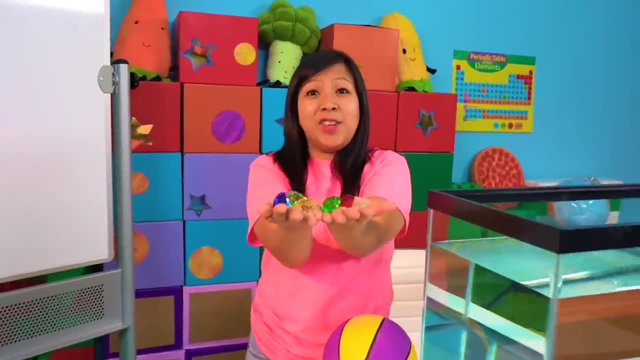 So what does that mean? It's less dense than water, Yay, Woohoo, Okay, Let's see what we have next. Next we have these stones: So colorful, Woohoo, Ah, so bright. They're smaller than the squishy toys. 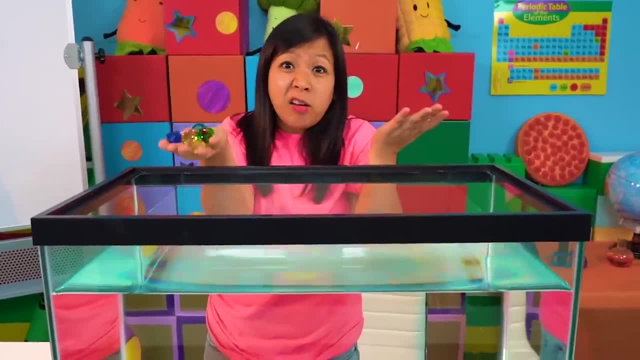 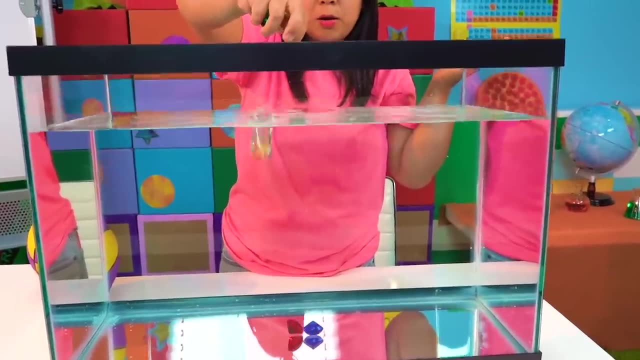 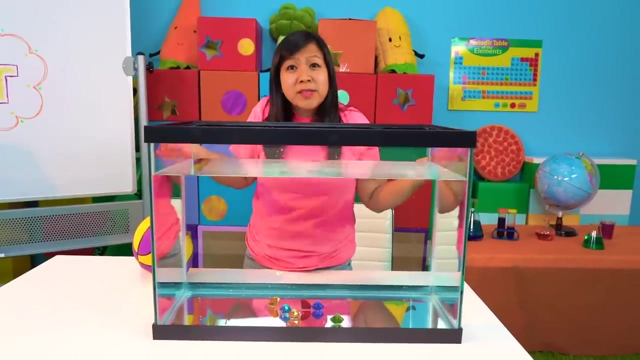 Do you guys think they'll float in water? But they're heavier. Does that make a difference? Let's see One, two, three, Oh no, Wow. So what does this mean? These stones are more dense than water. 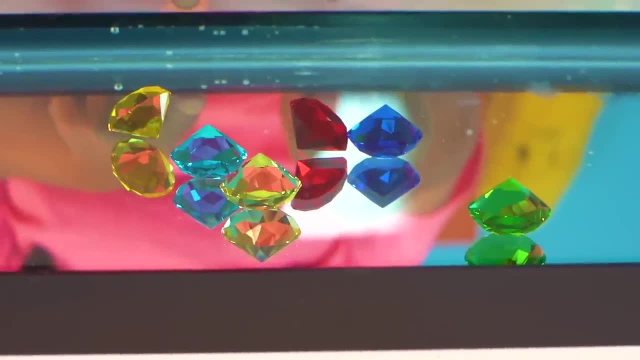 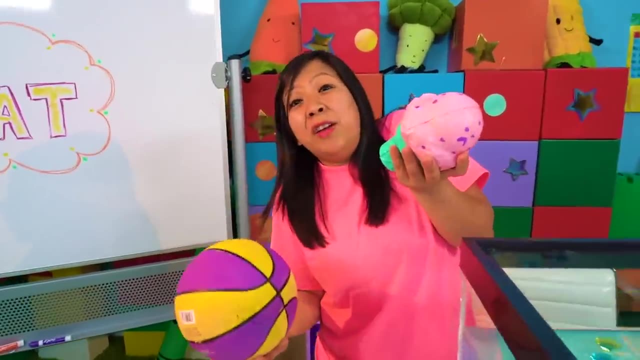 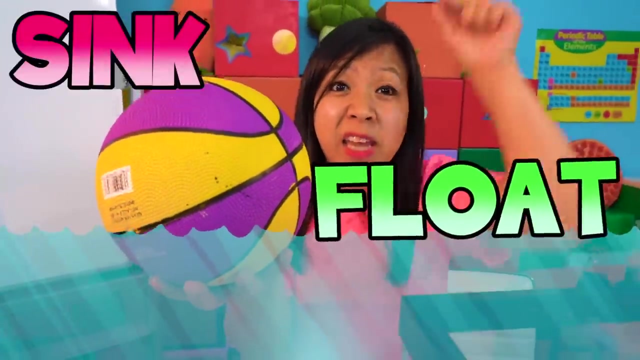 Look, They sink all the way to the bottom. Next we have a basketball. Look It bounces. It's heavier than the squishy toy. It is bigger than the squishy toy. Do you guys think this will float or sink in water? 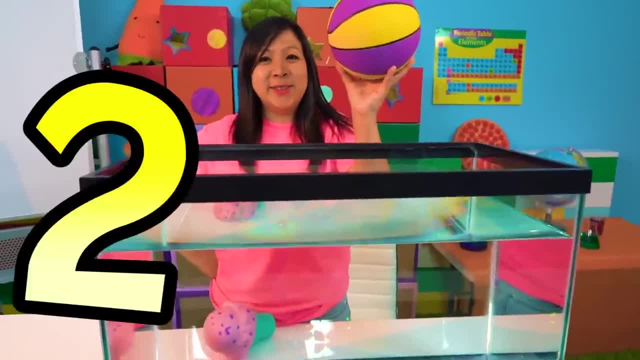 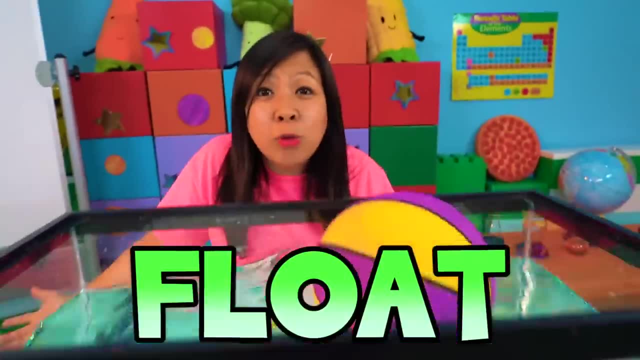 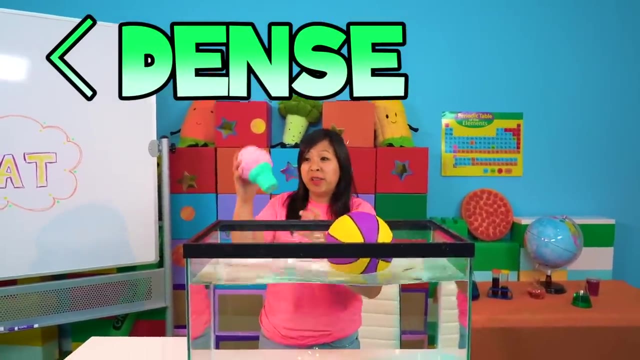 All right, Let's test it out. One, two, three, Whoa. What did you guys notice? It floats in water. What does that mean? It's less dense than water, Even though it's bigger and heavier than the squishy toy. 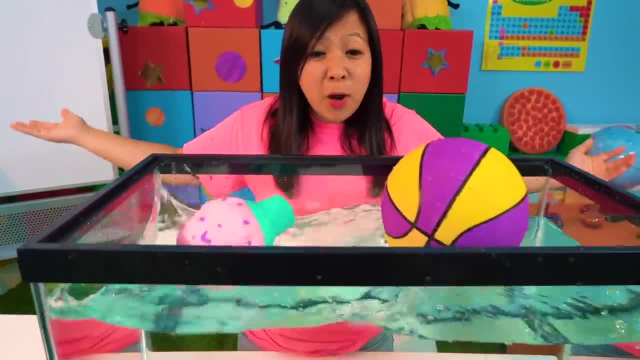 They both float. So why does the basketball float? Well, it's hollow and empty inside and it's full of air, And air is less dense than water, so it helps the basketball float. Woohoo, I have an idea. Let's go grab a whole bunch of other stuff to try. 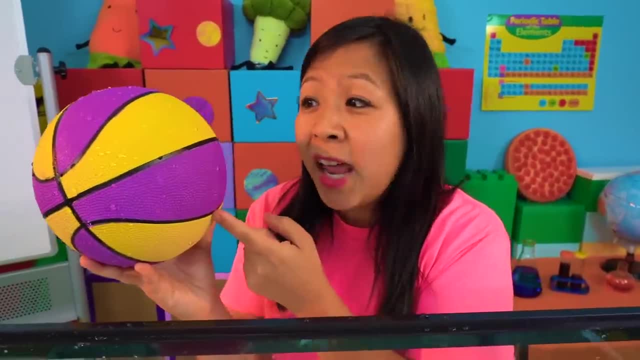 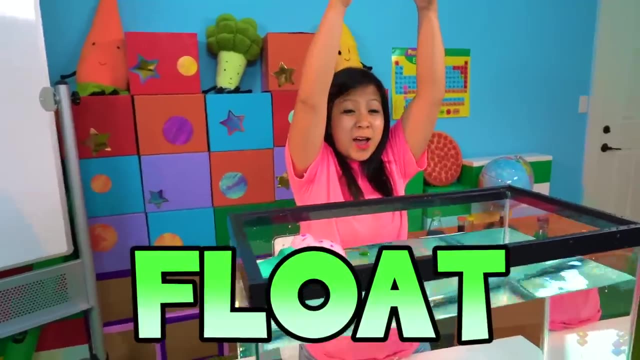 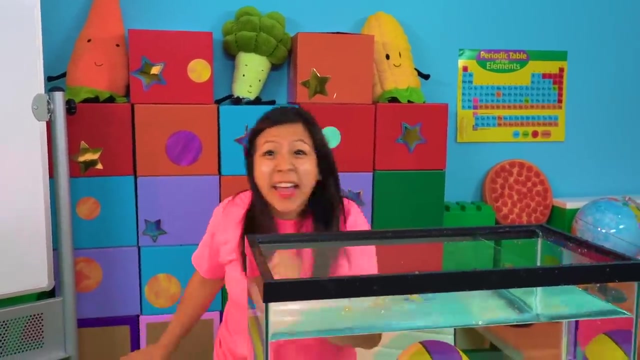 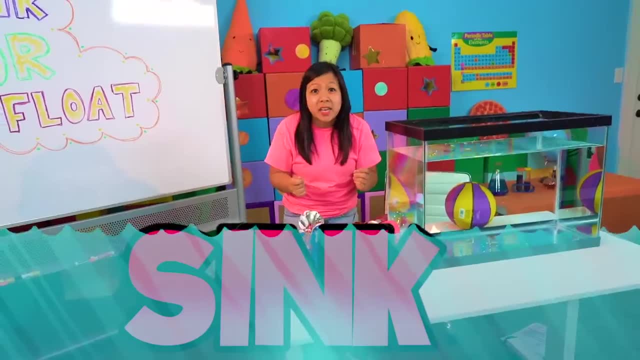 Okay, Okay, Okay, Let's go. Okay, guys, I have a whole bunch of stuff for us to try, Okay. So remember, an object will sink if the density is greater than water, and an object will float if the density is less than water. 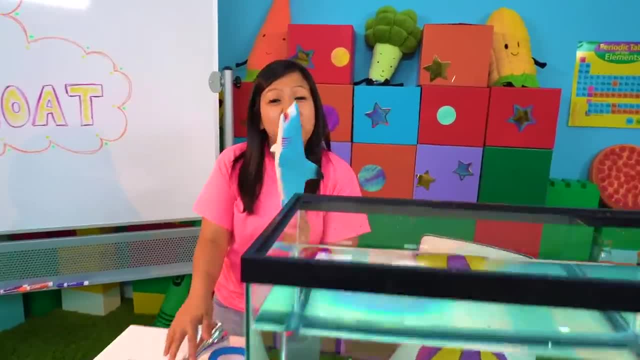 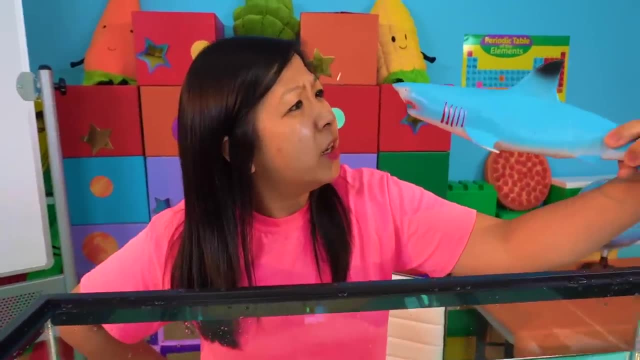 So let's see, Mr Shark, you want to give it a try? It's not a real shark, It's a toy shark. Sink or float, Let's see. Are you greater than water for density or less? One, two, three. 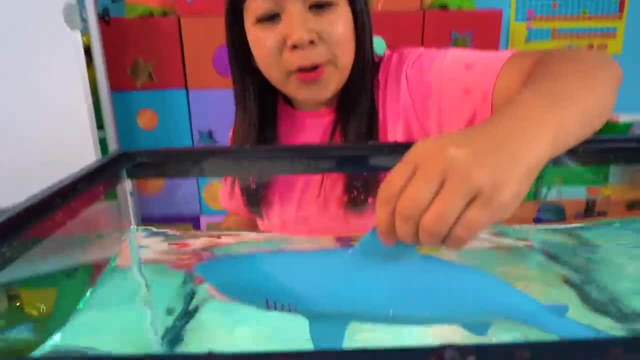 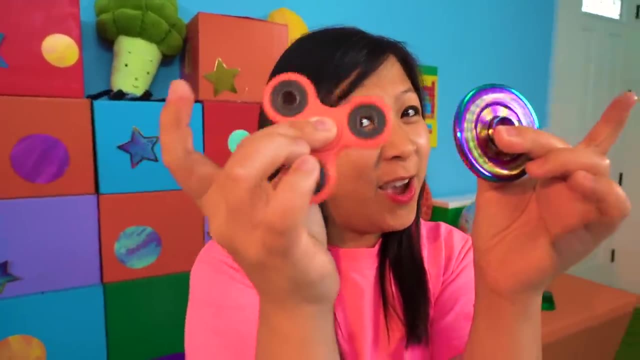 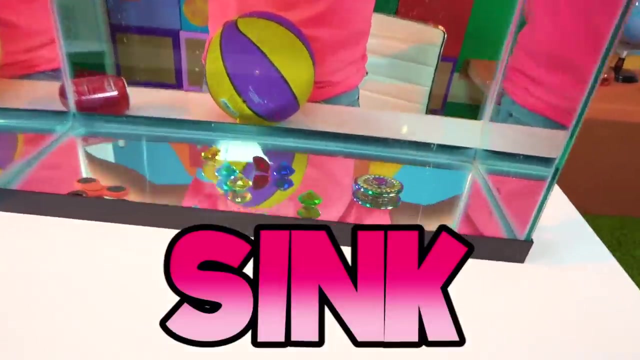 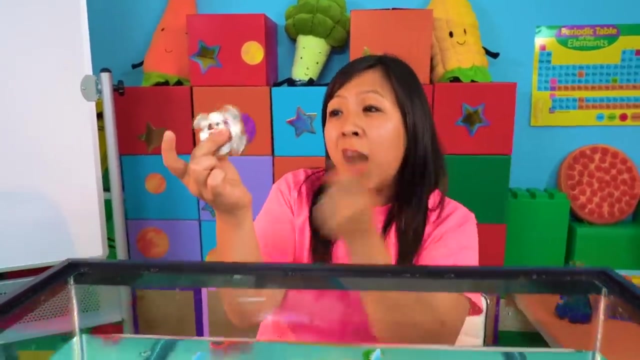 Wow, must have a lot of air inside. Do you guys remember these Fidget spinners? sink or float? Let's test it out: One, two, three. So what does that mean? The density of fidget spinner is greater than water. 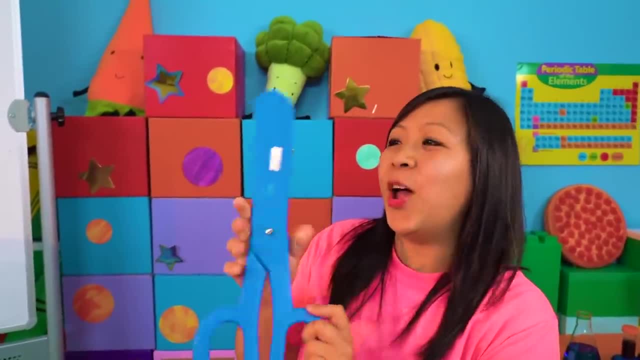 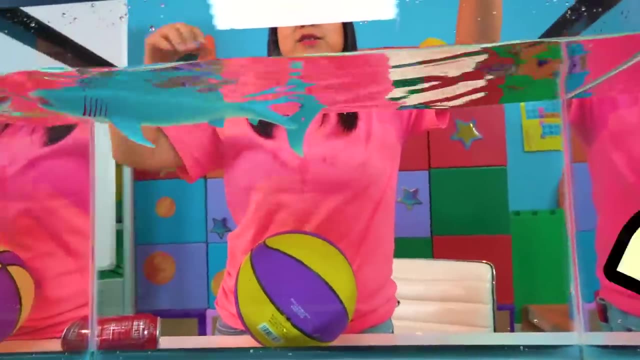 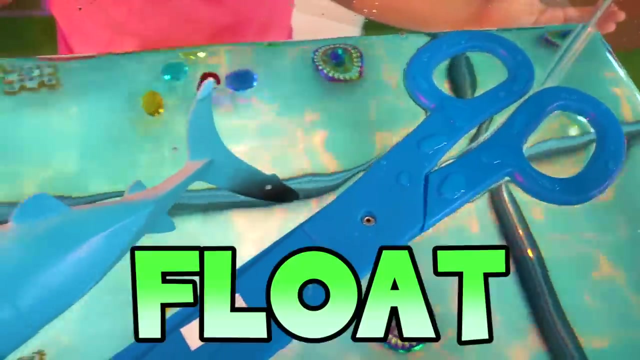 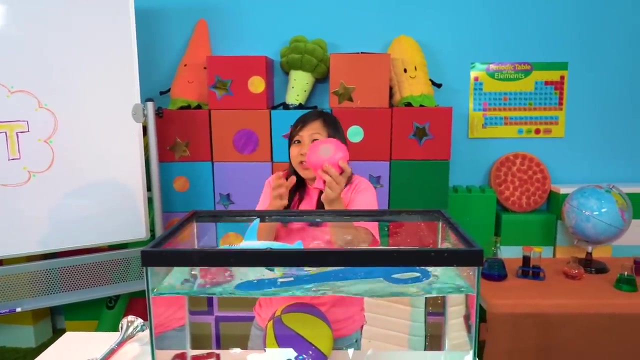 Next, scissors. So this is a plastic scissor, but we're gonna see if it sinks or float in water. You ready, One, two, three. It floats. Did you guys guess that right? So these are less dense than water. Okay, Whoopee cushion. Okay alright, Sink or float. 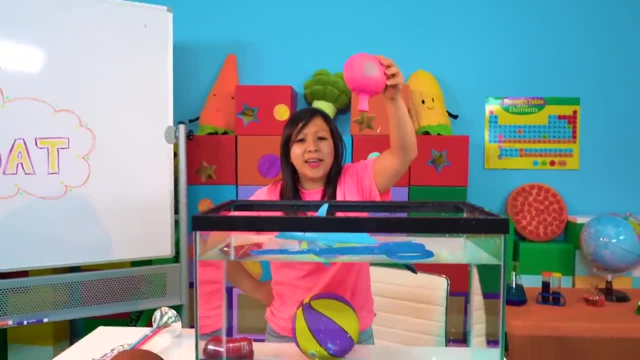 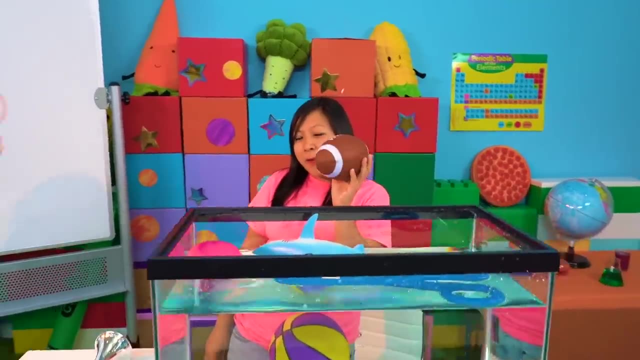 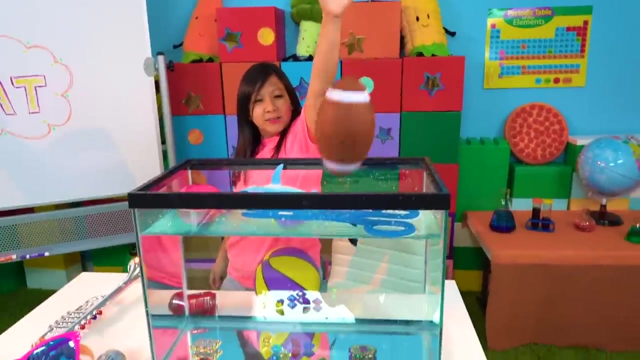 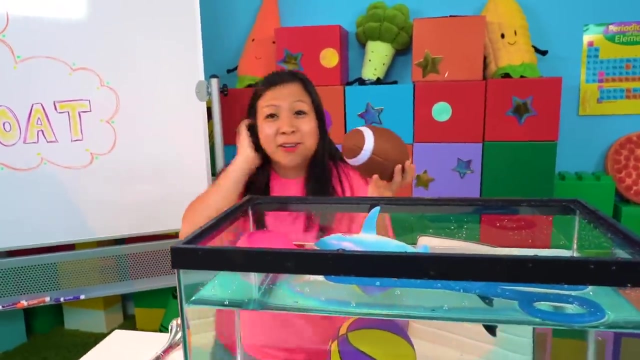 What do you guys think? One, two, three. One, two, three, Also floats. Who likes to play American football? Hut, hut, pew Sink or float. One, two, three. Sorry, I'll be right back. Obviously not good at American football. 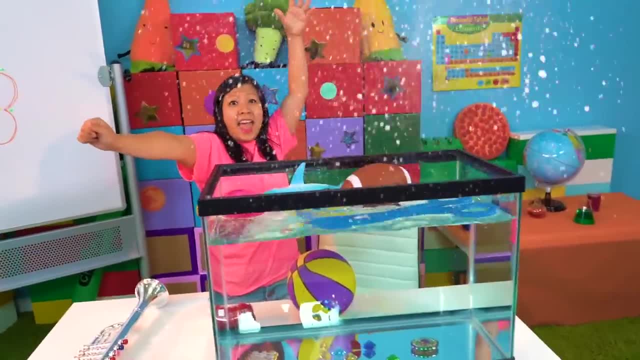 One, two, three Hut hut catch Yay. Also floats One, two, three Hut hut catch Yay. Also floats One, two, three Hut hut catch Yay. 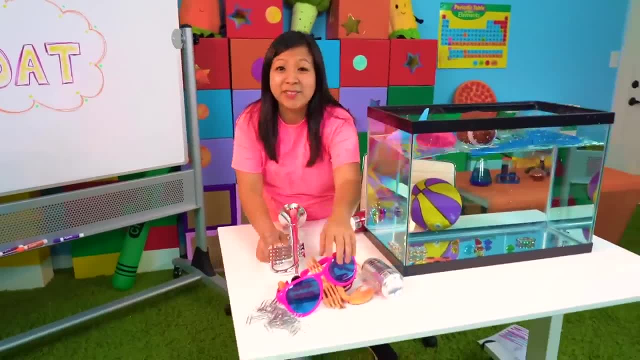 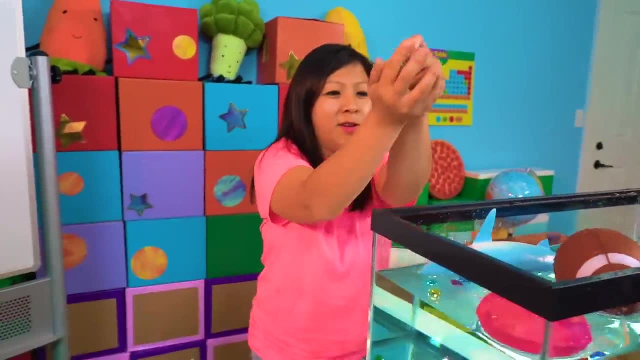 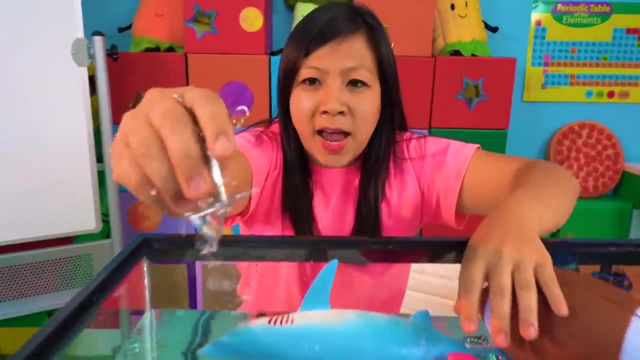 Oh wow. So far we're doing great, But here's a tricky one: Paper clips, Sink or float, Let's see. One, two, three, Move away. whoopee, cushion, Whee. So what's happening? 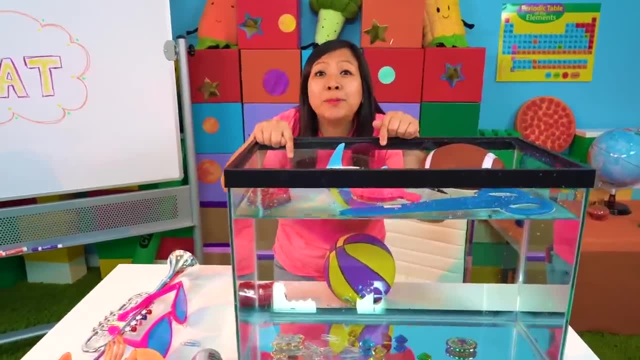 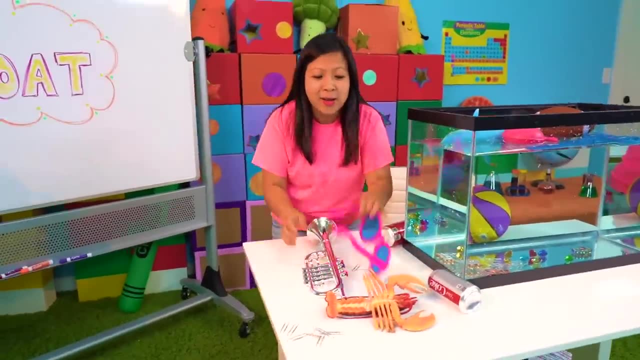 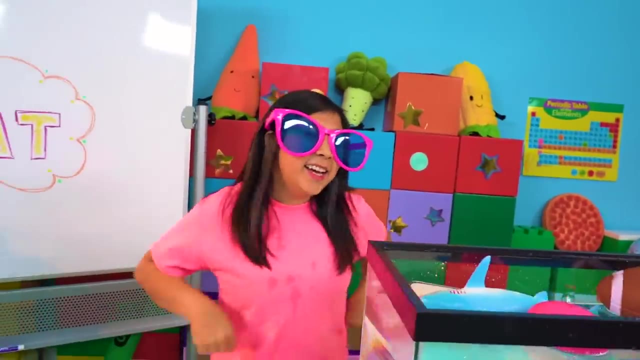 They all sink. That means the paper clip's density is greater than water. Okay, what's next? This is so fun. What about the giant glasses? These sink, or float, Any guesses? Alright, Bye-bye. glasses One, two, three. 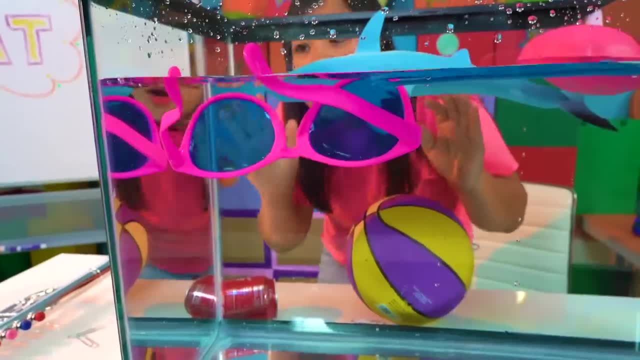 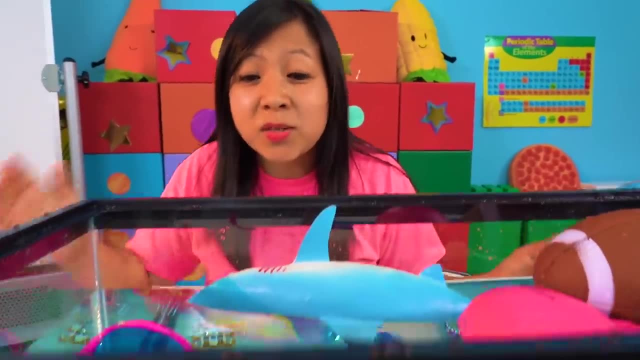 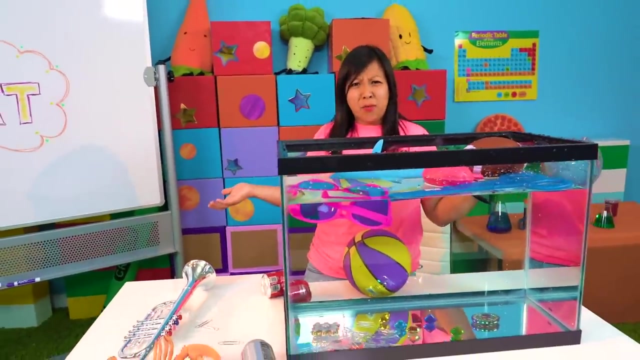 Is it gonna sink or is it gonna float? It's hovering. It's hovering. What do you guys think? I think it's pretty close to water's density. That's why it's right there in between sinking and floating. So, since you guys didn't ask what is the density of water, 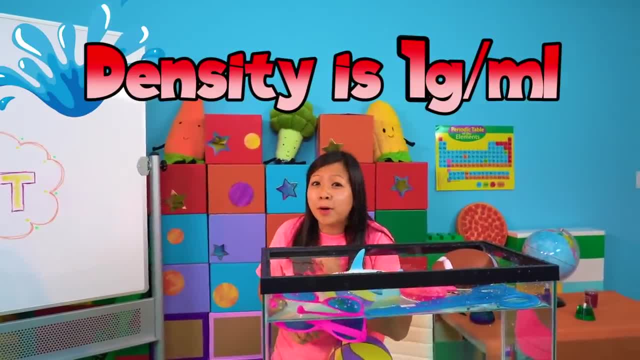 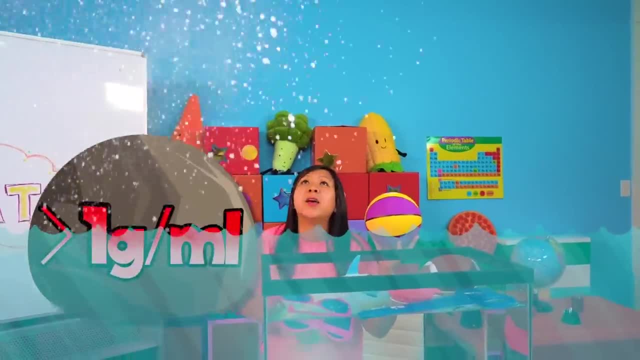 It is. the density of water is one gram per milliliter, So any time an object's density is greater than one gram per milliliter, it sinks. Any time an object's density is less than one gram per milliliter, it floats. 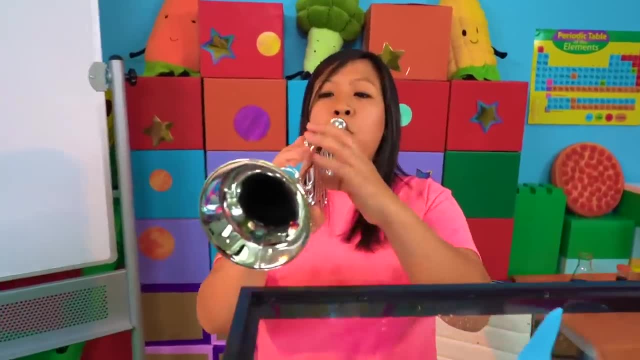 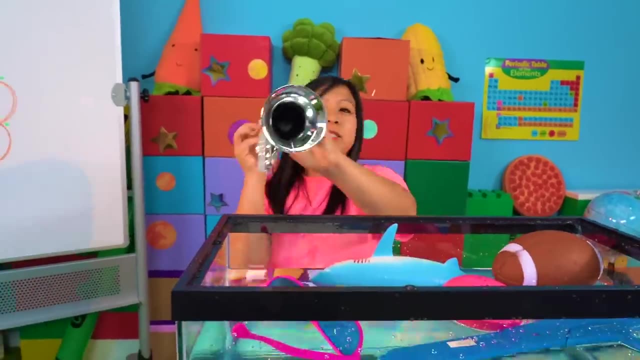 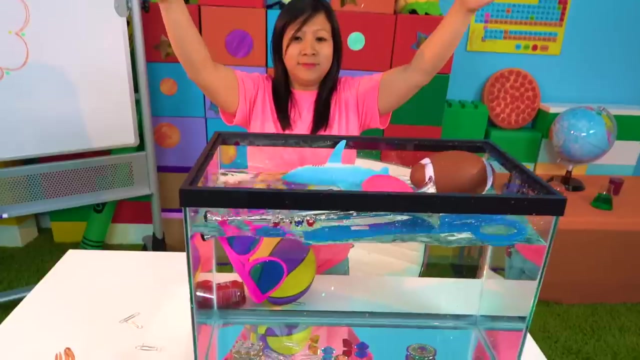 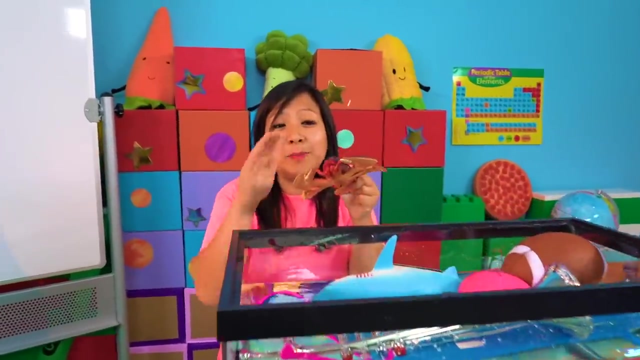 Um, what else? Trumpet, Sink or float, Don't forget, there's lots of air inside here, lots of holes, and it's pretty plasticky. One, two, three Float. Alright, Lobster, You guys like lobster? 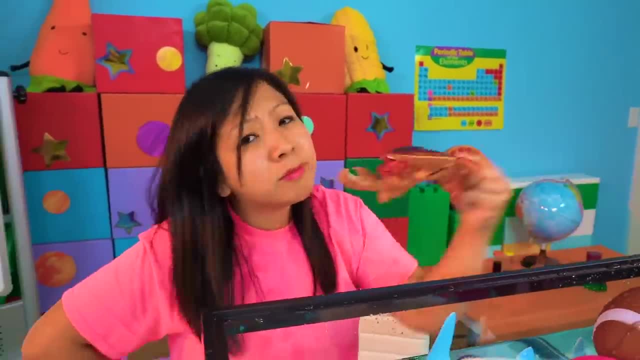 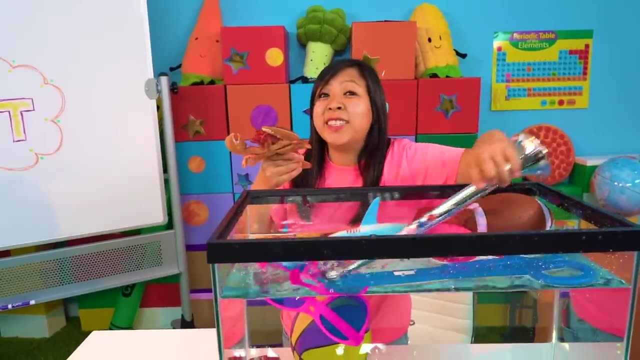 Hey, Mr Lobster, do you sink or float in water? Well, I am a lobster, so I think I'm going to sink. Oh, okay, Let's see. if it's true He thinks he's gonna sink, What do you guys think? 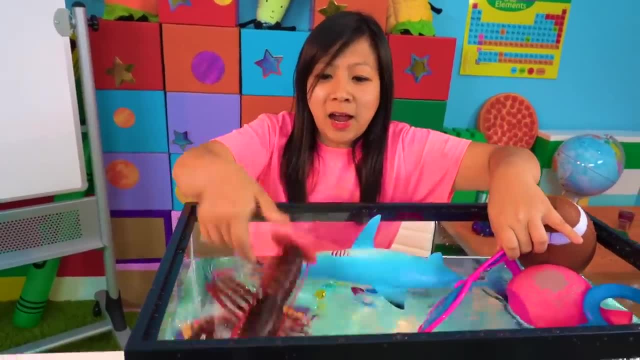 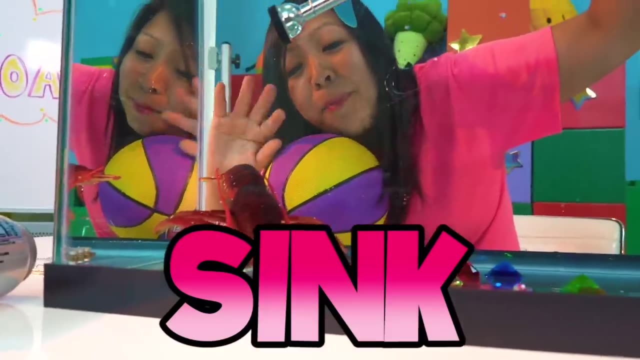 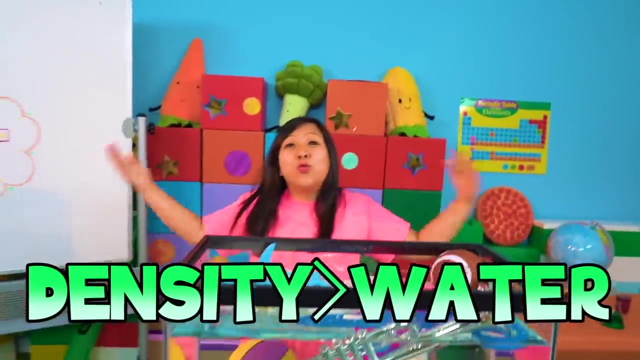 One, two, three. Oh, Mr Lobster did sink. Bye-bye lobster. Good thing he likes water, huh. So what does that mean? Density is greater than water. Okay, we're gonna clear out the tank because I have a super fun experiment. 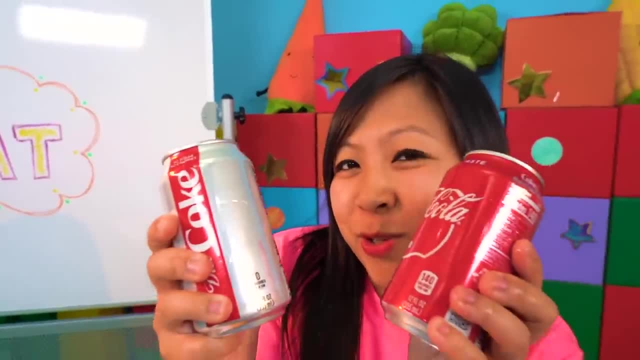 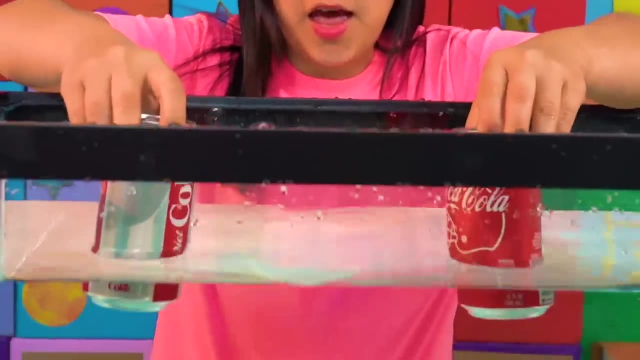 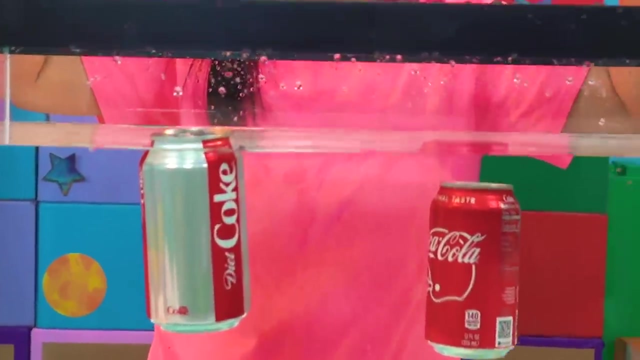 Diet Coke versus regular Coke, Which one will sink and which one will stay afloat? Alright, let's put it into the water. Okay, guys, we have to wait. okay, Something cool is gonna happen. Wow, Look what you guys noticed. 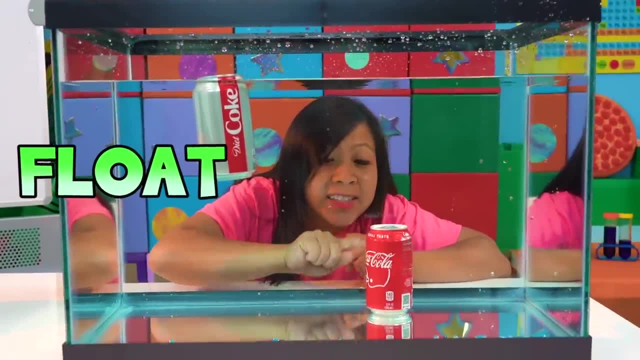 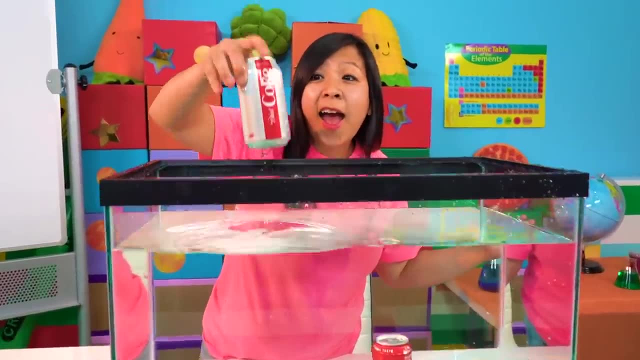 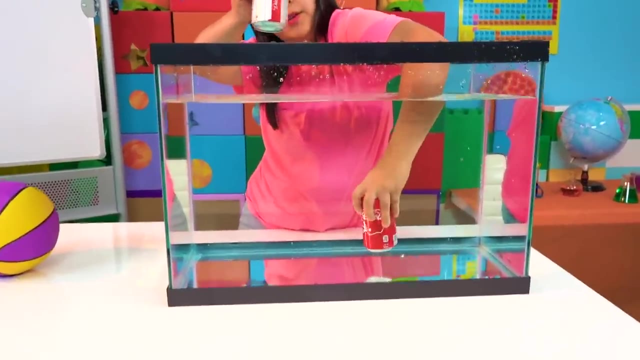 That Diet Coke float and that regular Coke sink. So what does this mean? The Diet Coke is less dense than water, But the regular Coke- Oh, where are you regular Coke? There you are- is more dense than water. 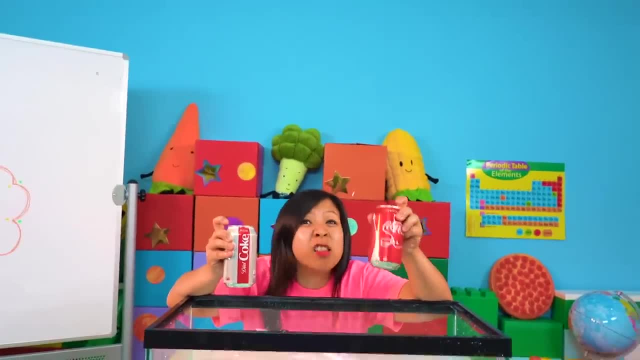 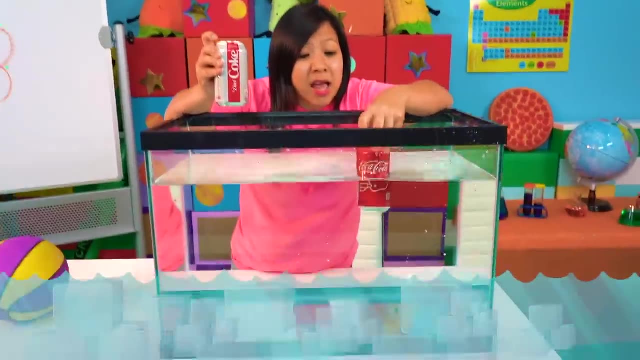 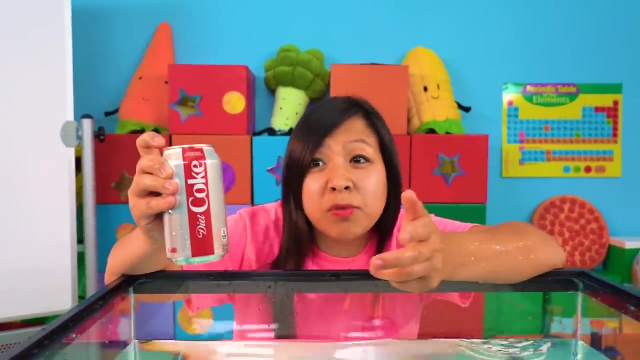 Do you know why? Because this actually has lots and lots, and lots of sugar inside. So the sugar is more dense than water, so it sinks. the Coke Ding ding ding, And the Diet Coke actually has less than one gram of sugar. 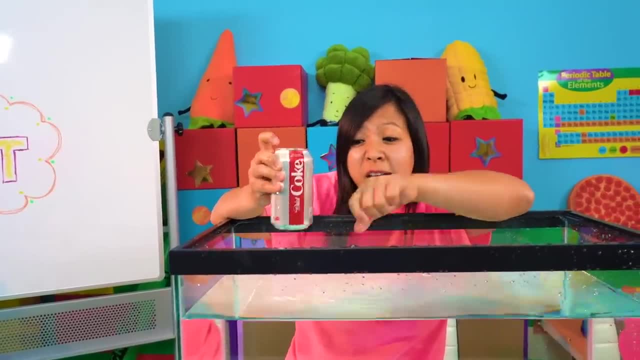 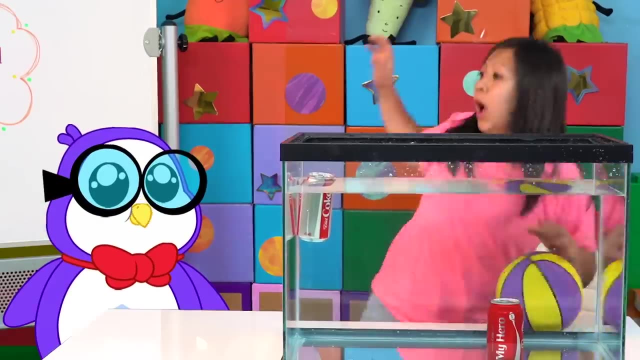 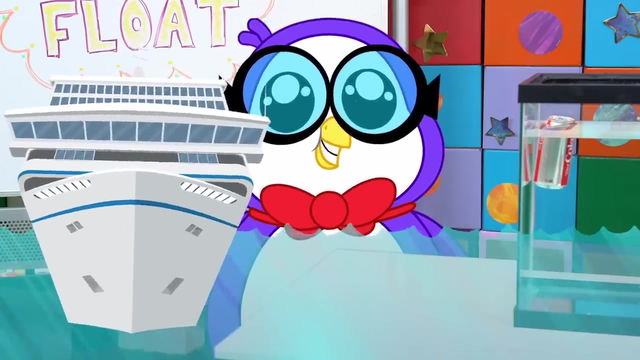 So mostly just water and air inside, so it floats. Wow, Excuse me, Ms Ryan's mom. Yes, Peck, I'm doing some homework on buoyancy And I'm trying to understand how these giant cruise ships are able to float in the ocean. 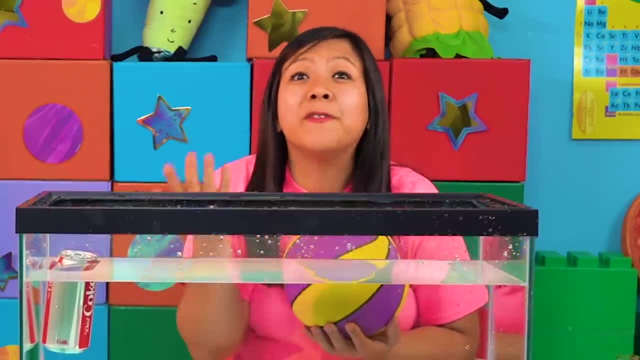 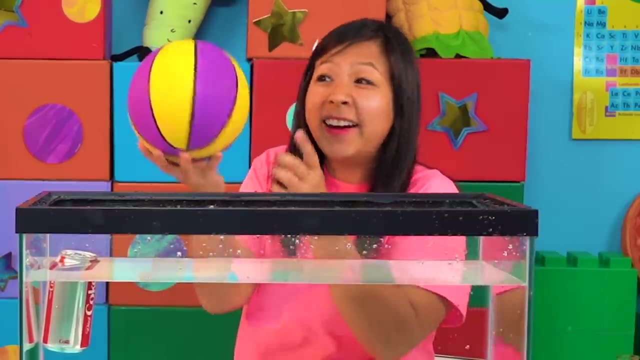 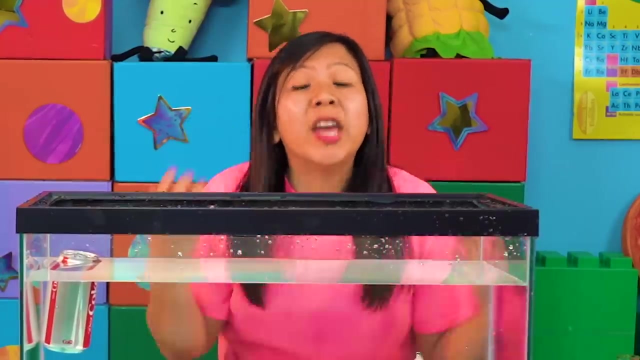 That's a good question. Peck, Those cruise ships can float in water because it's hollow, Like this basketball, Full of air. It's hollow and full of air, Got it. But that's not all. Peck It's because also the shape of the cruise ship. 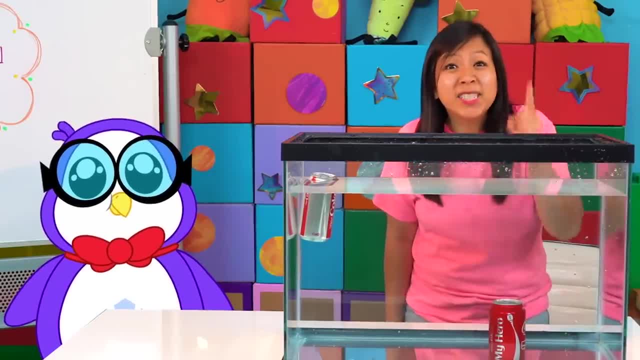 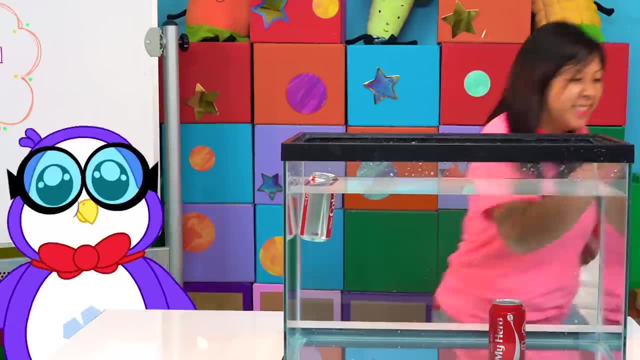 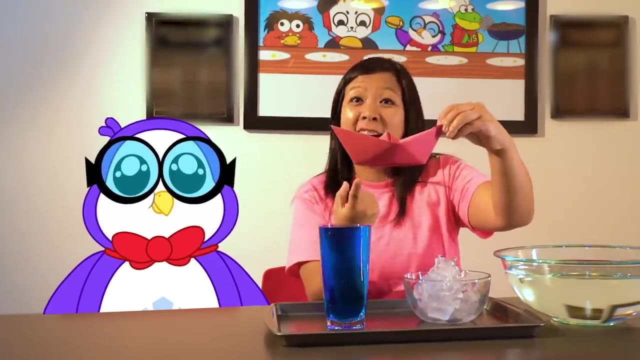 I have an idea. Let's do one more experiment. Oh joy, Another experiment. I love experiments, Let's go. Did you know that ship is shaped so that most of it is above water? That way it doesn't displace too much water. 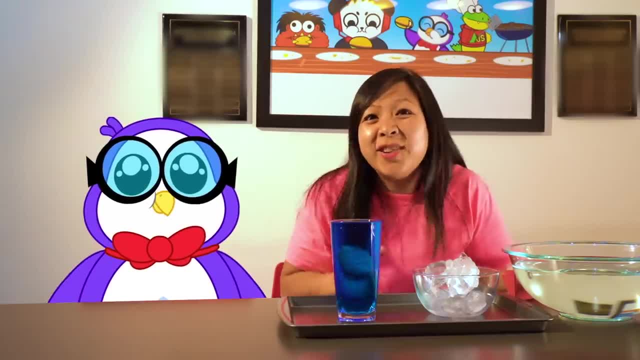 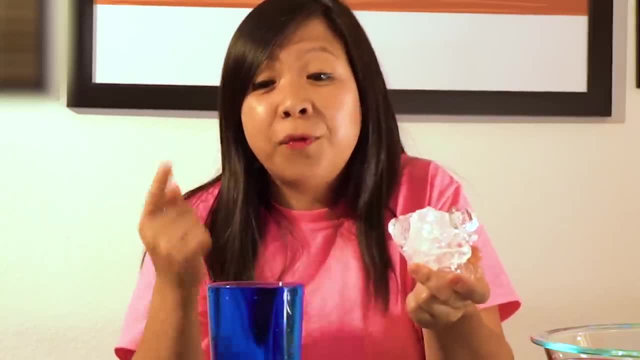 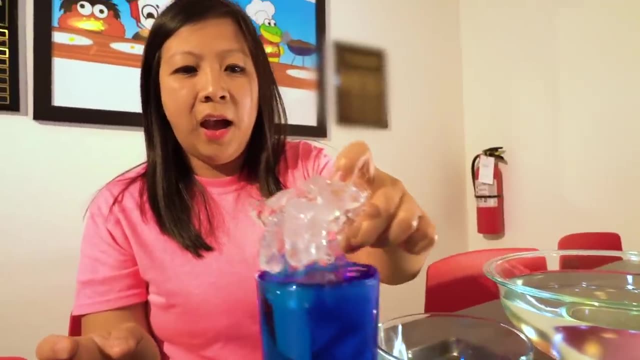 Displace. Yeah, Let's try this. I'm going to put ice- Oh it's cold- In this cup that is full of water and see what happens. You guys ready? Oh, it's so cold, Okay, Wow. 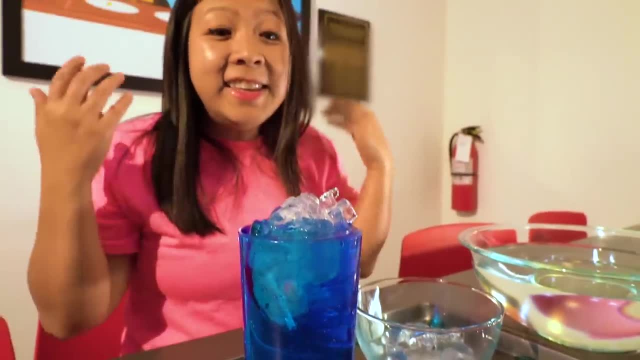 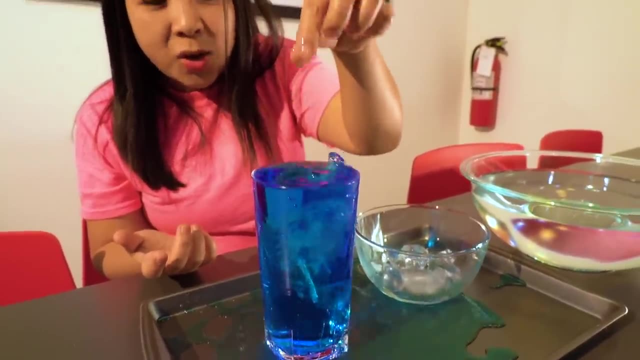 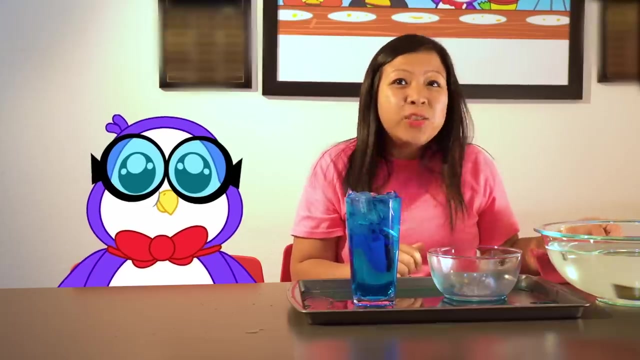 Whoa, The water spilled everywhere. Yeah, So when we put the ice in a cup of water that's already filled, the water spills out, right. So when an object pushes water out of the way, this is called displacement, Yeah. 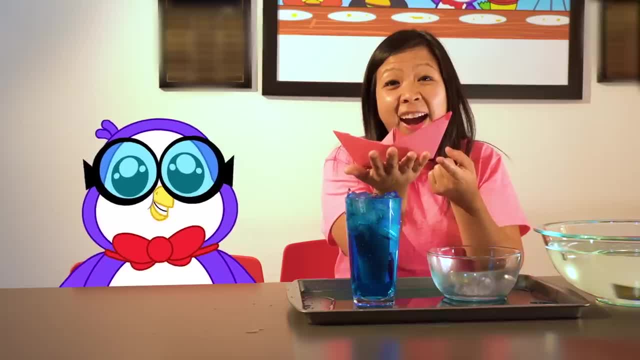 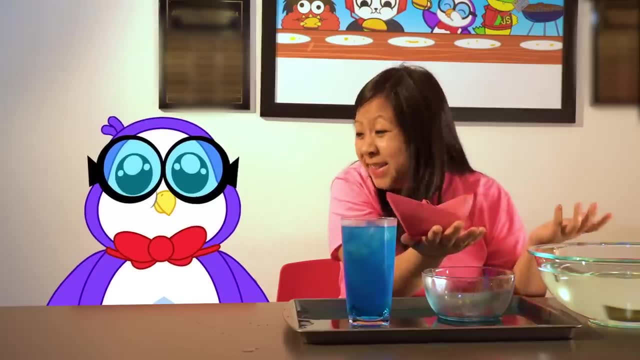 So this is why ship don't sink. They are hollow like the basketball and full of air, and they're shaped so that they don't displace too much water. That's right. Oh joy, I can finish my homework now. Thank you, Ms Ryan's mom. 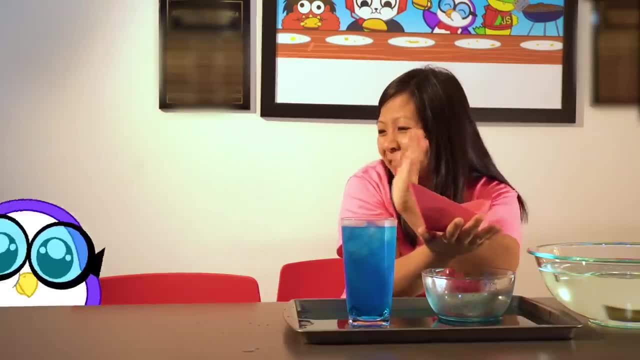 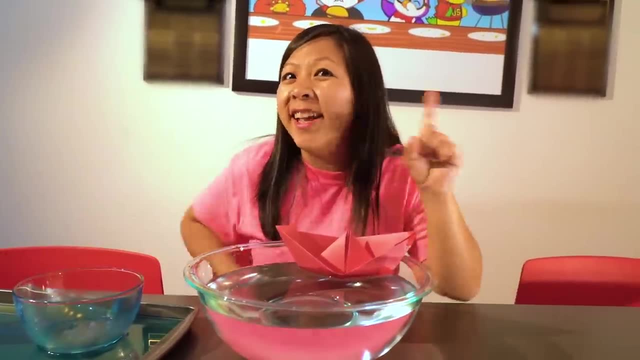 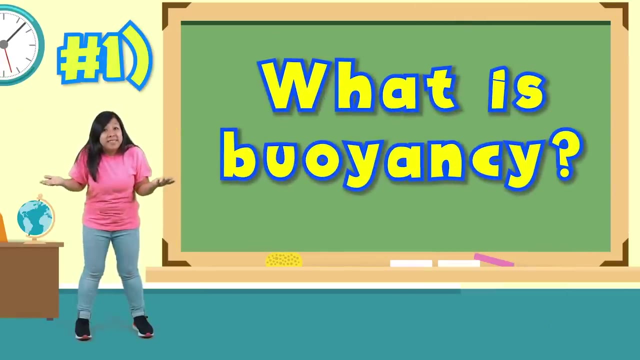 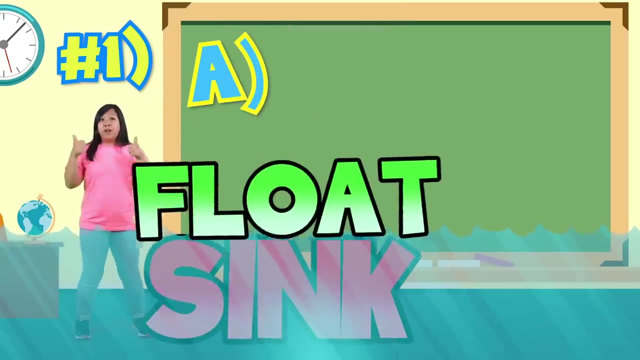 See you later. You're welcome, Peg Bye. So I think that now we're an expert on objects sinking or floating in water. Let's try a pop quiz. Let's go Question number one: What is buoyancy? Is it A an object's ability to sink or float? 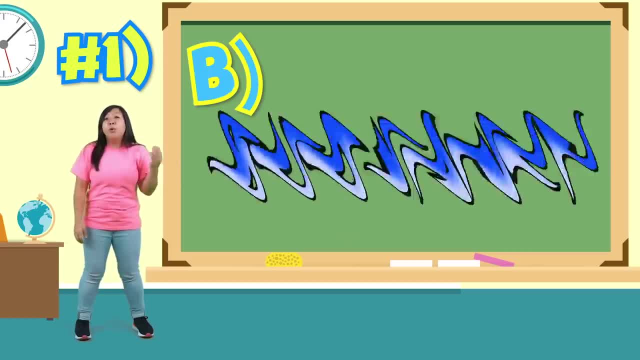 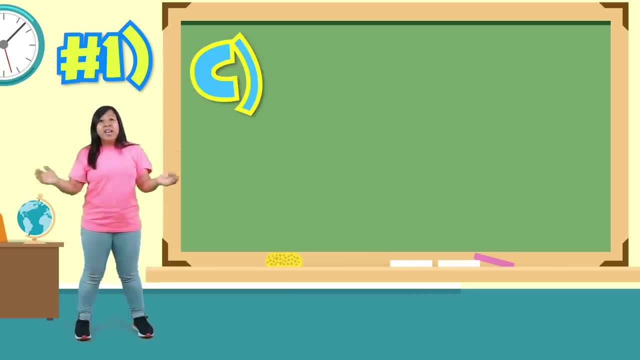 Or is it B? buoyancy is a buoyant, Or is it C? is buoyancy a cheeseburger? Any guesses? The answer is A. buoyancy is an object's ability to sink or float. Yay, All right guys. 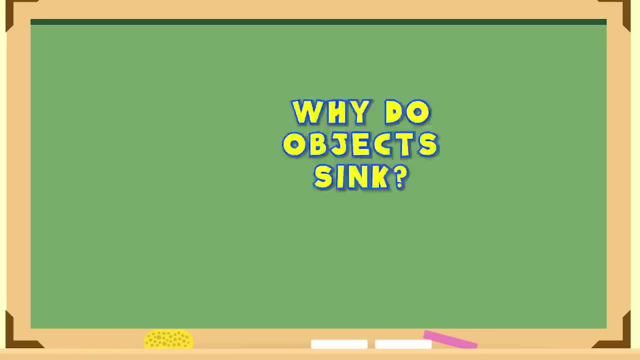 We move on to question number two. Why does object sink? Is it because A- they're blue- All objects that are blue float. Or is it B- they like to swim. Or is it C- they are more dense than water? 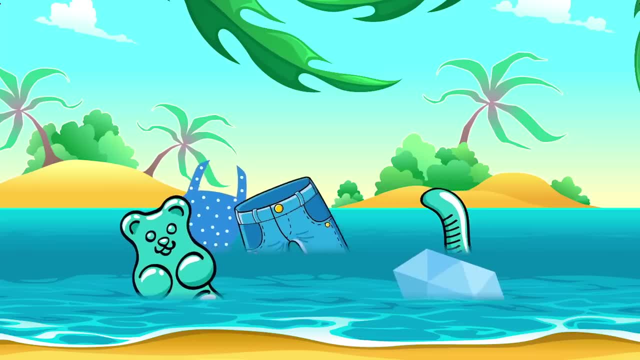 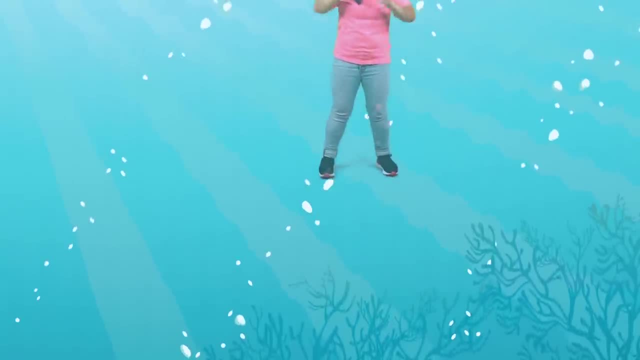 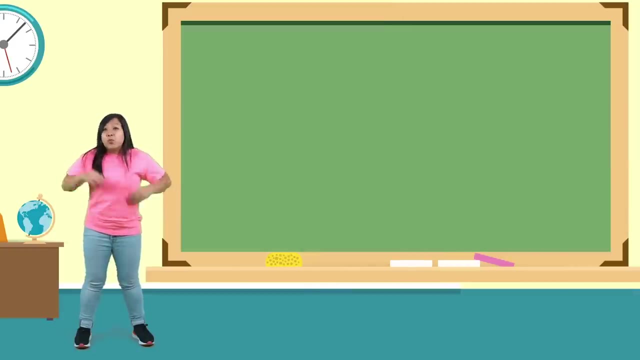 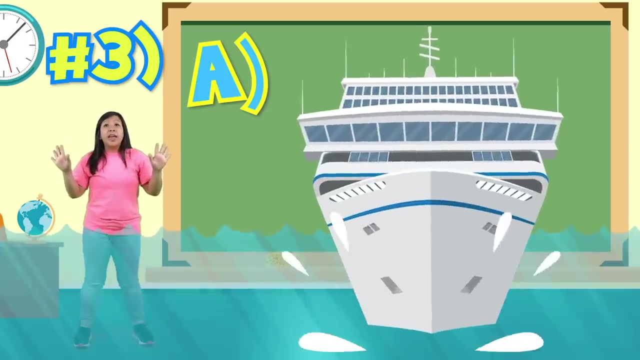 So what's the answer? Why do objects sink? It's because C- they are more dense than water. Question number three: Why do objects sink? Question number three: why do ships float? Is it because A- they're hollow and full of air? 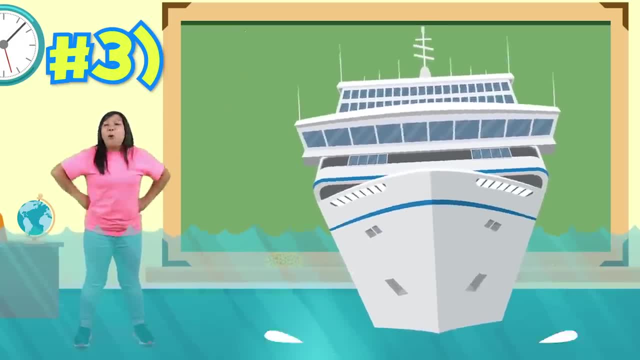 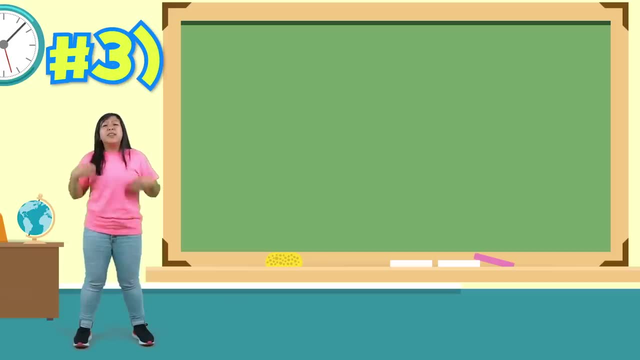 and they're shape doesn't replace too much water. Or is it because B, they're made of squishy fruit? Or is it because of C, they're hungry? Do you know the answer? why do ships float? It's because of A ships float. 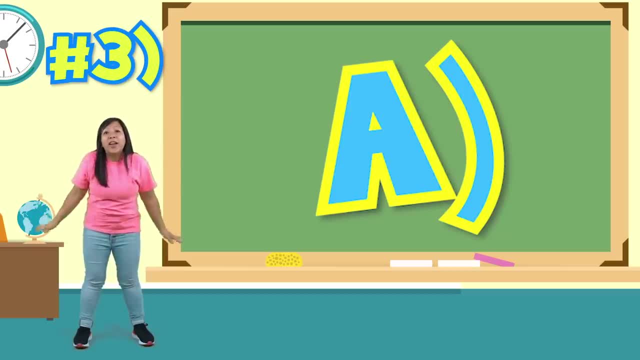 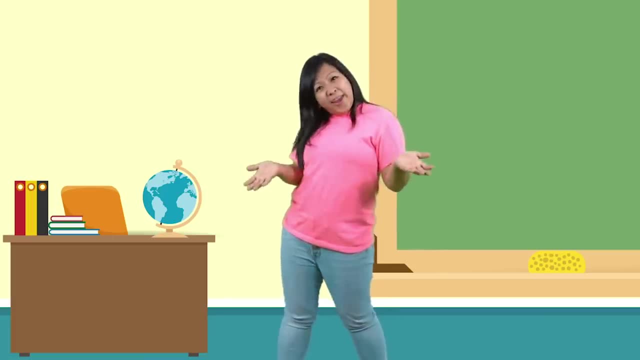 because they're hollow full of air and they're shape doesn't replace too much water. So how did you guys do on the quiz? If you didn't get it right, you can try again next time, Now that we learned so much about how objects. 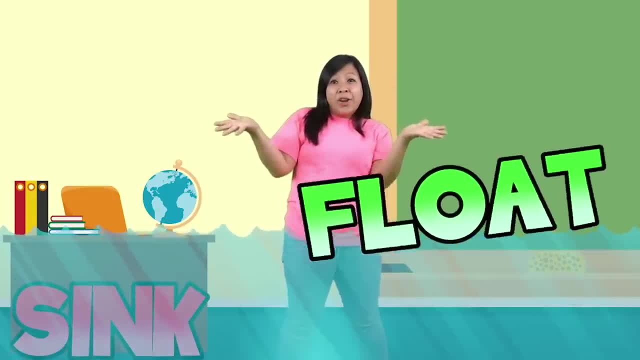 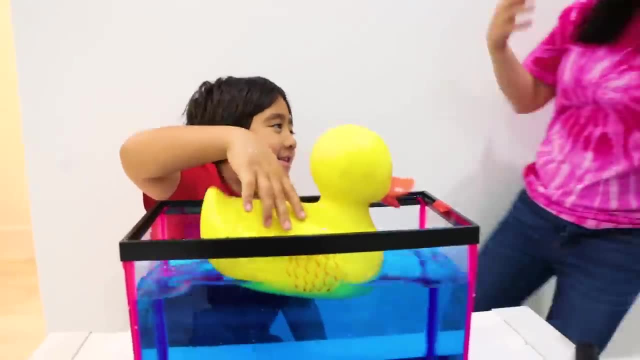 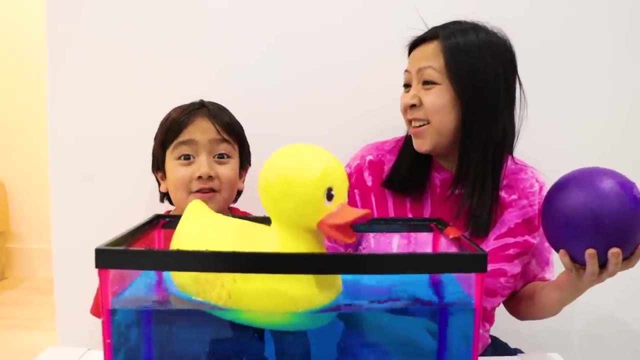 are able to sink and float into water. tell Ryan Paul about it. okay, come back, Wah, wah wah. So, Ryan, That's why some things sink and some things float. Thank you for showing me all about what sinks and floats, Mommy. 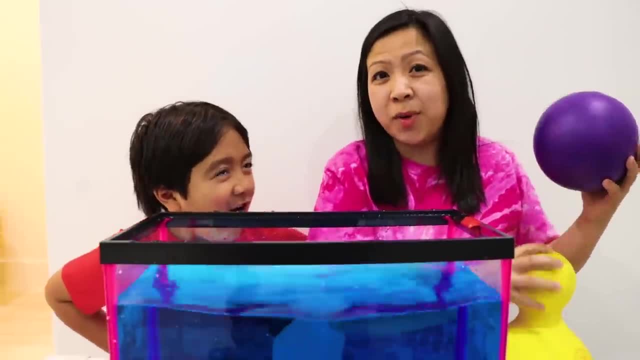 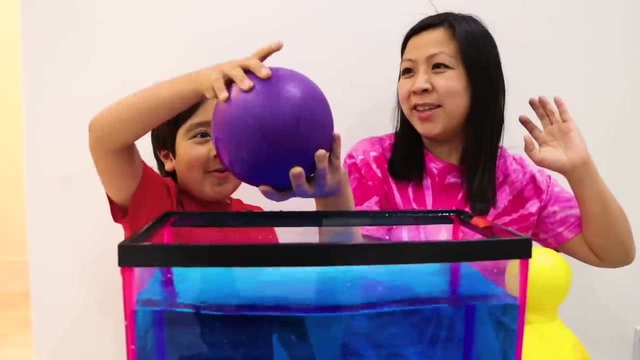 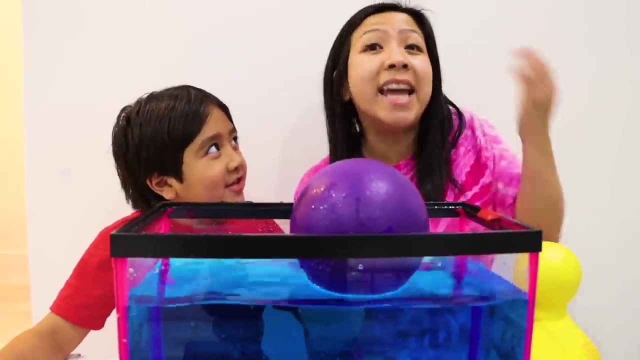 Of course. now final question for you, Ryan: Will this ball sink or float? It will float, Okay, let's see. if Ryan's right, Yay, Good job now. does that mean this ball is less dense than water? 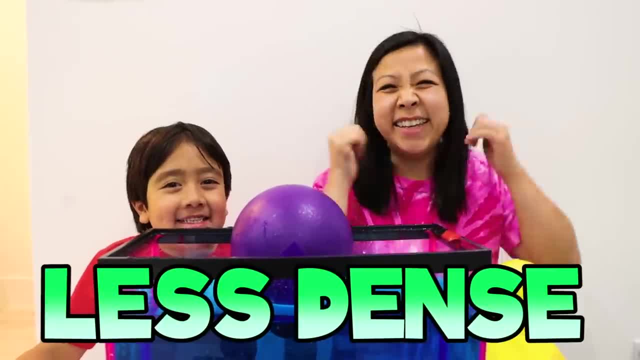 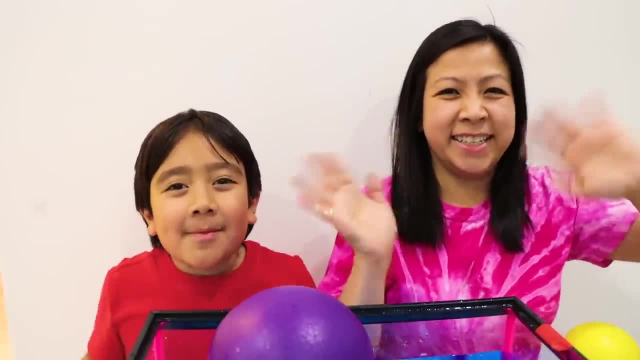 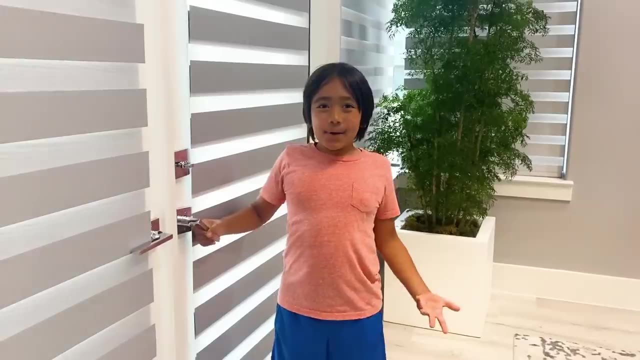 Or more dense than water, Less dense. Yay, Thank you for watching our sink and float video. bye, Remember, always stay happy and rise up. Bye, Hey guys, let's go outside and play. Yeah, Wait, no, I forgot sunscreen. 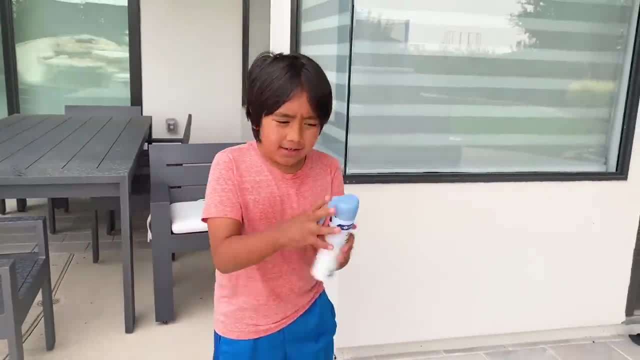 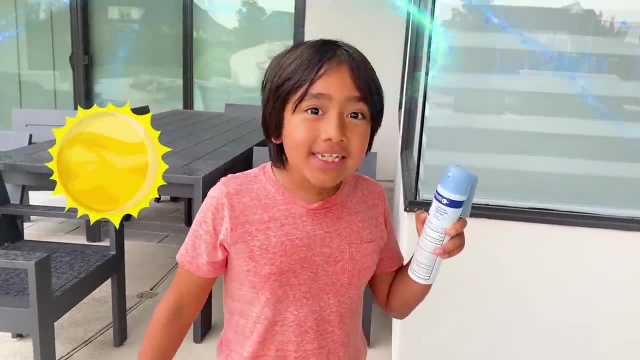 Wait, Oh no, I didn't. I forgot the sun. Did you know that sunscreen is an excellent substance that protect the skin from the sun? Let's buy some sunscreen. Just like Earth's ozone layer. Did you know Earth has a layer called ozone? 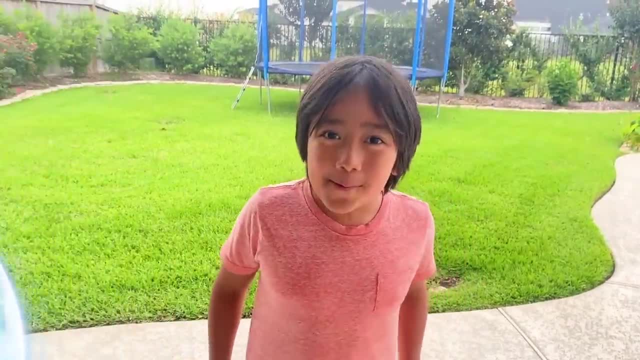 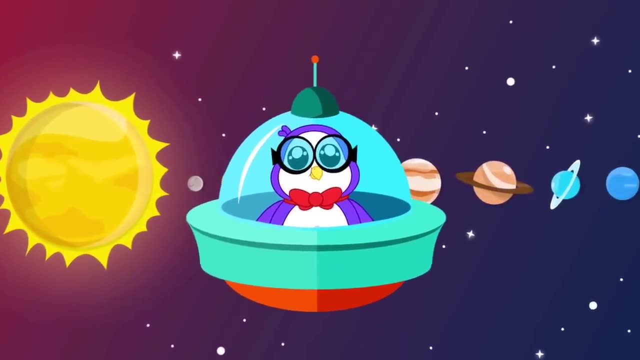 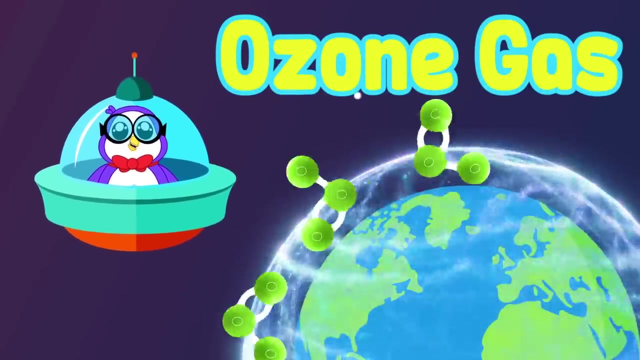 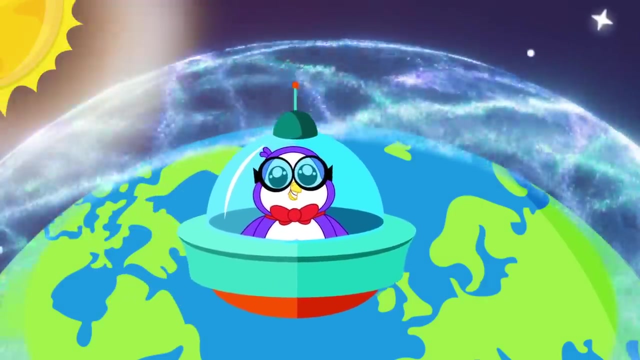 and it helps protect the Earth from the sun. Let's learn more about it. I'll take it from here, Ryan. Hi everybody. do you see that pale blue layer around Earth? That's a layer of ozone gas. It's this layer in the Earth's atmosphere that protects all living things from the sun's ultraviolet radiation. 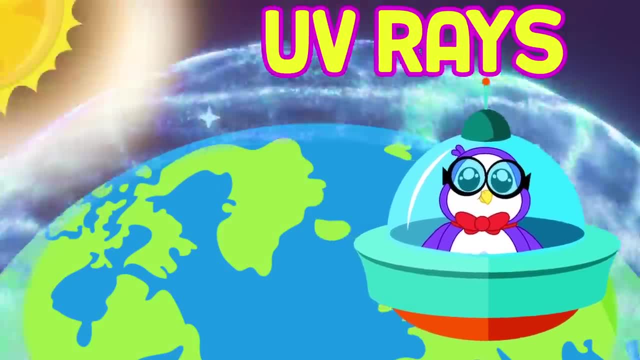 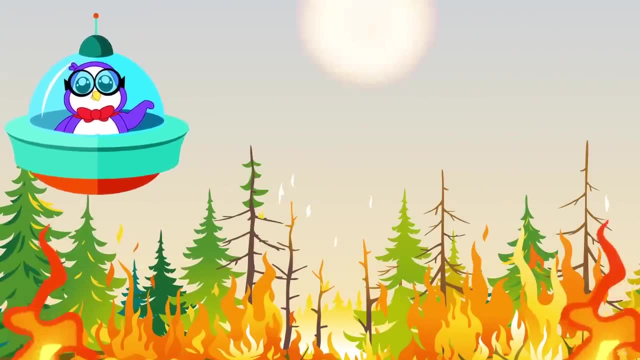 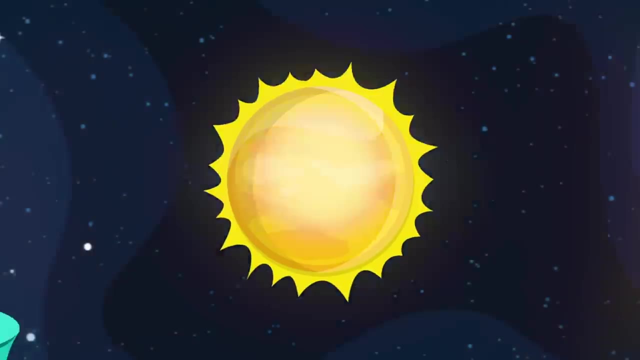 also known as UV rays. These rays can be dangerous to our skin, damaging to the plants and increase the temperatures on Earth. We have to take care of the ozone layer so it can keep protecting us. Oh gosh, look, I see a spot where UV rays are reaching. 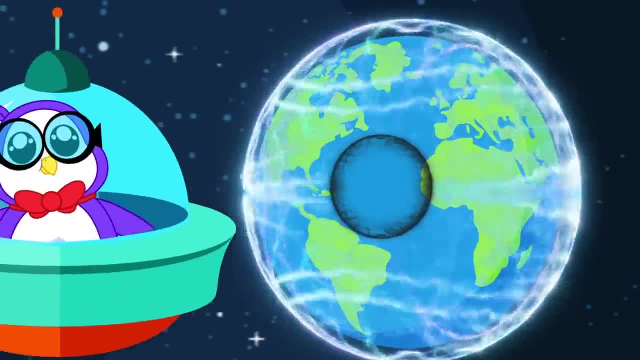 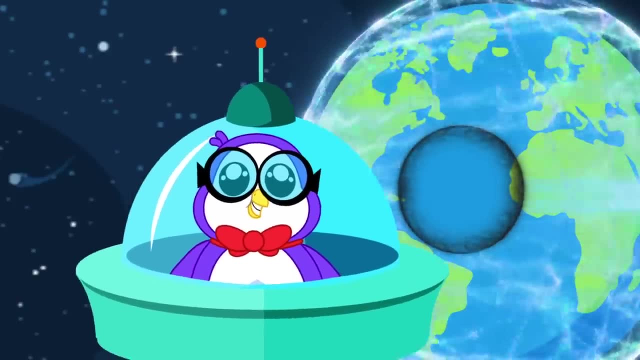 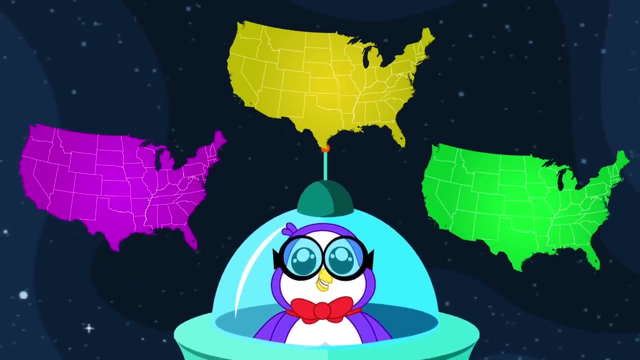 Earth. come on. Wow, look how big it is. This year, the hole in the ozone is 24 million square kilometers, which is approximately 9.3 million square miles. That's the size of three United States put together. Wow. 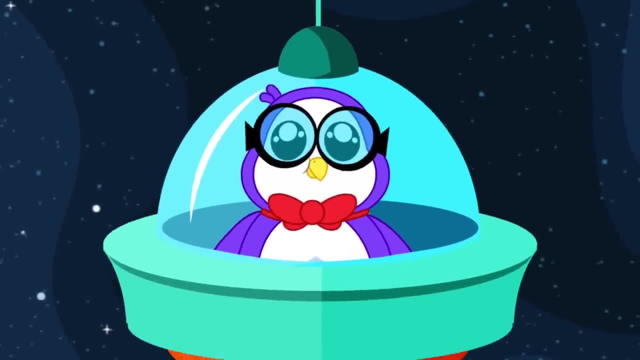 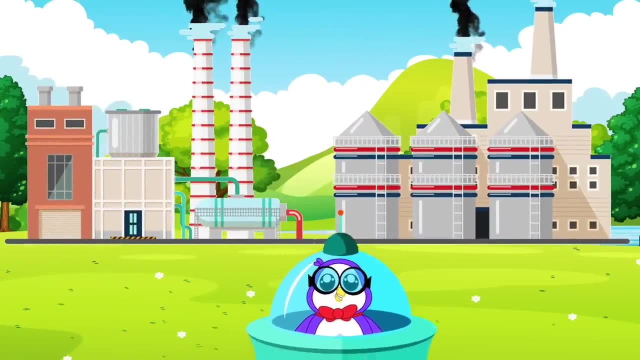 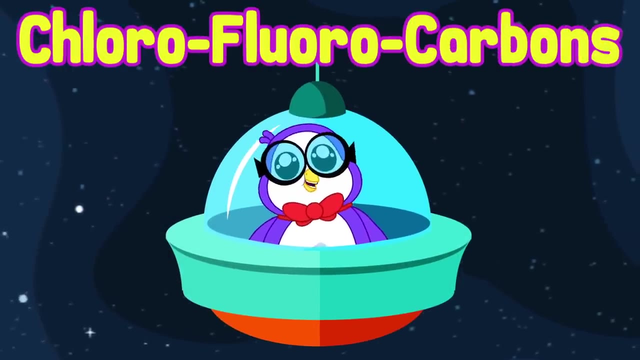 This hole wasn't always here. It was first discovered in 1985.. The world advanced with technology and industry started to relax. but it's not all these gases harmful to the atmosphere. Most of these gases are called chlorofluorocarbons. 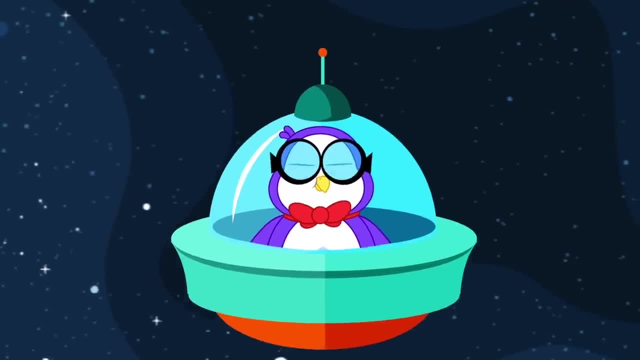 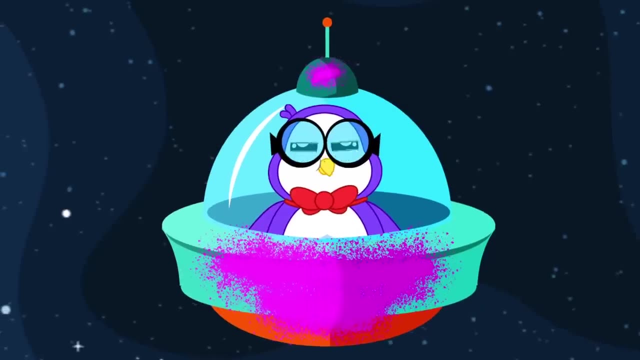 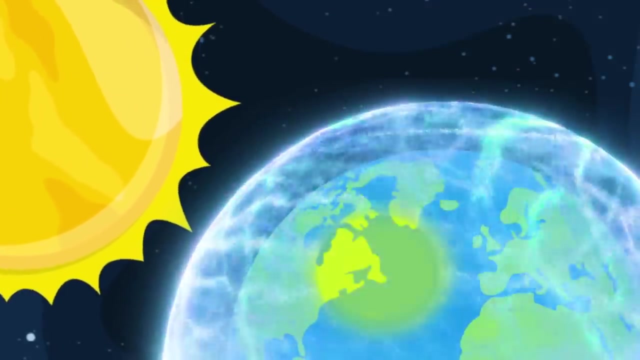 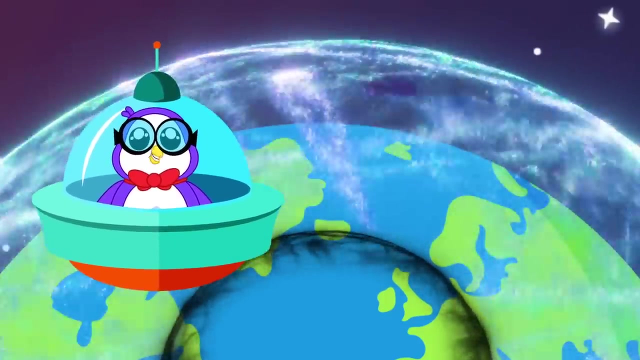 also known as CFCs. These are found in refrigerants and aerosol spray cans, So over time, the buildup of harmful gases caused this hole. Wait a second. we're floating right above my hometown. This ozone hole is located right above Antarctica. Let's go Hi Bye. On September 16th 1985, nations around the world agreed to protect the ozone layer. September 16th is officially known as Ozone Day Now that we all know about the ozone hole. 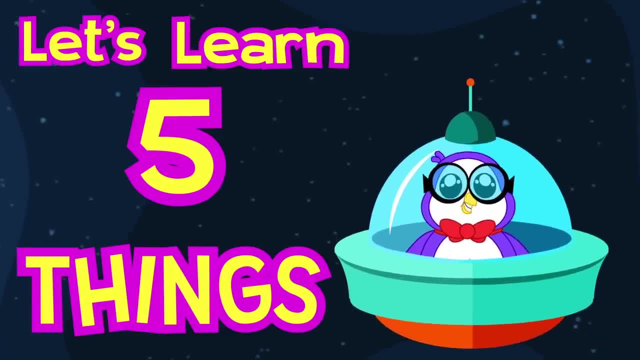 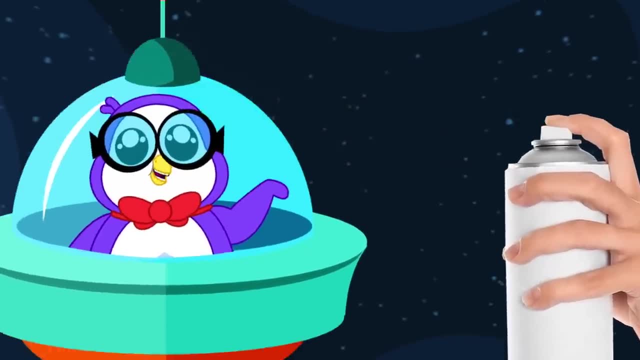 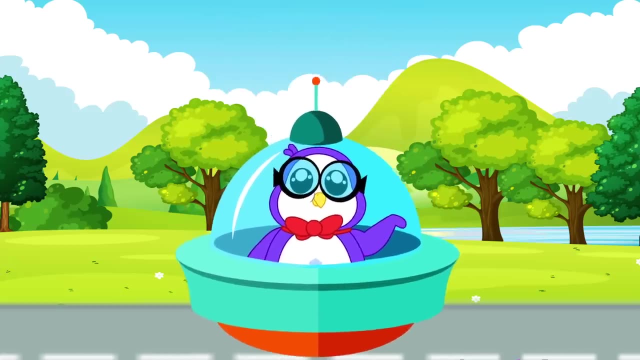 we must do our part to fix it. Let's learn five things that you can do every day to help heal the ozone. Number one: avoid any products that release CFCs or other harmful gases. Number two: reduce the use of vehicles. 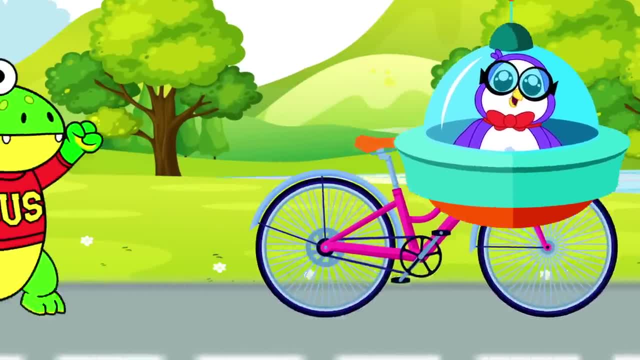 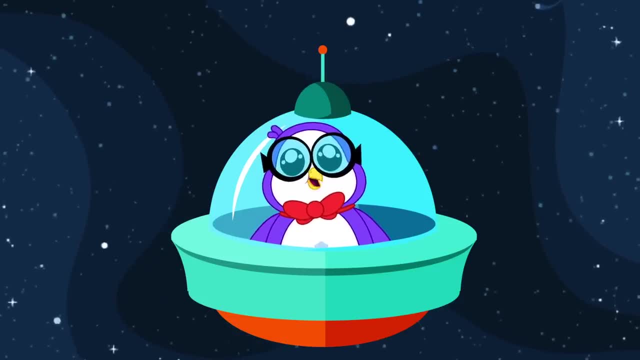 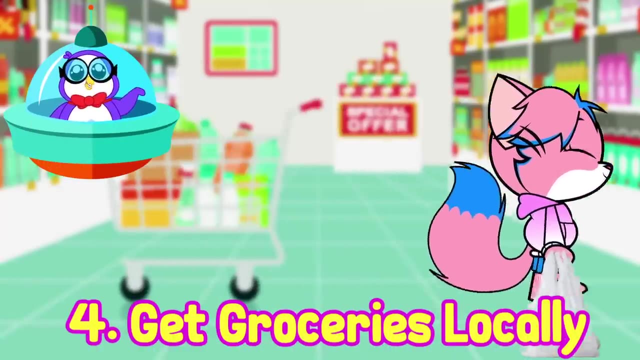 Instead of driving a car, you can ride a bike or walk, because these don't pollute the air the same way cars do. Number three: don't use cleaning products that release harmful gases. Number four: get groceries locally. It reduces waste from packaging. 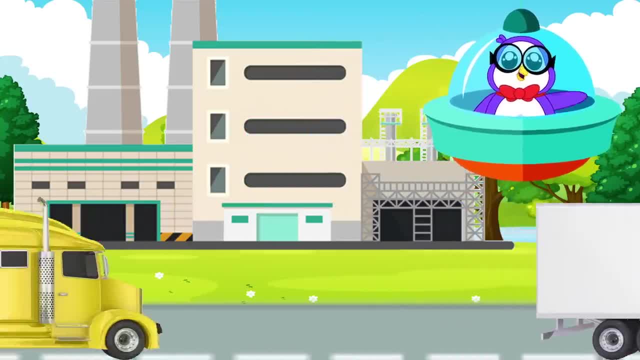 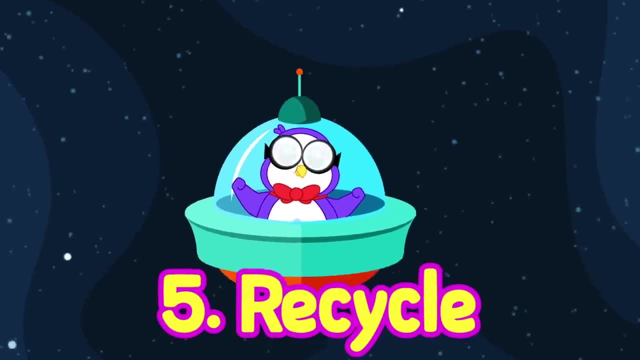 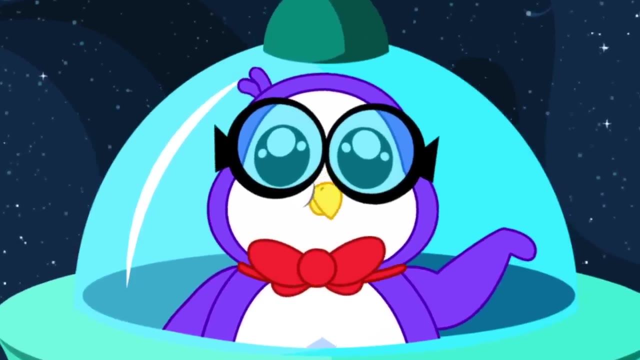 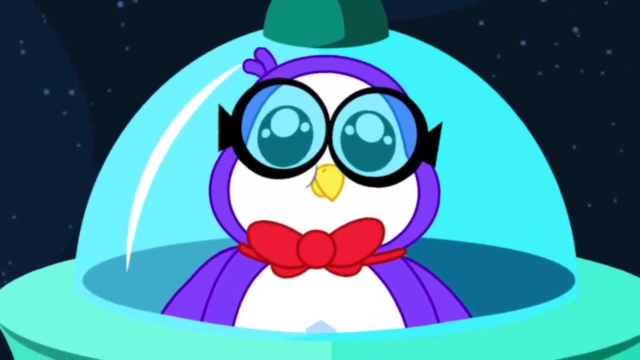 It also reduces gases being released into the atmosphere from shipping and transporting. Number five: recycle. When we recycle, we're reusing items we've used already. This means that they don't have to be manufactured again or burned, both of which release harmful gases into the atmosphere. 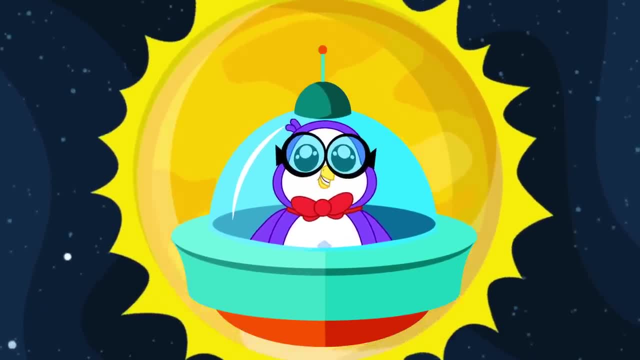 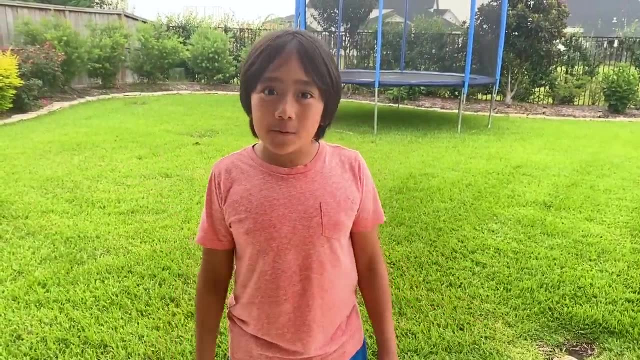 And remember, like Ryan, you should always wear sunscreen to protect your skin from the sun. That's right, Peck. Remember to do your part to help heal the ozone layer. That's all for today. Bye. Remember, always stay happy and rise up. Bye. 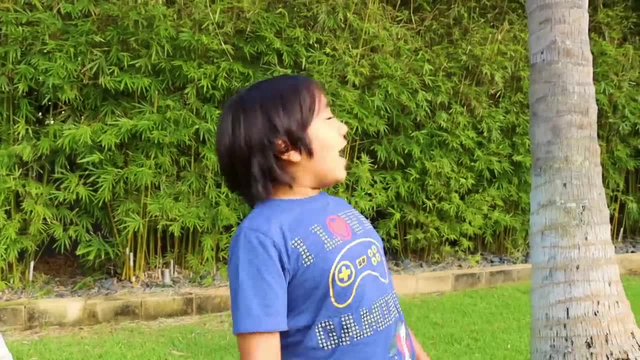 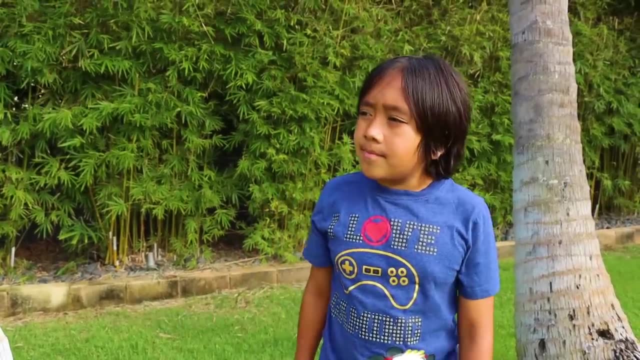 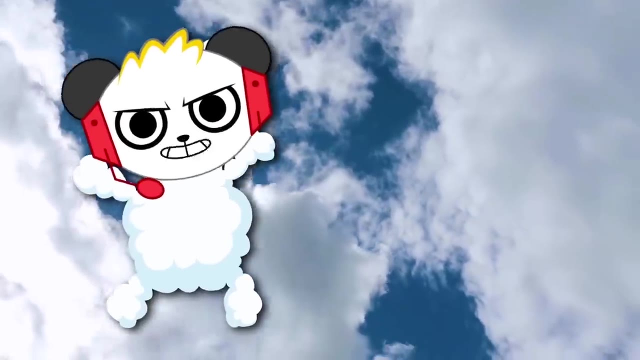 I'm going to go play now. Whoa guys, Check out the clouds today. I wonder where the clouds come from. That one's shaped like a panda, like Combo Combo Bunga, And that one looks like Peck. 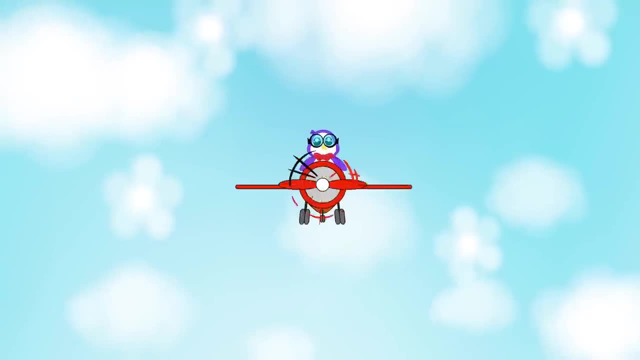 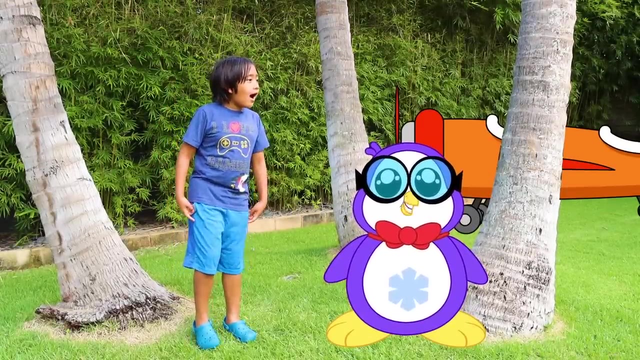 Wait a minute, It is Peck. Hey Ryan. Oh, hey Peck. What are you up to today? I've been learning all about the water cycle. I heard you wanted to know where clouds come from right. I heard you wanted to know where clouds come from right. 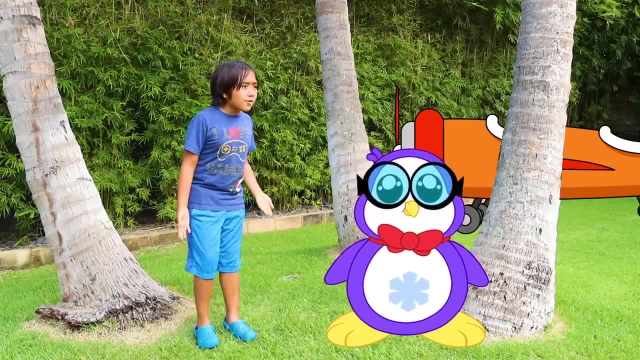 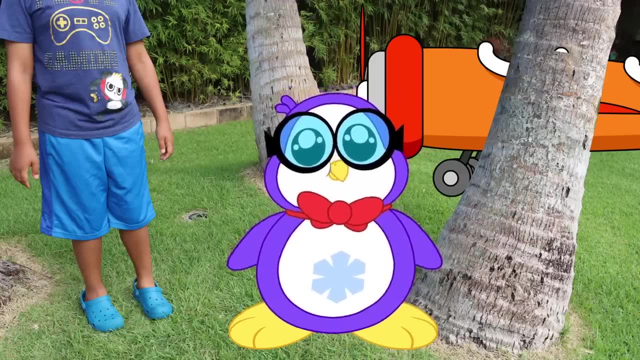 Wait, are you saying clouds are part of the water cycle? That's right. Can you teach me all about it? Of course, Leave it to me. Bye. Peck, Wait, where did Peck go? Peck, Hey, everybody. 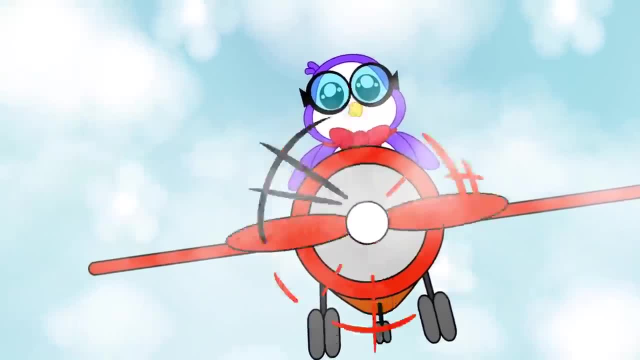 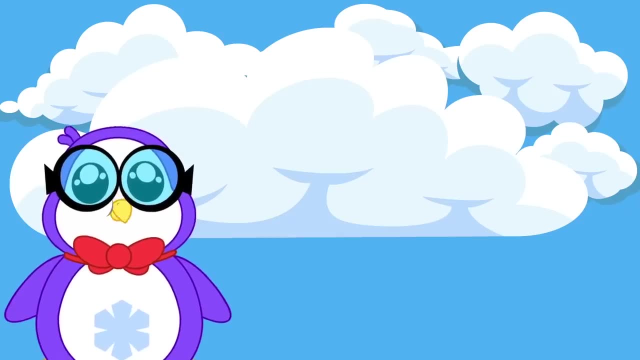 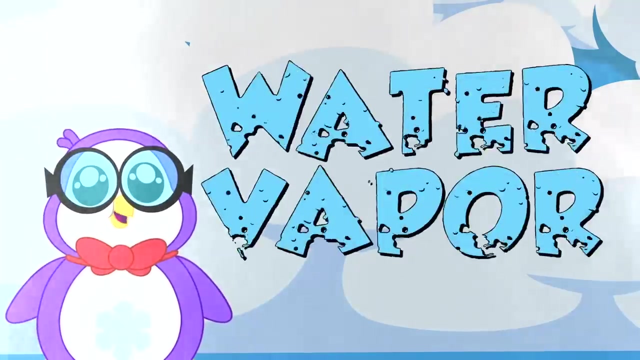 I've been flying through the clouds studying the water cycle. Let me show you what I've discovered. Condensation Clouds like this are made up of tiny water drops All around us. there's water in the air called water vapor. 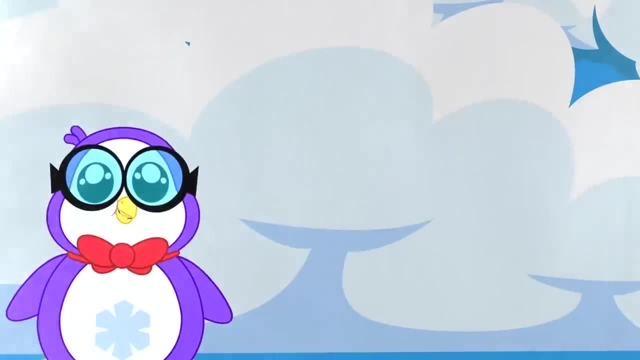 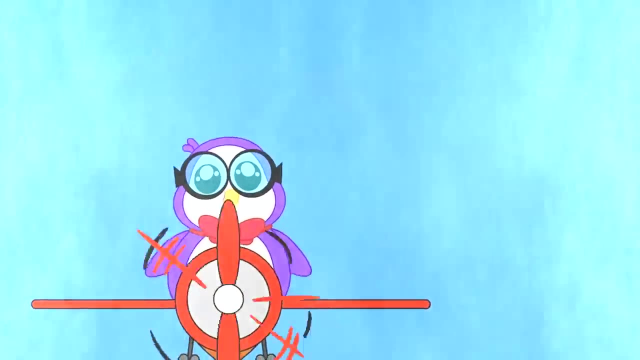 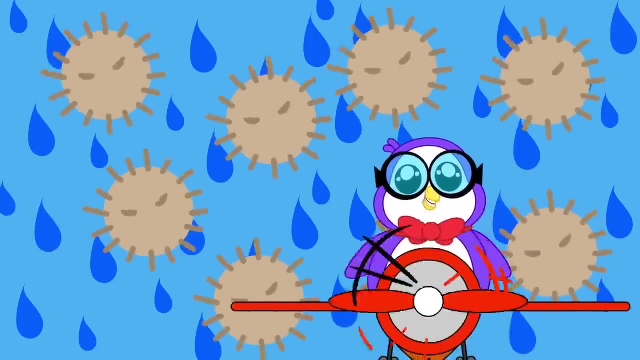 It's too small for us to see because it's in the gas form of water. When water vapor gets high in the sky, like when we are, the water vapor cools and condenses back into liquid water. This liquid water sticks to things in the air like dust. 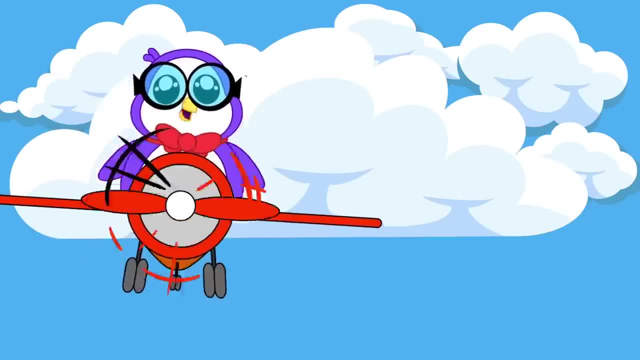 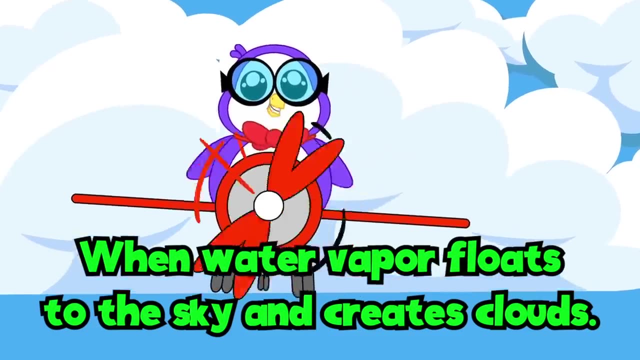 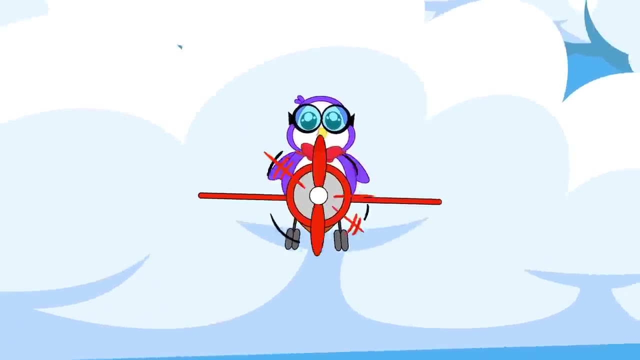 and this is how clouds form. This phase of the water cycle is called condensation. Look more. water is condensing and making the cloud grow. It's getting heavier, which means it's almost time for the next step of the water cycle. 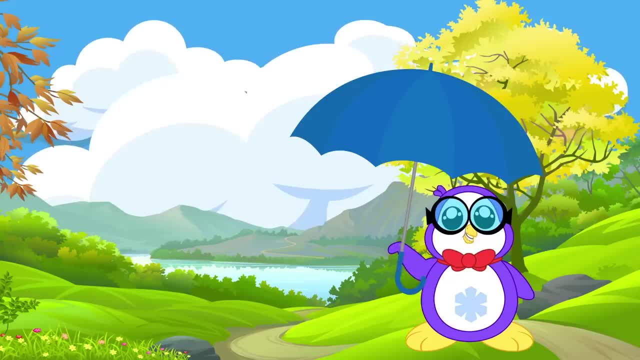 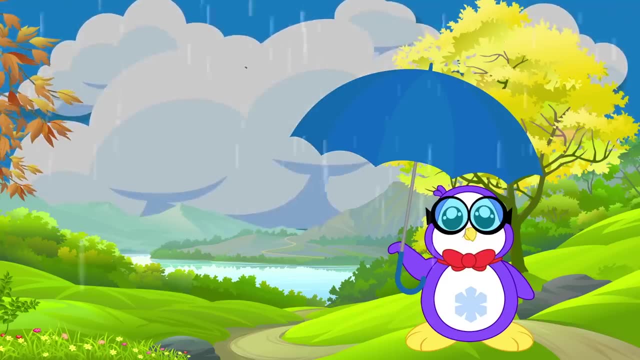 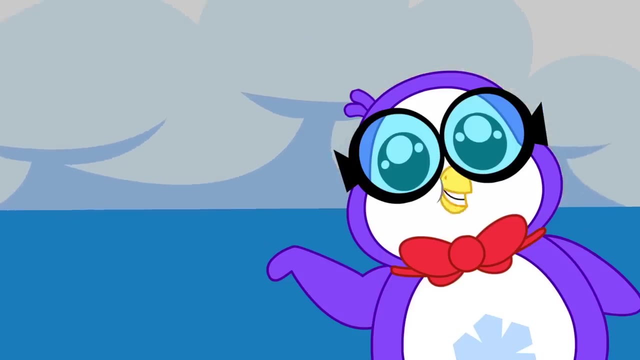 Precipitation. We're on the ground now and we're waiting for the next phase of the water cycle, which is precipitation. Eureka, See, When the clouds can't hold any more water. gravity can't hold any more water. 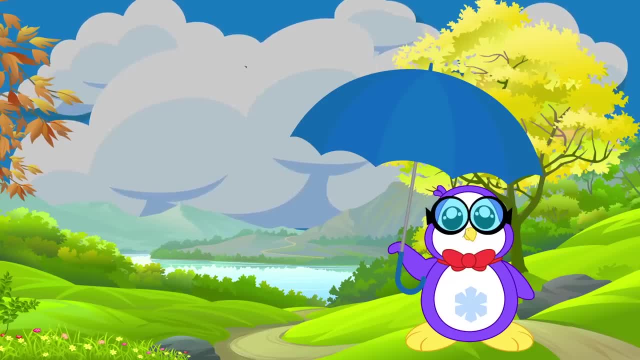 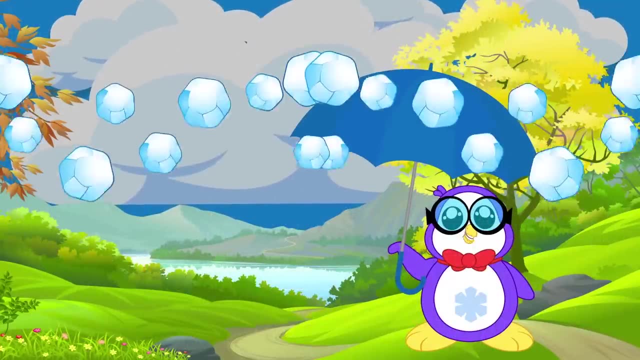 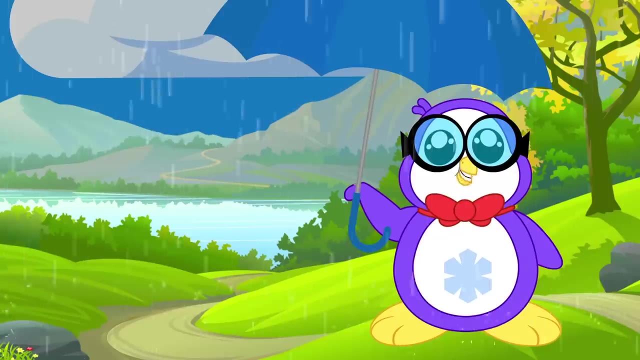 It makes the water fall back to Earth. This is called precipitation, And it can be in the form of rain, sleet, snow or even hail. Let's follow the path of where this water is going. It will surely lead us to the next phase of the water cycle. 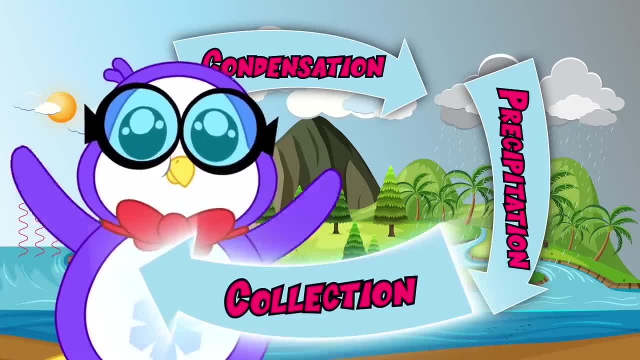 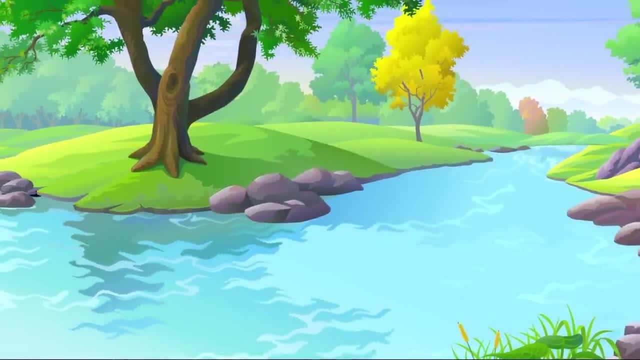 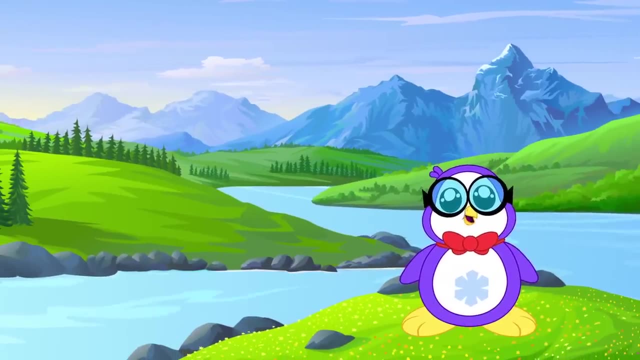 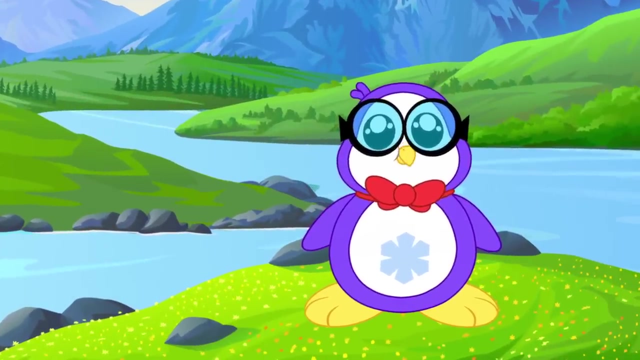 Let's go Collection. Ha ha, The rain stopped. Let's examine where it ended up. We followed the flow of water through a process called runoff, And all the water seems to collect in this area. This is the collection phase of the water cycle. 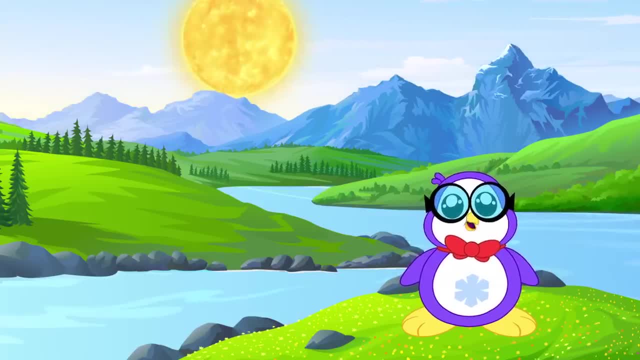 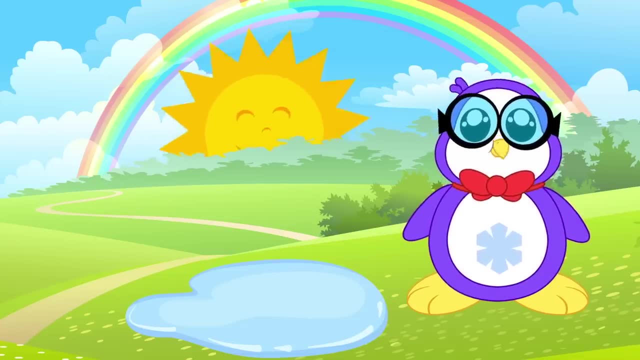 And here comes the sun. to complete the water cycle, Let's go Evaporation. I found the best way to show the final stage of the water cycle: A puddle. If we wait here long enough while the sun is out, we will be able to see this puddle disappear. 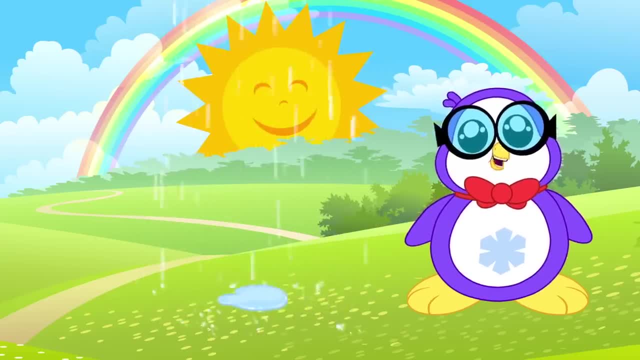 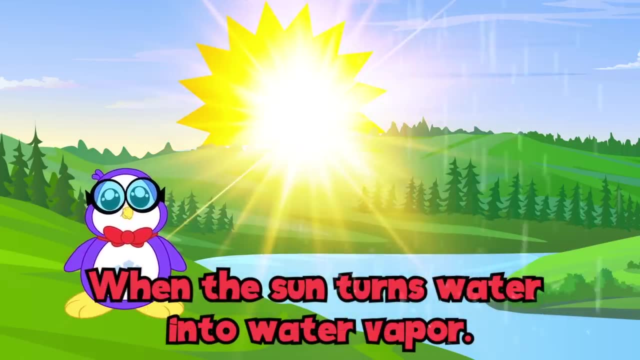 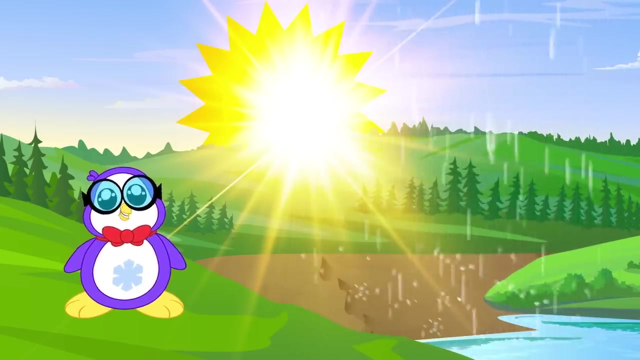 It will evaporate, which is the last stage of the water cycle for us to cover. Evaporation happens when the rays from the sun heat the liquid water and turn it into water vapor. At this stage, water goes from a liquid into a gas. 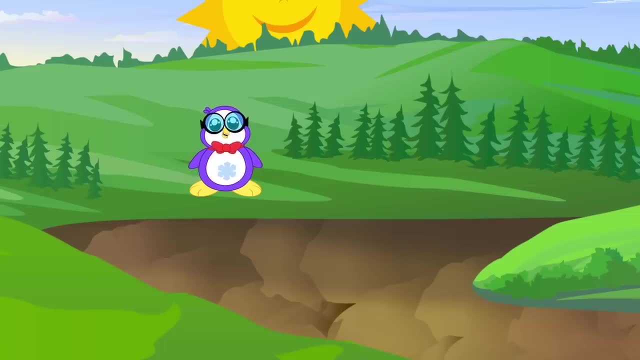 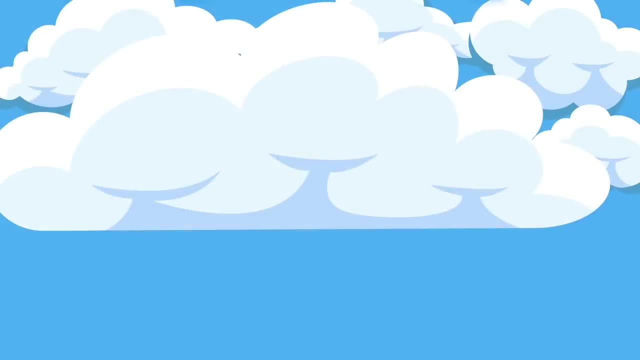 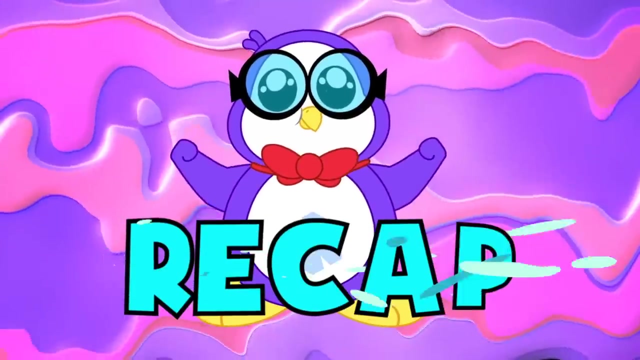 Oh boy, Look All the water evaporated. That means it's become a gas and it's rising into the atmosphere To become clouds again. And that's all for the water cycle Recap. Let's go over what we learned about the water cycle. 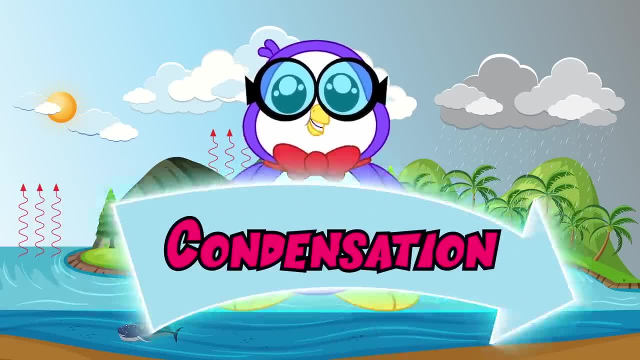 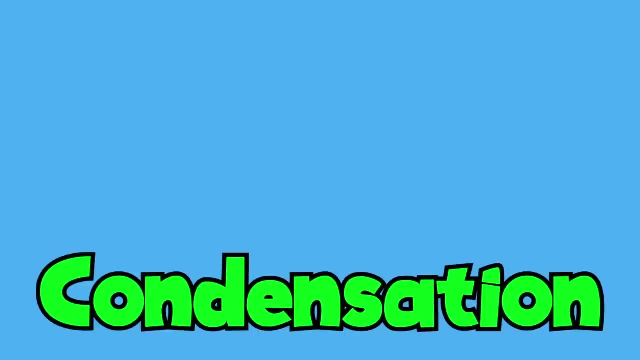 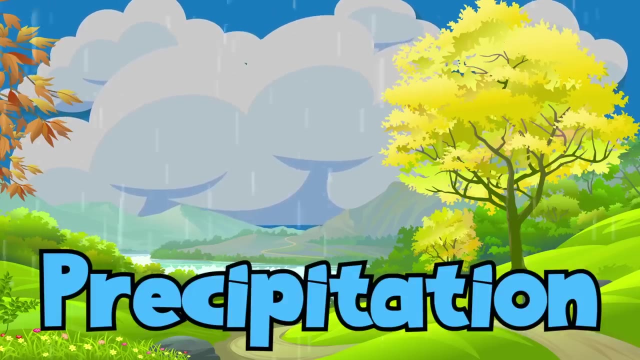 There are four stages of the water cycle: Condensation, Precipitation, Collection And evaporation. Condensation is when water vapor floats to the sky to create clouds. Precipitation is when water falls to the ground, as in rain, sleet, snow or hail. 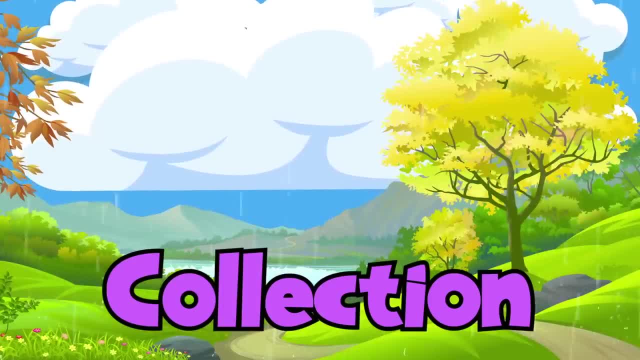 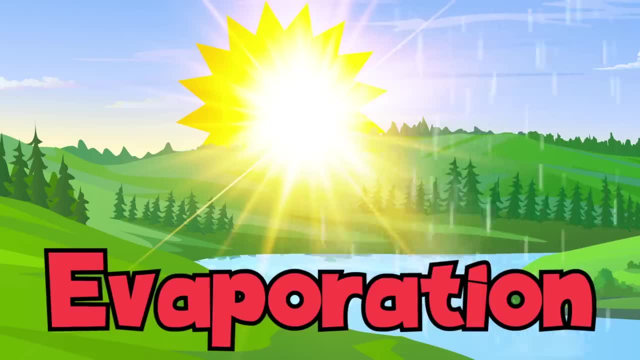 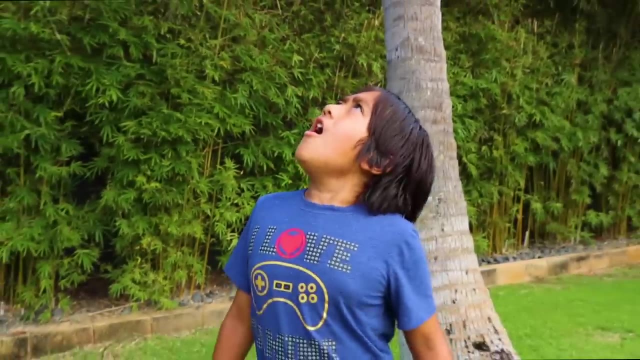 Collection is where water collects after it falls into the ground. It could be in rivers, lakes and even puddles. Evaporation is where the sun rays heat up water to become vapor and that vapor rises to the sky to become clouds. Wow. 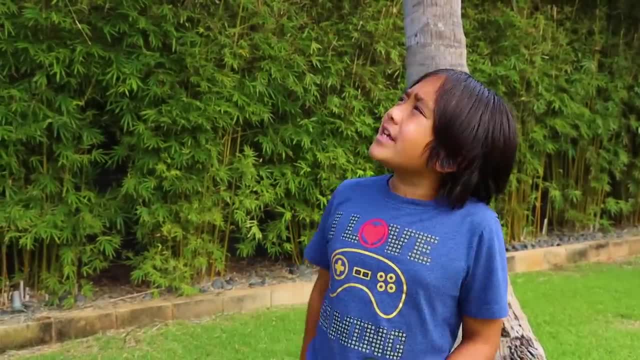 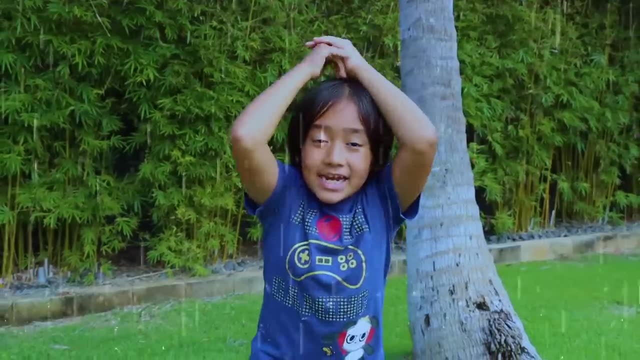 Thanks to Peck's water cycle research. I think all these clouds mean it's about to rain. Whoo, Whoo, I was right. I better get inside now. Bye, guys, Remember: always stay happy and bright, Bye. 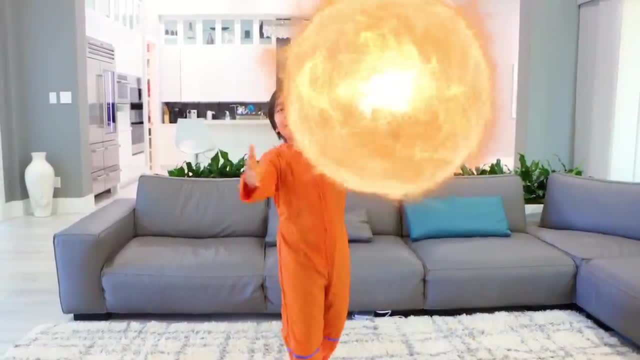 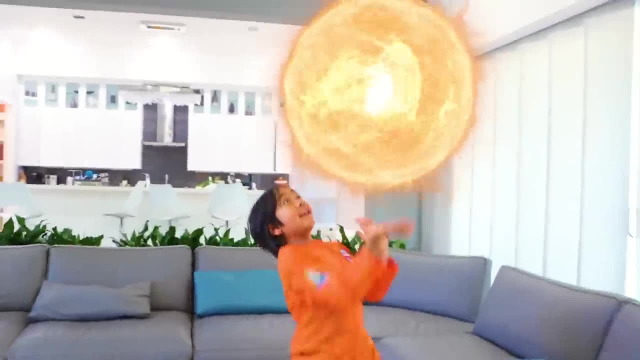 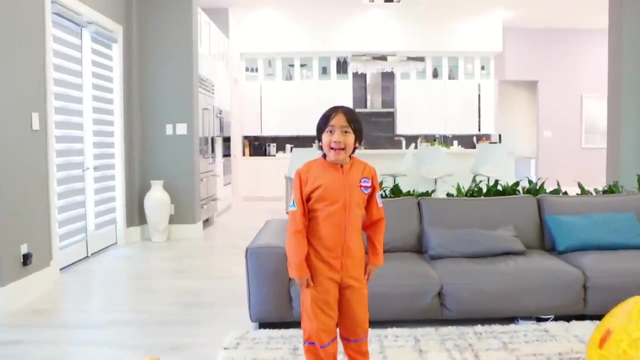 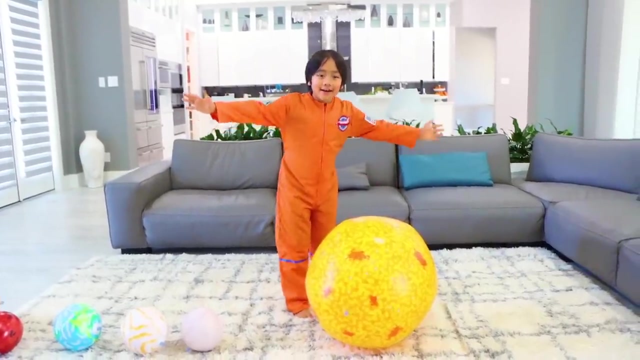 The sun is a yellow dwarf star that is in the center of our solar system. The sun is a super, duper, hot, giant ball of gas. Ha, Hey guys, astronaut Ryan here Let me teach you all about the planets. First, let's start off with the sun. 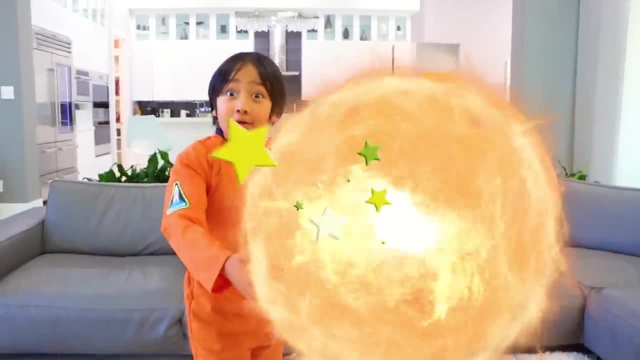 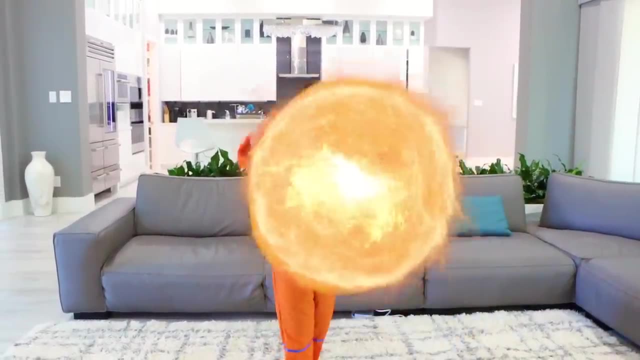 It's actually not a planet, it's a star. So all those stars you see are exactly like this. The sun is a yellow dwarf star that is in the center of our solar system. The sun is a super, duper, hot, giant ball of gas. 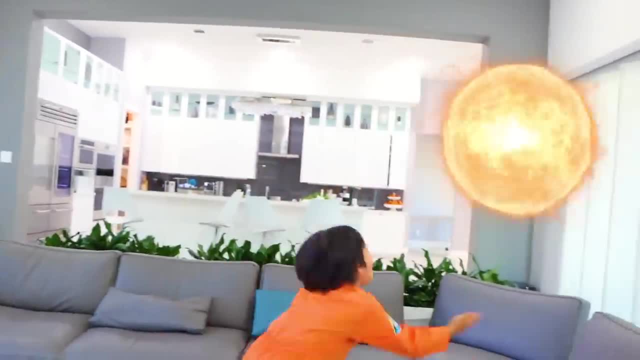 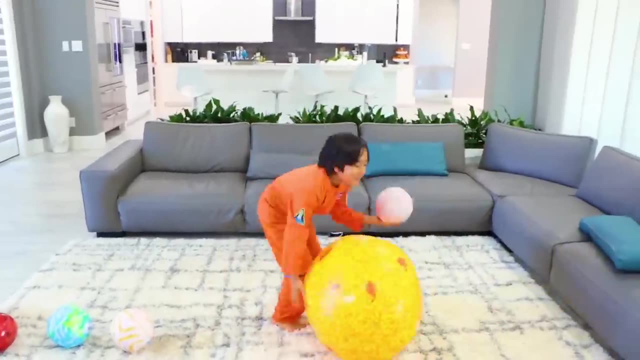 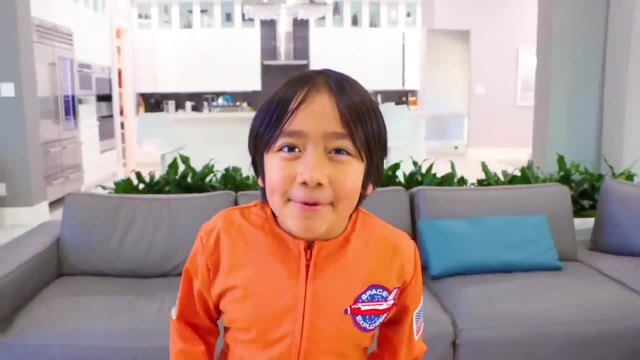 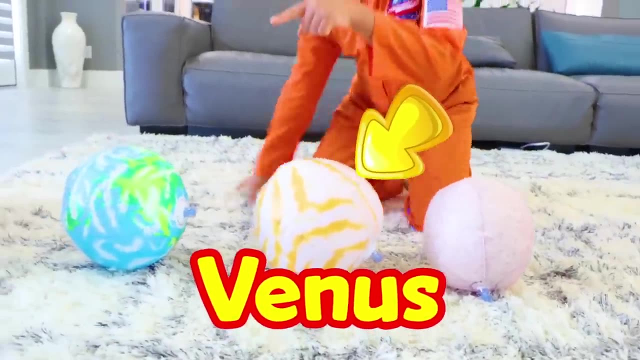 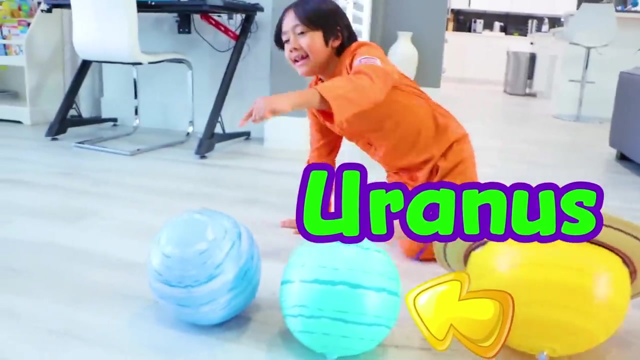 Do you know how many planets there are? There are eight planets in our solar system. Let's learn the names in order: Mercury, Venus, Earth, Mars, Jupiter, Saturn, Uranus and Neptune. Okay, so what is the order of the planets? again, 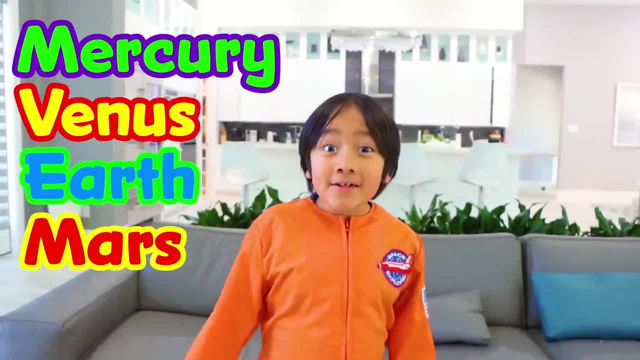 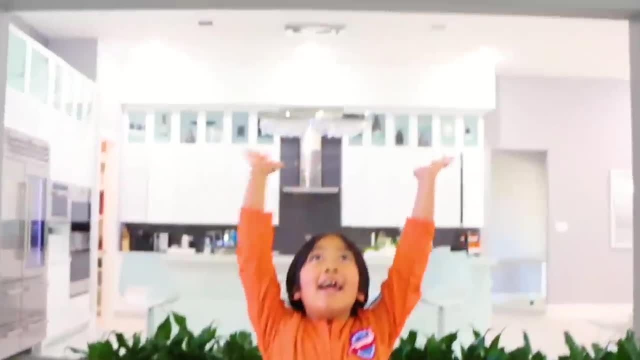 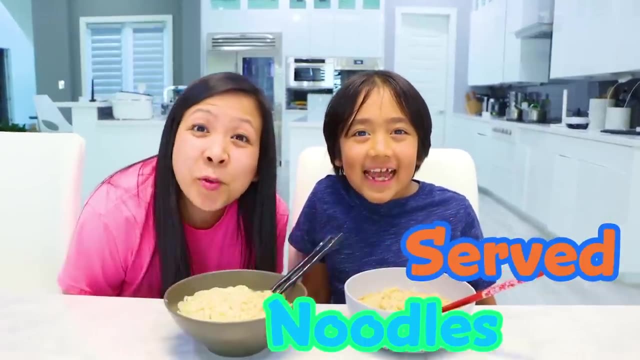 It's Mercury, Venus, Earth. Mercury, Mercury, Venus, Earth, Mars, Jupiter, Saturn, Uranus and Neptune. Here's a trick to remember the order: Whee, How do you remember the planets again? My very excellent mother just served us noodles. 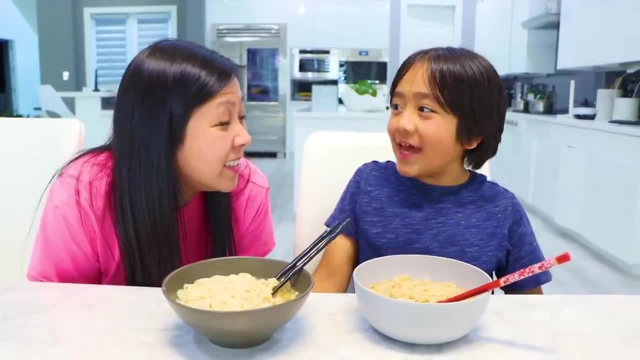 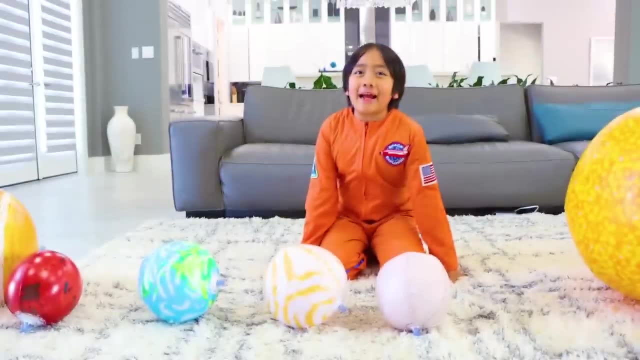 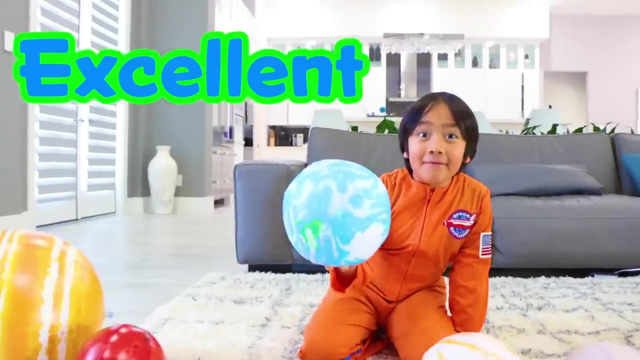 You ready to eat, Ryan? Yeah, after I learn about the planets, Okay, well, I'm not gonna wait for you. Hmm, So here's what each letter stands for: My Mercury, very for Venus. excellent for Earth. 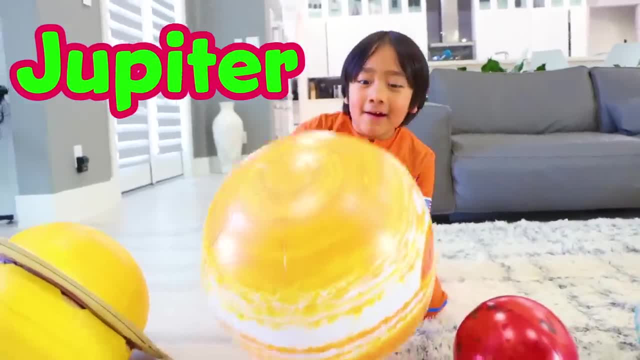 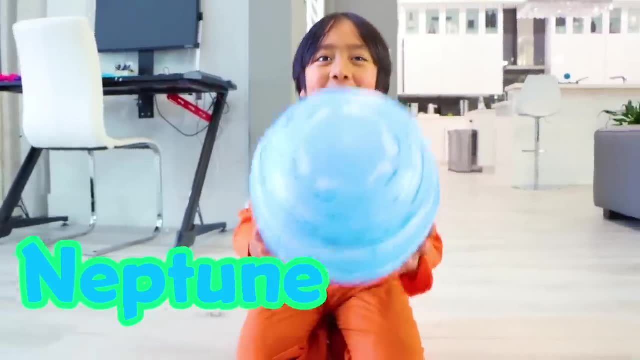 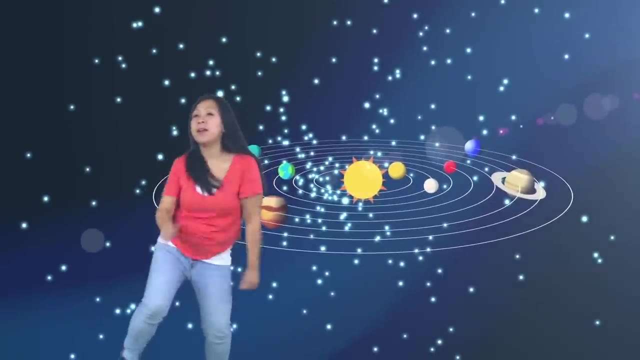 mother for Mars, just for Jupiter, served for Saturn, us for Uranus and noodles for Neptune. Here's also a very fun song to help learn the planets: Whee whee, whee, whee whee. This is the Planet Song. 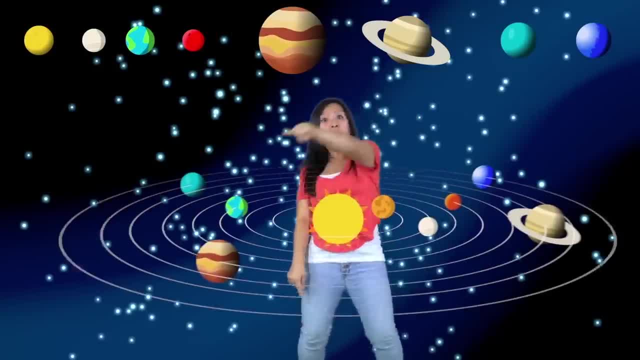 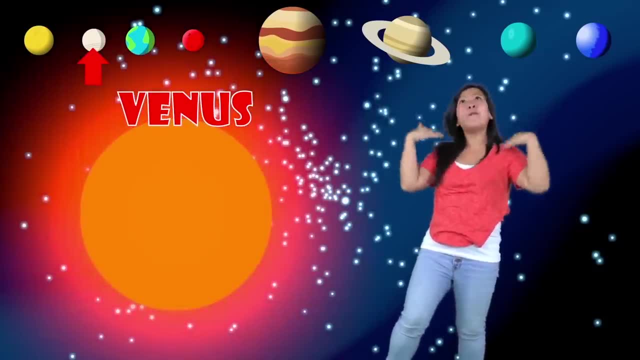 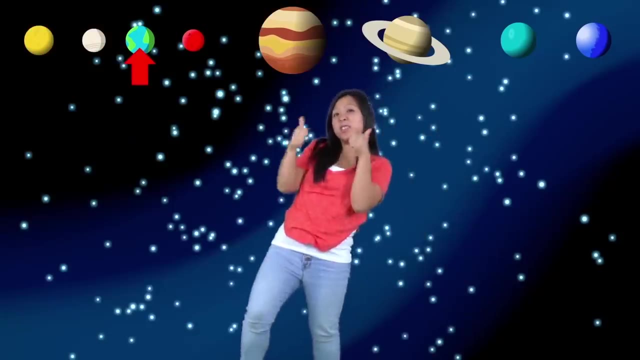 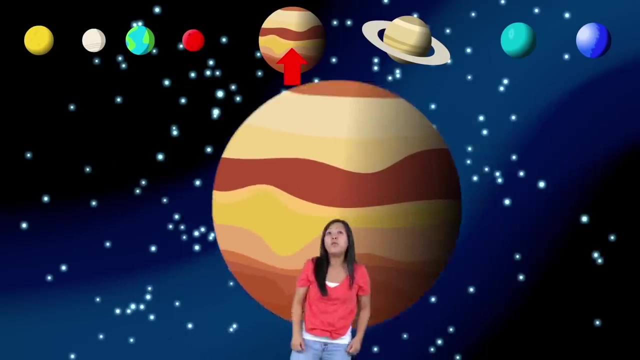 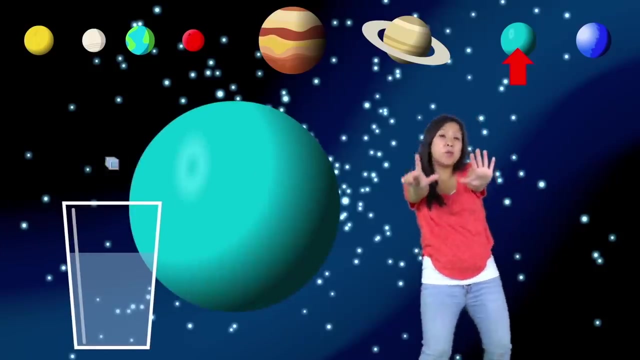 If you know the order, Sing along. Planets revolve around the sun. Mercury is number one. Venus is number two- It's too hot for me and you. Earth is the place to be. It's planet number three. Now let's learn some more. Mars is red and it's number four. Jupiter is number five And it's known for its giant size. Saturn is the one with rings: It's number six in the order of things. Seven is the planet with ice: It's Uranus, and it's been on its side. 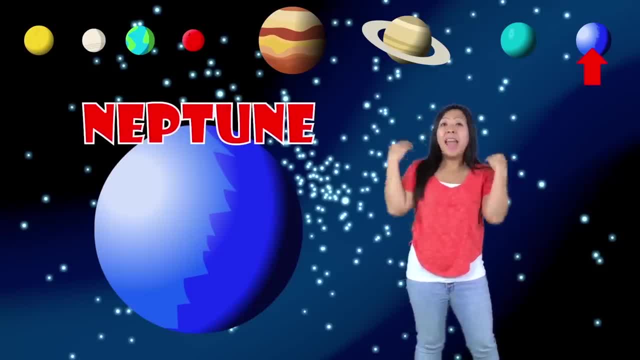 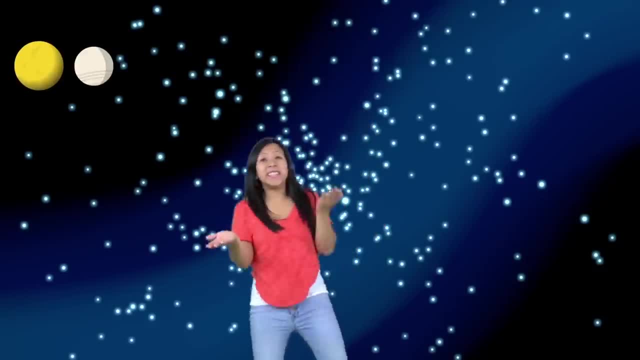 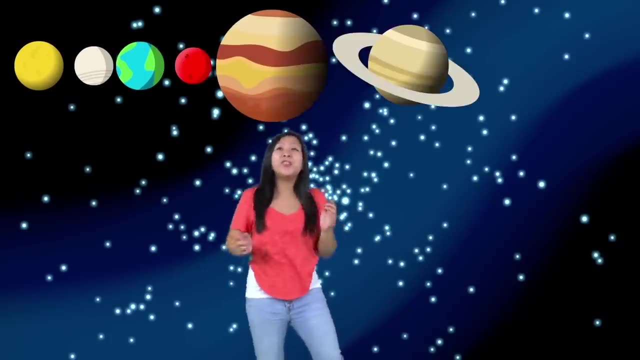 Number eight's called Neptune, It's the last one and it's blue. This is the planet song. Now you know the order. Sing along: Mercury, Venus, Earth, Mars, Jupiter, Saturn, Uranus and Neptune. Mercury, Venus, Earth, Mars, Jupiter, Saturn, Uranus and Neptune. 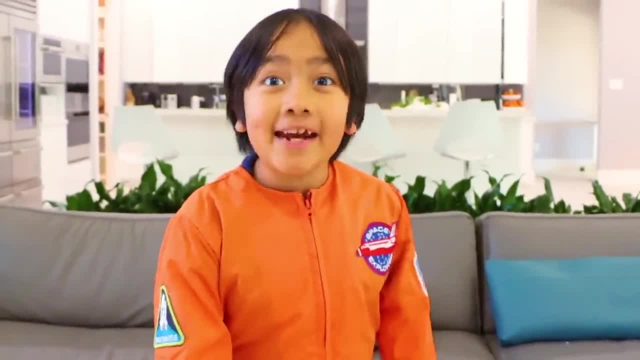 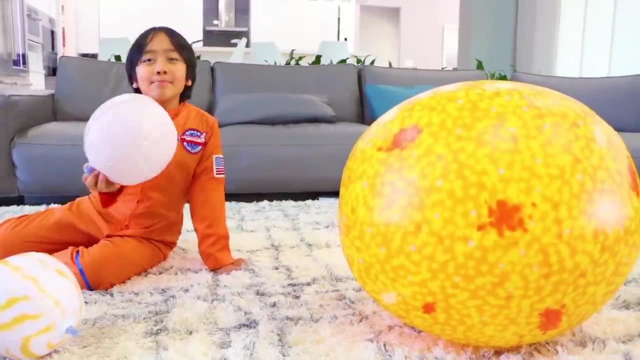 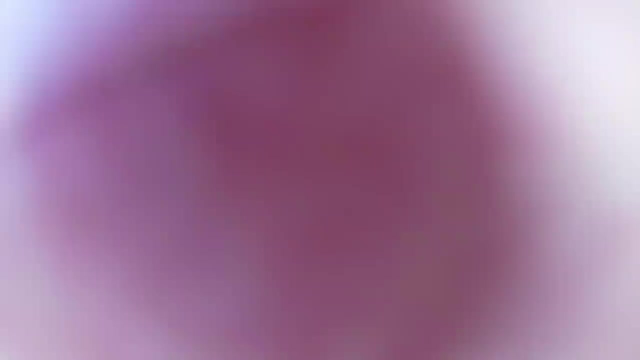 Ready to learn some fun facts about each planet with me, Let's do it. The first planet that is also the closest to the sun is Mercury, And it's also the smallest planet. I'll have Peck tell you more about Mercury. Thanks, Ryan. 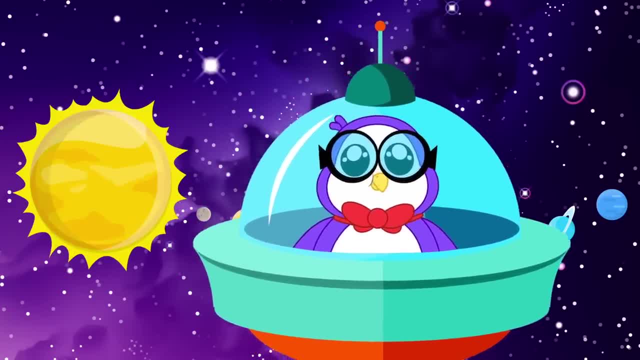 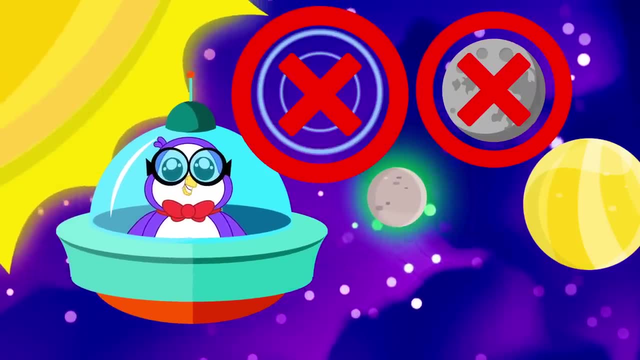 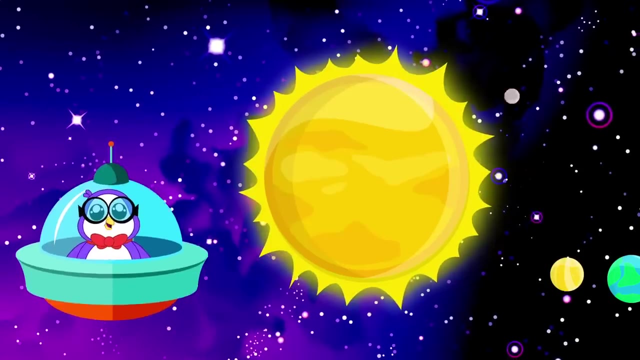 I'm so excited to share some facts about the planets. Let's start with Mercury. Mercury is the smallest planet. It does not have any moons or rings. Even though Mercury is the closest planet to the sun, it's only the second hottest planet. An entire year of Mercury takes only 88 Earth days. 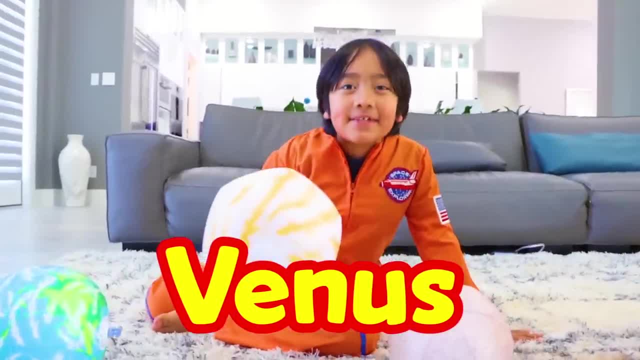 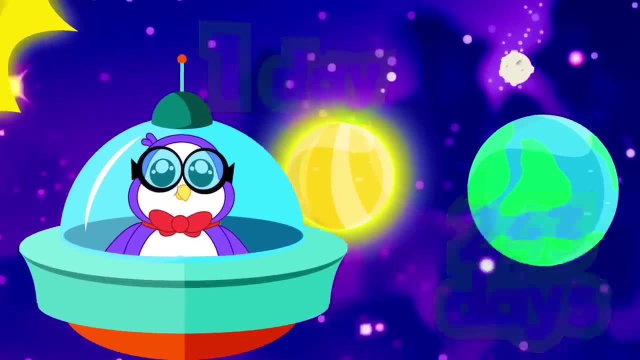 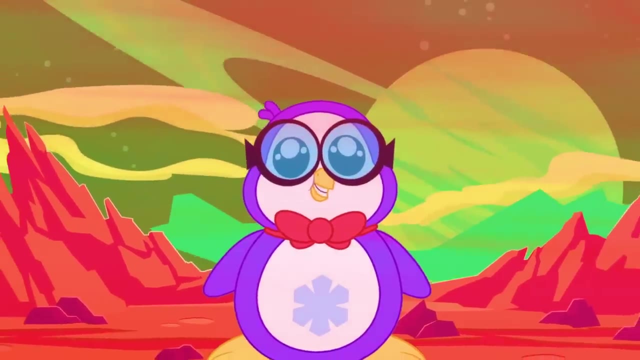 The second planet is Venus. Peck, tell us more about Venus. Did you know one day on Venus lasts 240 days? Did you know one day on Venus lasts 240 days? Venus is the second brightest object in the night sky. Only the moon is brighter Because of its harsh atmosphere. Venus is the hottest planet in the solar system. 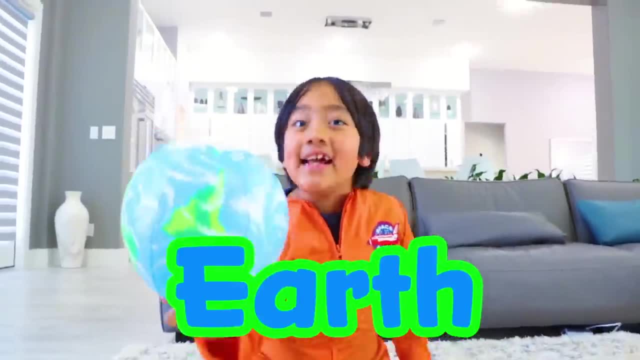 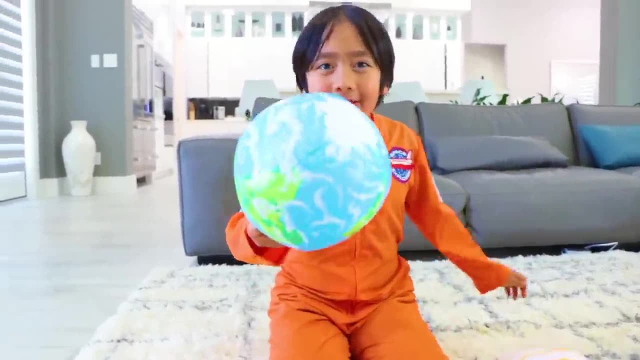 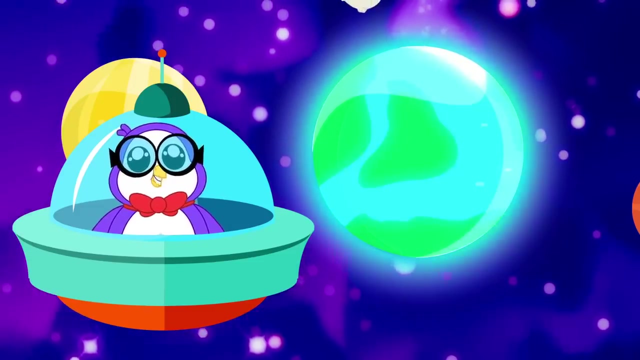 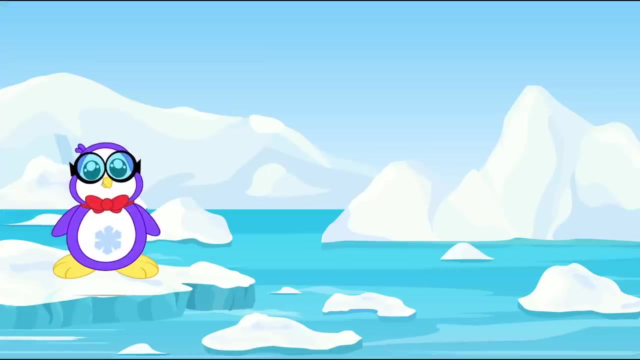 The third planet from the sun is Earth. It's also my favorite because we live here. Okay, Peck, it's your turn to tell us some fun facts about Earth. Earth is the only known planet to support life. 71% of the Earth's surface is covered in wine, Although 3% is fresh water and 2% is frozen in ice sheets and icebergs. 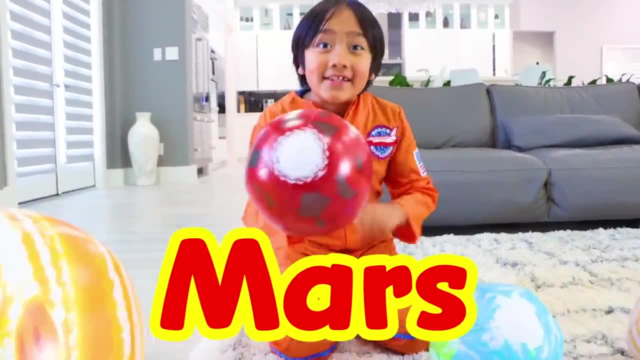 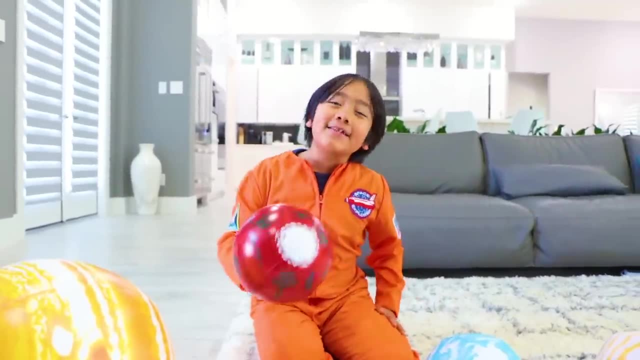 Next up planet is Mars. It's also sometimes called the red planet because it looks red from Earth. Okay, Peck, now tell us some fun facts. Mars is known as the red planet due to its reddish appearance. Mars is known as the red planet due to its reddish appearance. 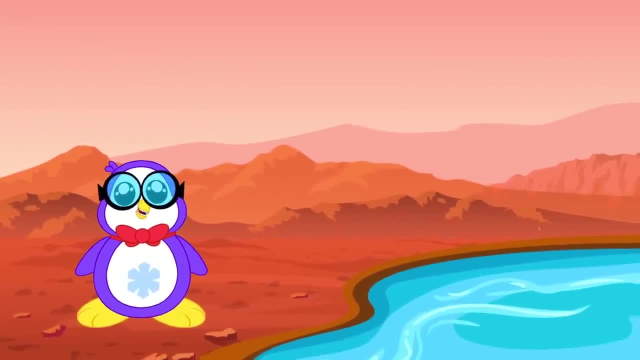 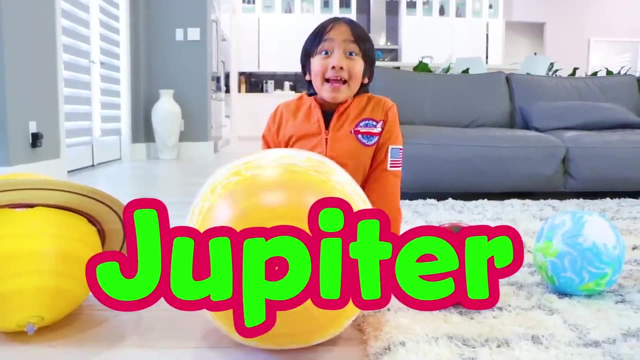 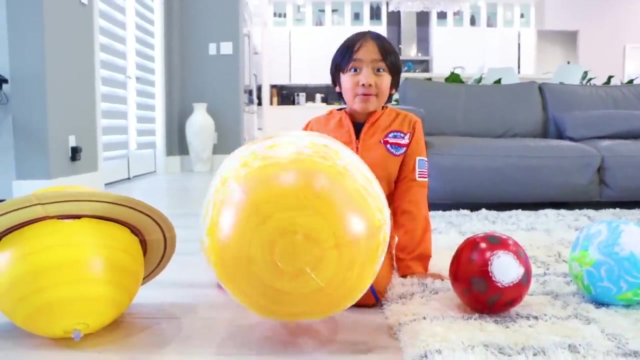 Unlike other planets, there are signs of liquid water on Mars, which means maybe it could one day support life. The fifth planet from the sun is Jupiter. It's also the largest planet in our solar system. Okay, Peck, can you tell us some fun facts about Jupiter? 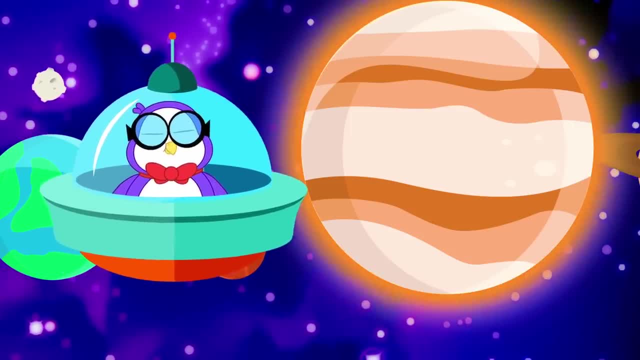 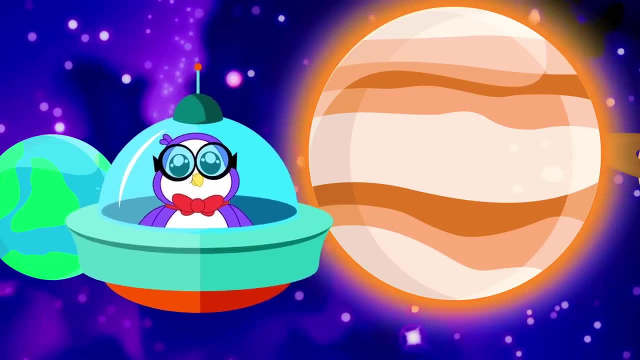 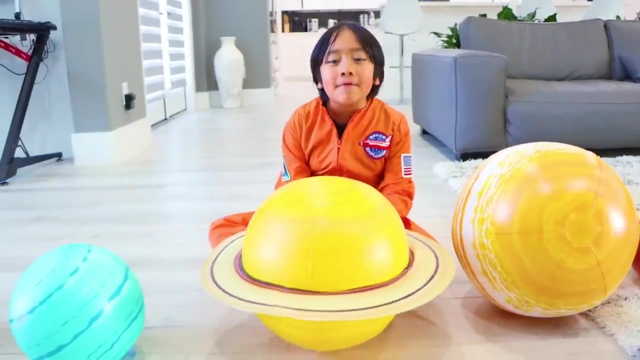 Jupiter is the largest planet in the solar system, Whoa. It's primarily made up of gas and is therefore known as the gas giant. The Great Red Spot is a huge storm on Jupiter that is the size of three Earths. This is the sixth planet from the sun. It's Saturn. And you see these rings? They're actually made out of millions of ice chunks. 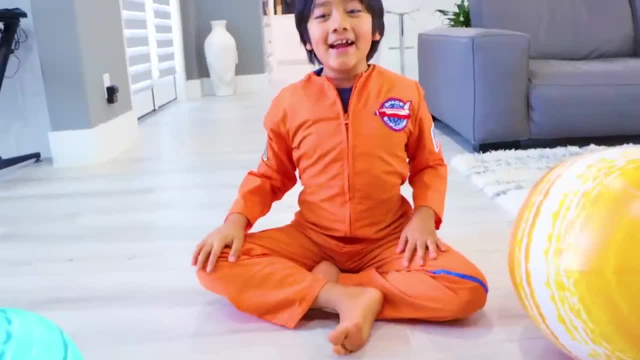 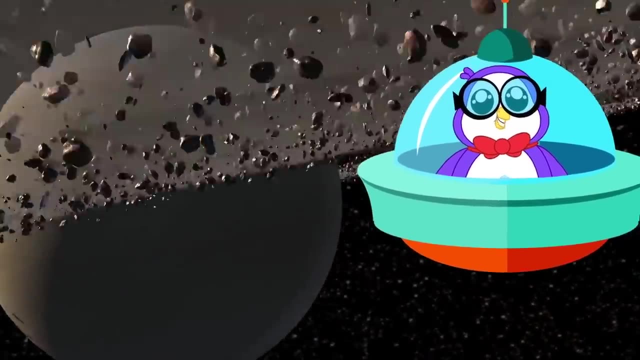 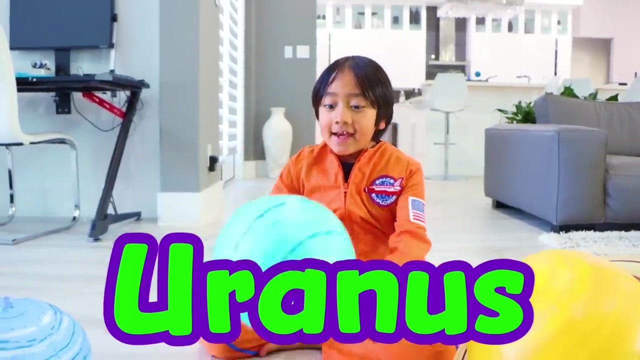 Okay, fun facts with Peck Whee. Saturn is another gas giant. It has the most extensive rings that are made up of ice chunks and dust. Saturn has 82 moons. The seventh planet from the sun is Uranus, And it appears to spin on its side. 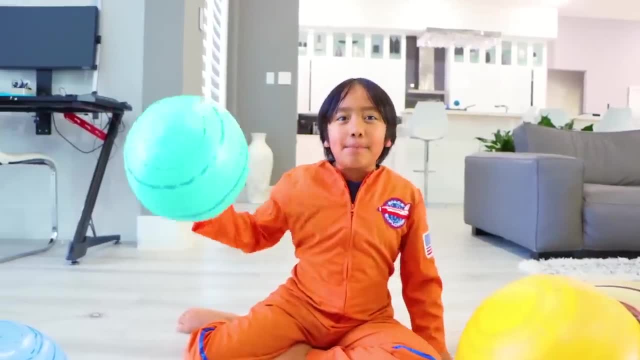 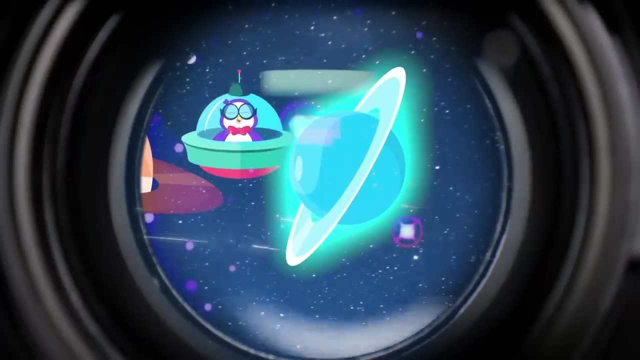 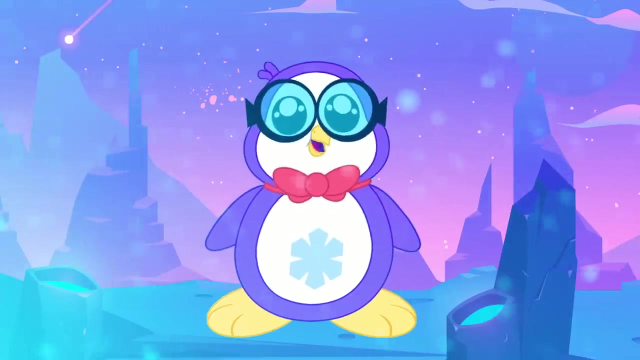 And Peck will tell you some more fun facts about Uranus. Uranus is not visible to the naked eye and is the first planet discovered by the use of a telescope. It is referred to as an ice giant planet. Although it's not frozen, the atmosphere is filled with ice crystals. 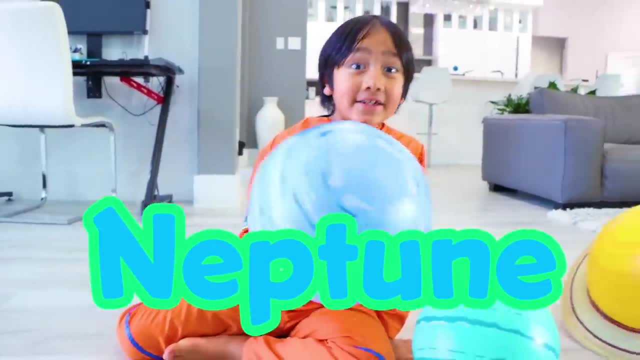 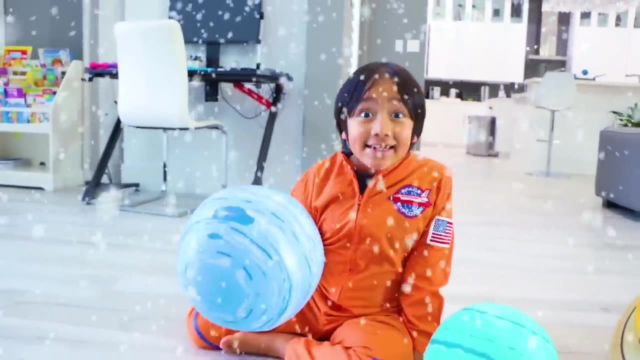 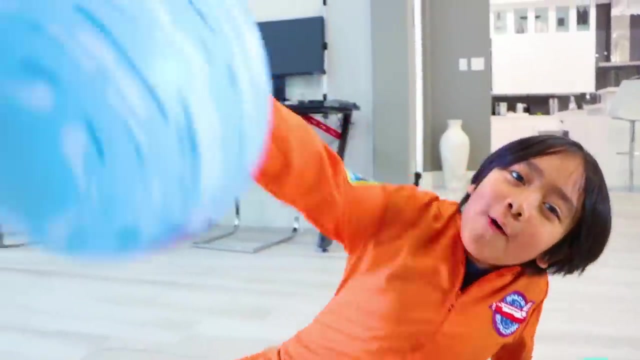 The eighth planet from the sun is Neptune And since it's so far away from the sun, it is super dark and cold here And it rains diamonds Cha-ching. Okay, and Peck will tell you some more fun facts about Neptune. 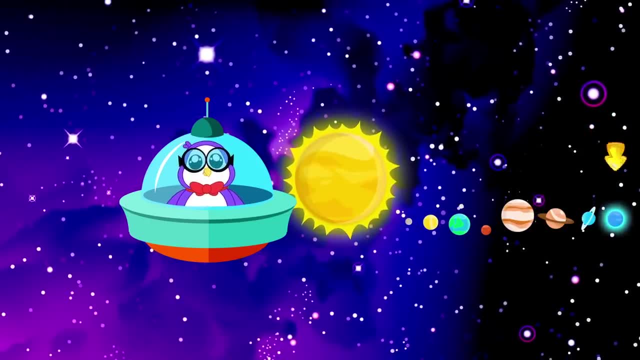 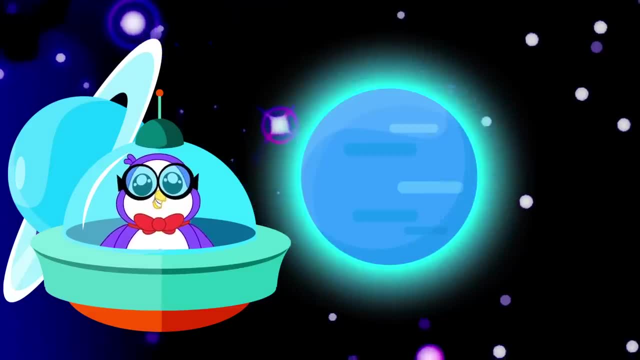 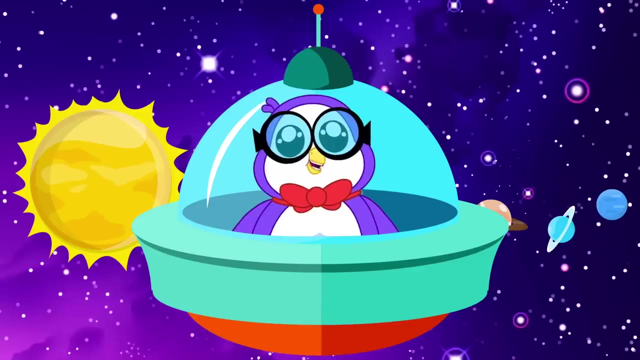 Neptune is the most distant planet from the sun. A year on Neptune lasts longer than 165 years on Earth. All the methane in Neptune's atmosphere gives it its blue color. Wow, Learning about the planets was fun, Ryan. See you later. 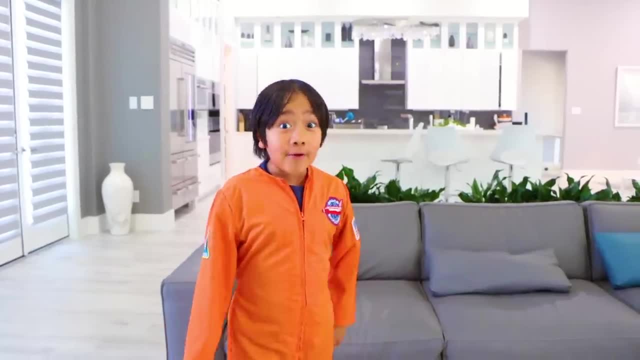 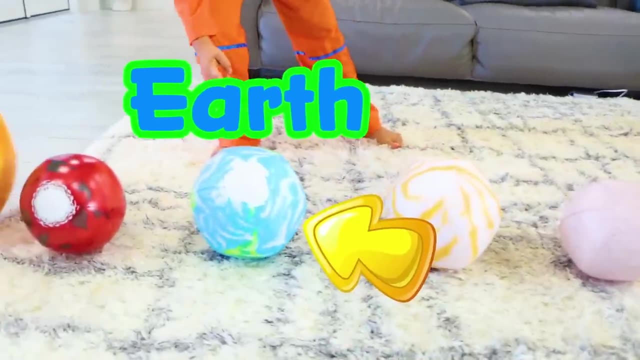 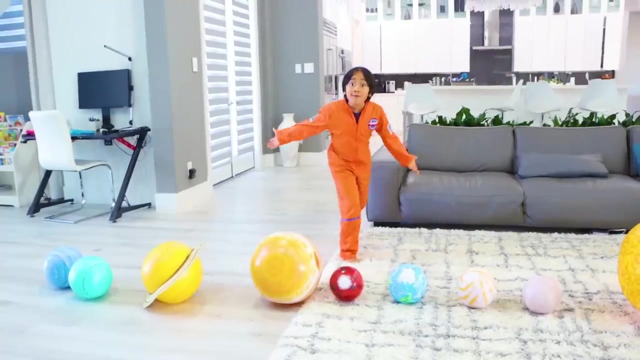 Recap time. How many planets are there in the solar system? There are eight. It is Mercury, Venus, Earth, Mars, Jupiter, Saturn, Uranus and Neptune. All of these planets orbit or go around the sun like this Whee. 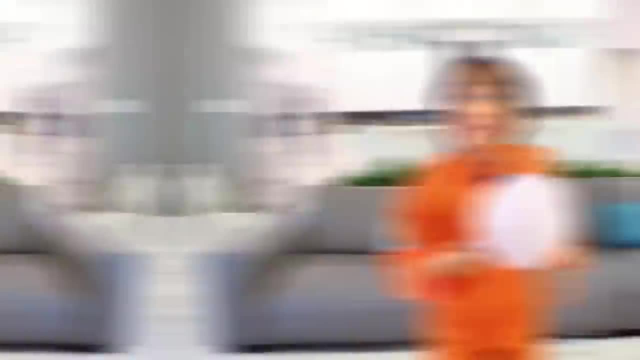 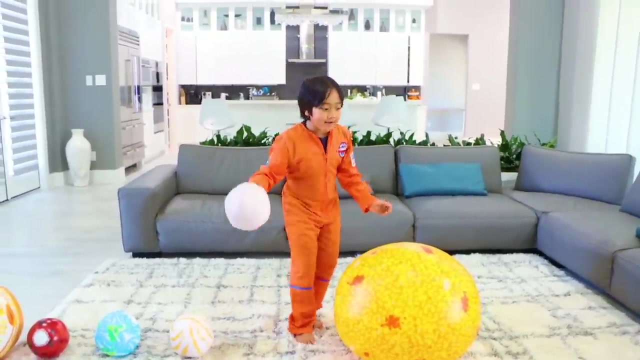 That's one year 365 days. Some planets orbit the sun super fast, like Mercury, It only takes 88 days, since it's the closest Whee Already there. Some planets take a very long time to orbit the sun, like Neptune. 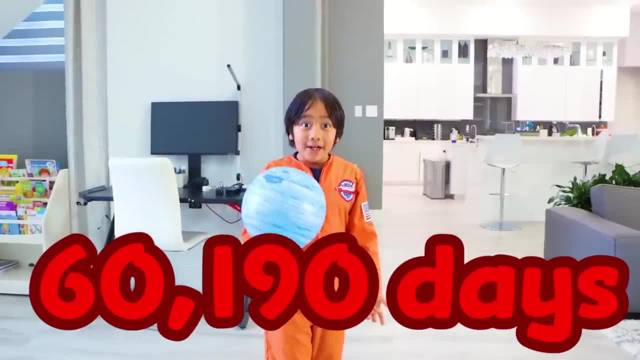 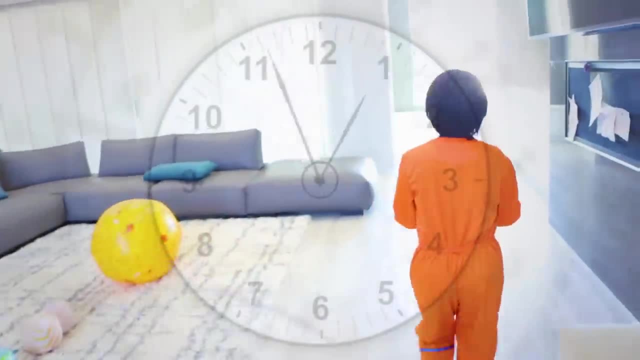 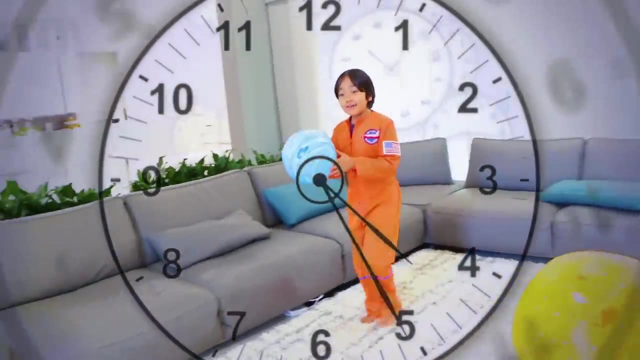 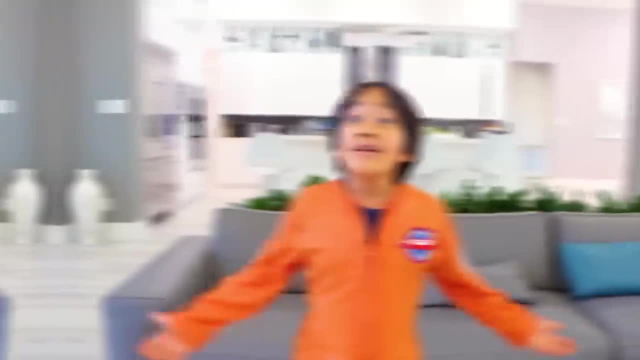 It's Mercury, Venus, Earth, Mars, Jupiter, Saturn, Uranus and Neptune. My very excellent mom just served us noodles. Okay, guys, thank you for learning all about the planets with me. Remember: always stay happy and bright, Bye. 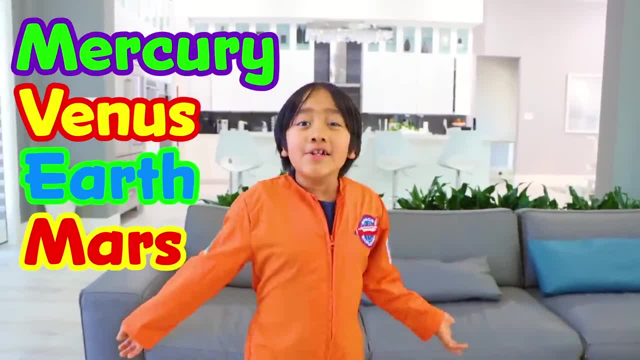 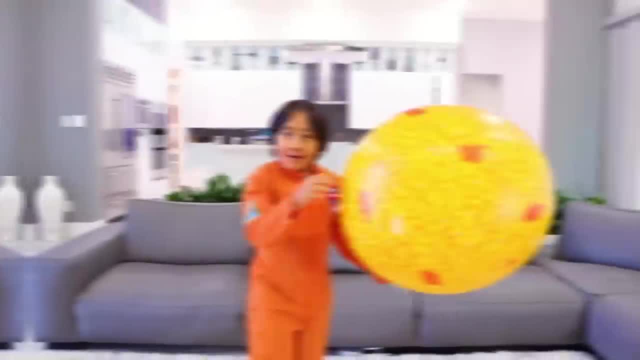 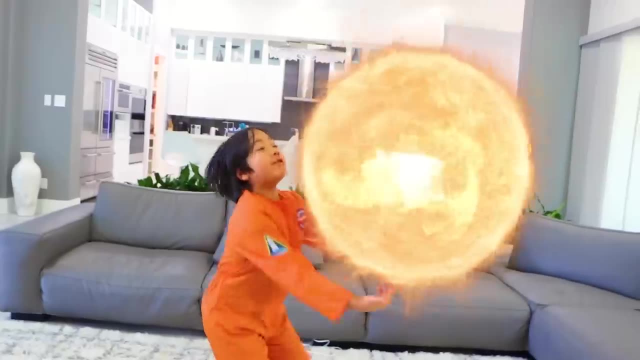 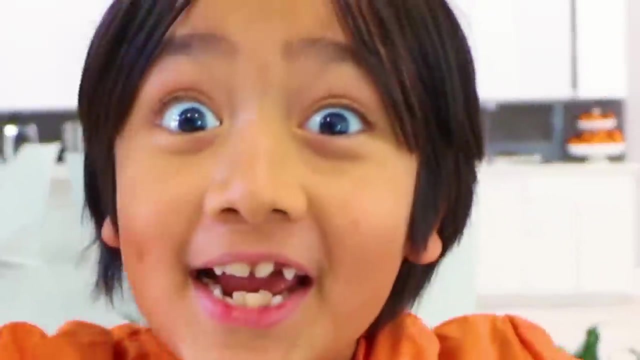 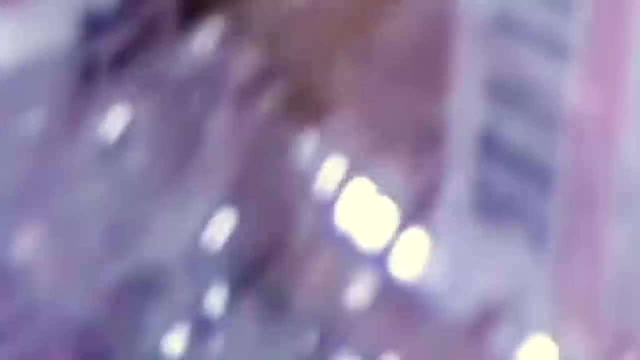 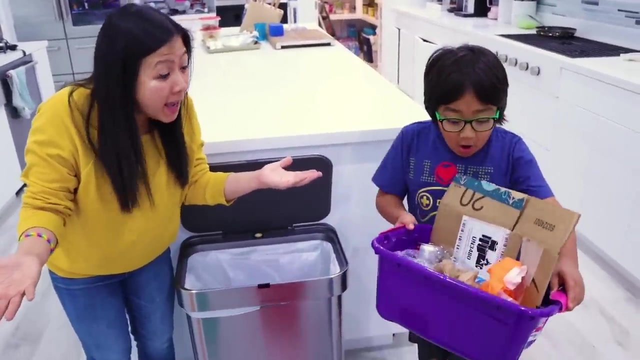 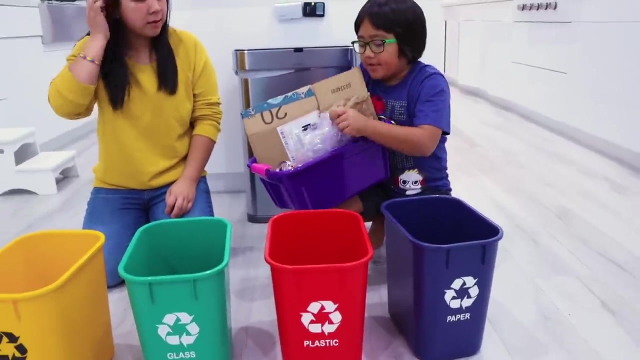 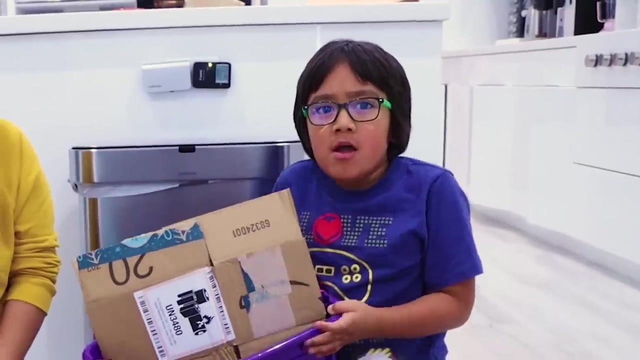 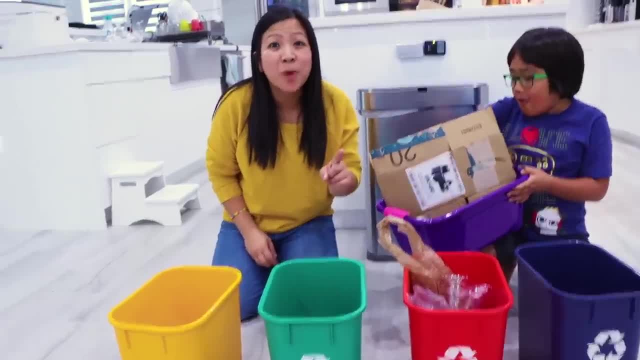 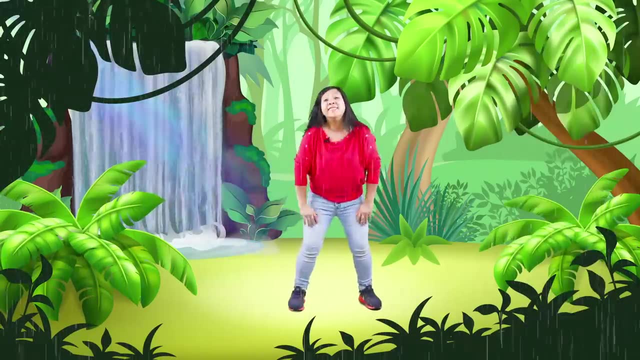 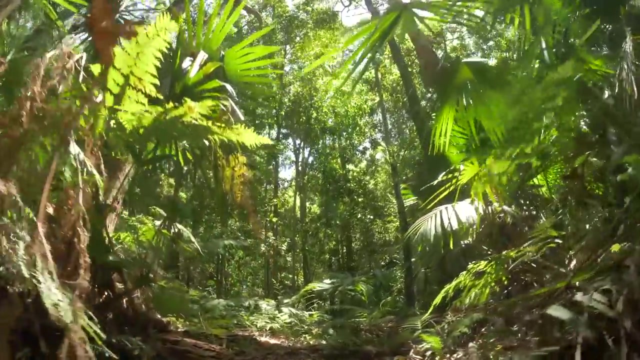 Well, mommy, I know it's good to recycle, but what other things can we do to save our planet? Good idea, Ryan, I'll show you. I'll be right back, you guys. Huh, Did you know? wild rainforests are tall, dense jungles with half of the world's plants and 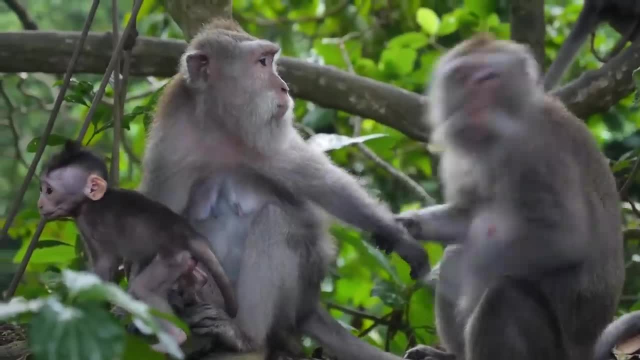 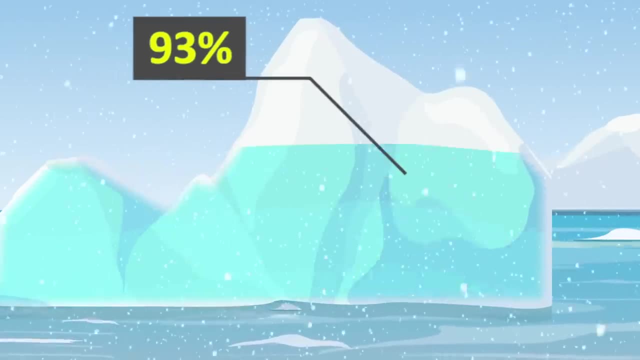 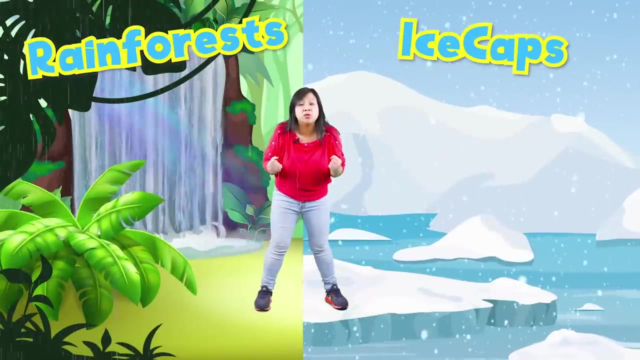 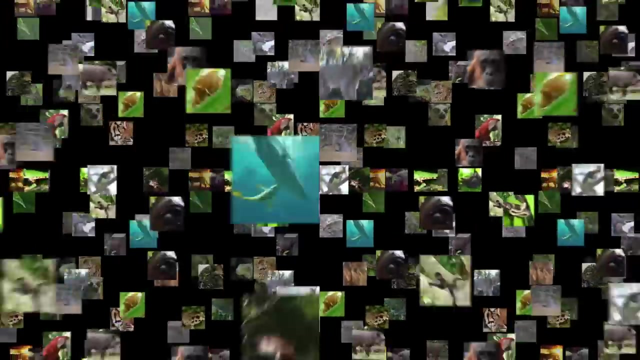 animal, And most of them are bows. Really, ice caps are huge glaciers of ice that holds 93 percent of fresh water here on earth. wild rainforests and ice caps are essential to planet earth and they're in big, big trouble. there are over 30 million species of plants and animals in the wild rainforest. 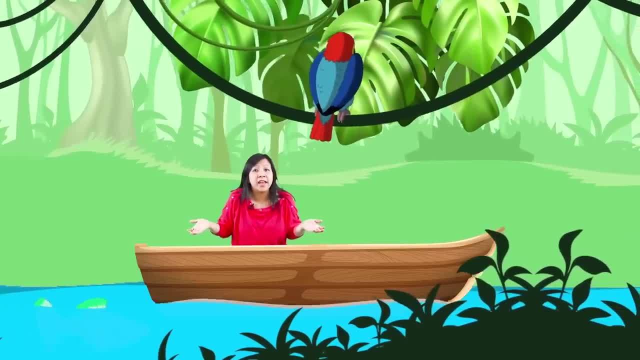 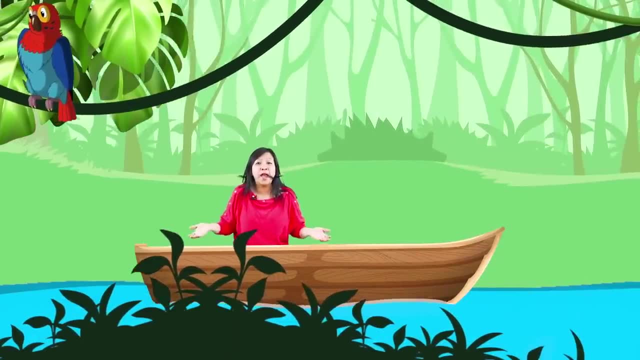 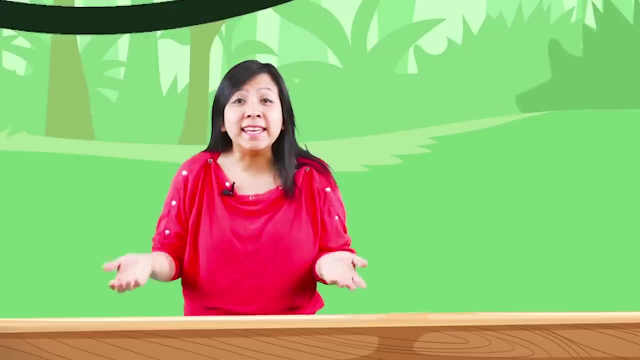 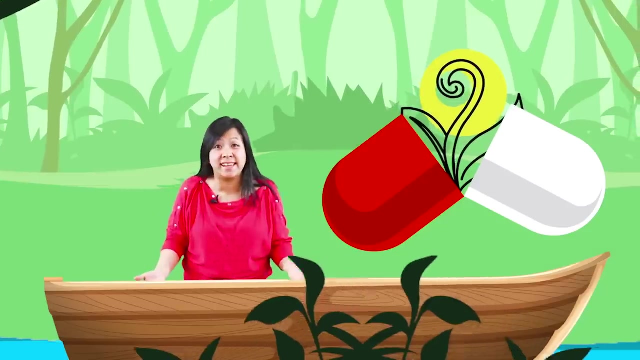 oh yay, we're in the rainforest and look, there are animals like fish and birds and orangutans that help spread pollens all around the rainforest so that pollen can produce all kinds of plants, and these rainforests have 70 percent of the plants that we use in medicine. 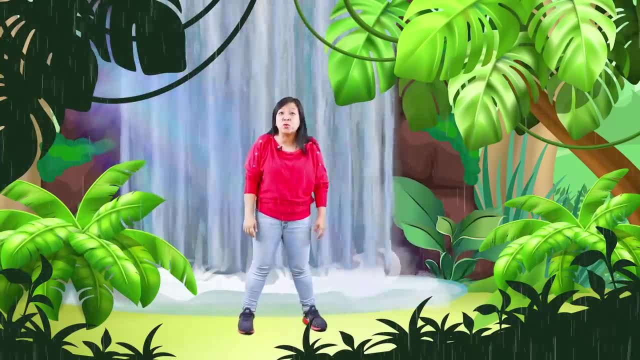 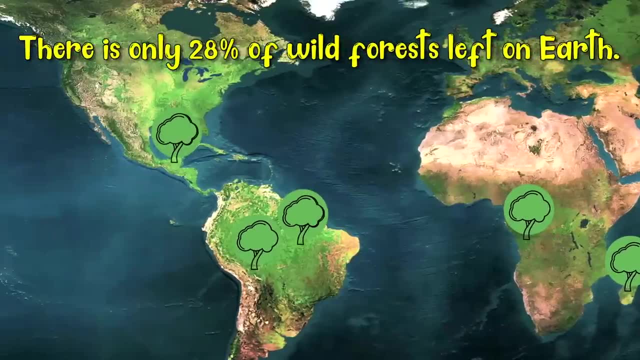 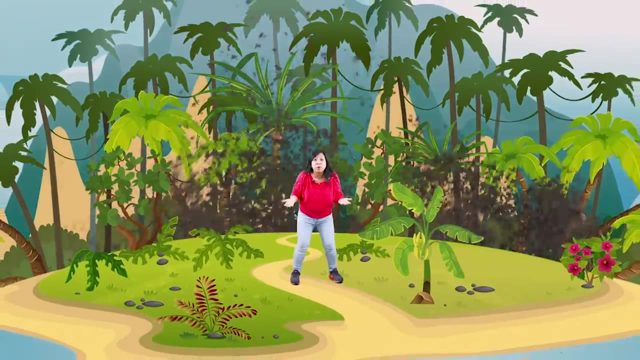 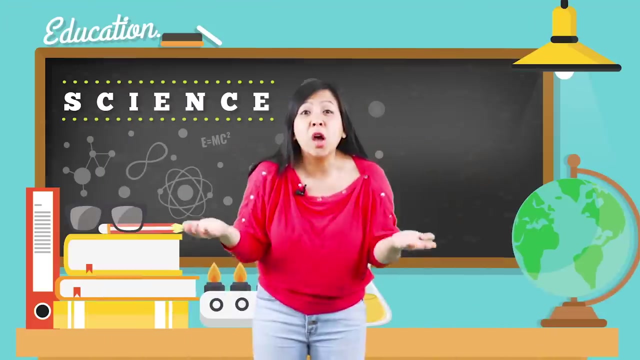 that's a lot of really important reasons why we need the rainforest. but did you know there are only 28 percent of wild forests left globally right now. so if we don't help out, the rainforest might disappear. bye-bye rainforest. no, we don't want that right. so what will happen if we let the rainforest disappear? 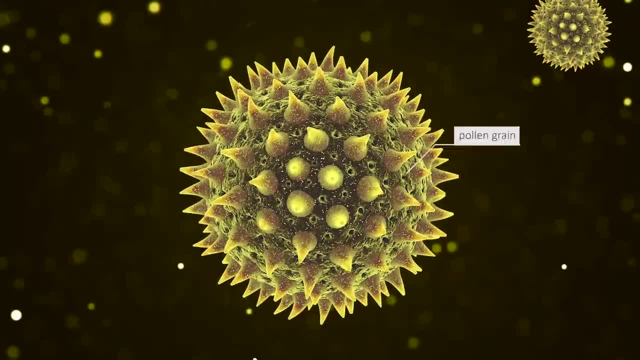 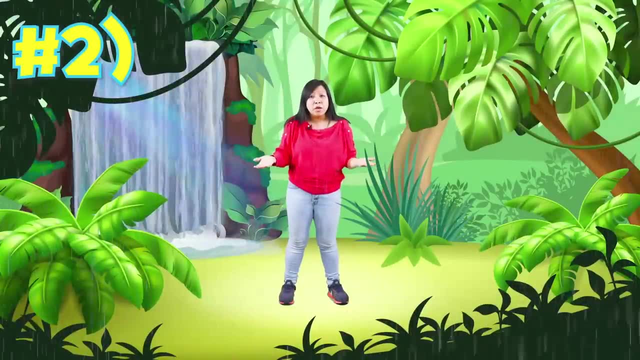 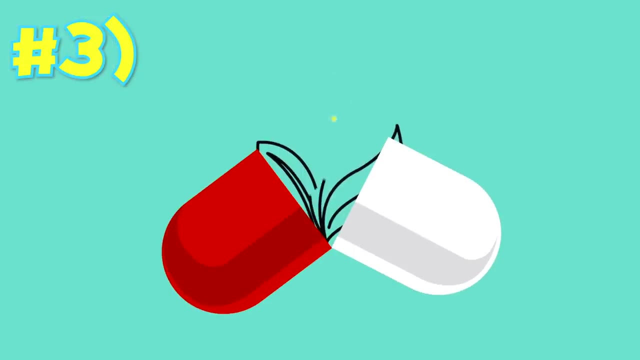 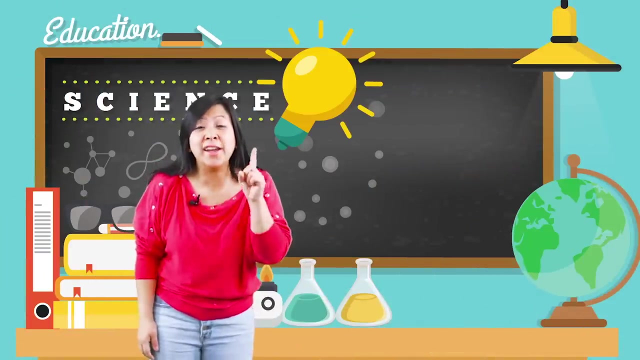 number one: the animals can't pollinate the plants, so that means we will have no more plants. number two: then the plants wouldn't exist. bye-bye plant. number three: then we wouldn't have plants to make our medicine. oh no. what could we do to help? i know one thing that we can do is build a home for animals. 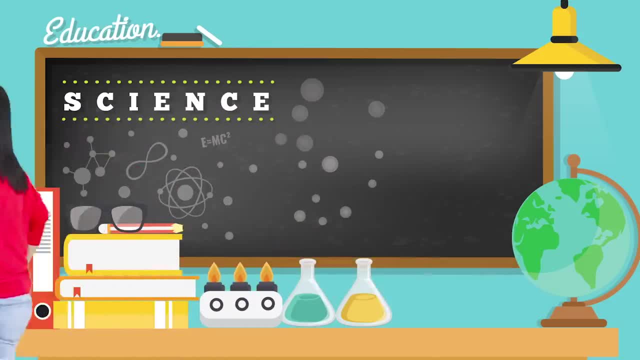 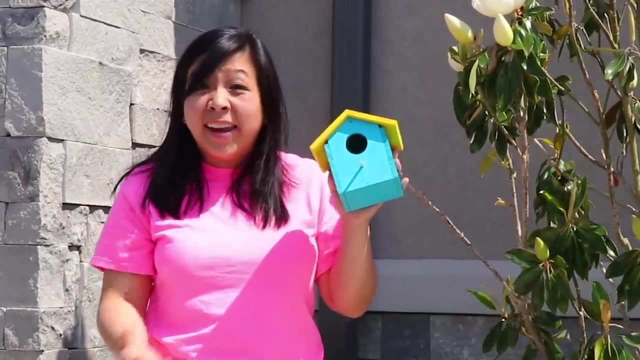 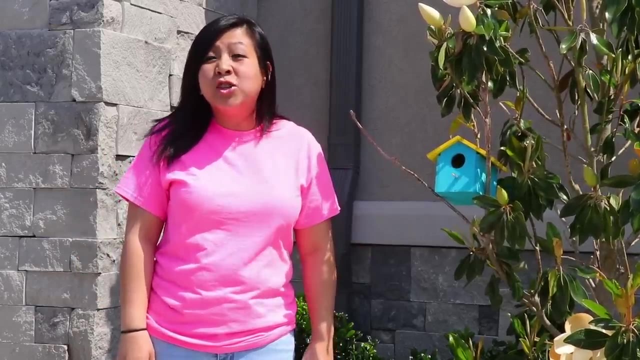 that are migrating Come on. So if you put a birdhouse like this one here, it will be a great help for birds who are migrating. We can help them get to where they need to go next and it will make their job. easier traveling and pollinating the plants. Oh look, Hi. We also need the rainforest to help us stop the ice cap from melting. Rainforests are full of trees that clean our air by converting carbon dioxide, which is what we breathe out. 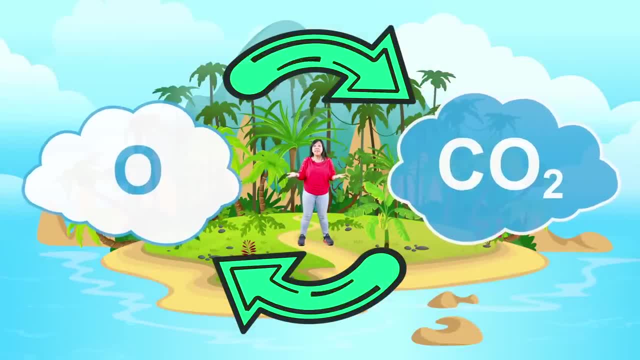 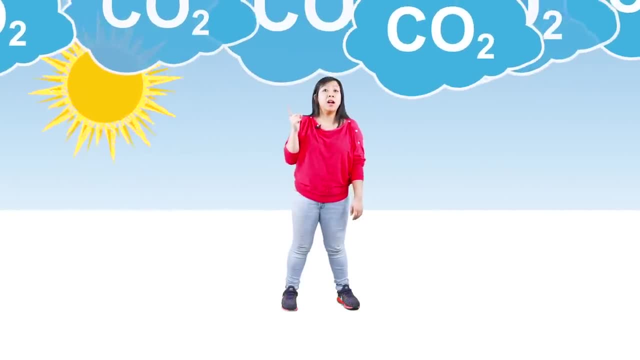 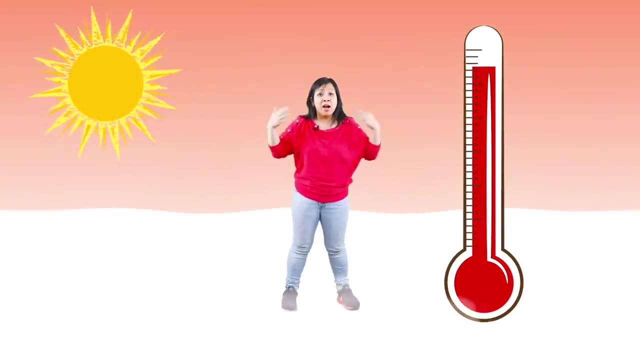 into oxygen, which is what we need to breathe. And if we have too much carbon dioxide in the air, the temperature of the planet will rise. Look, Oh, it's getting hot. And if the temperature of the planet rise, the 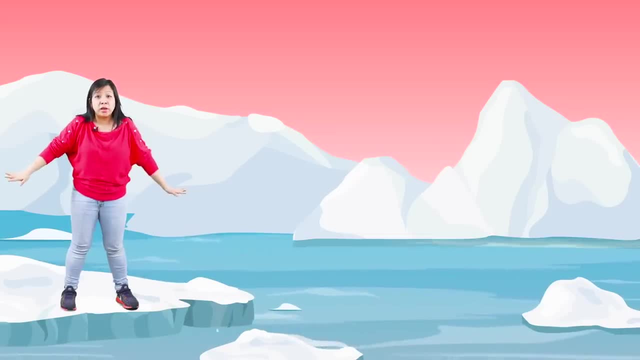 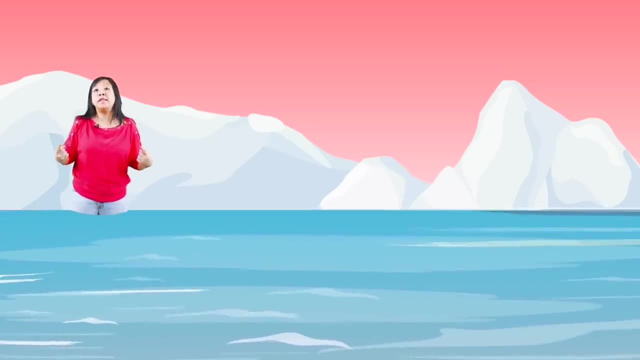 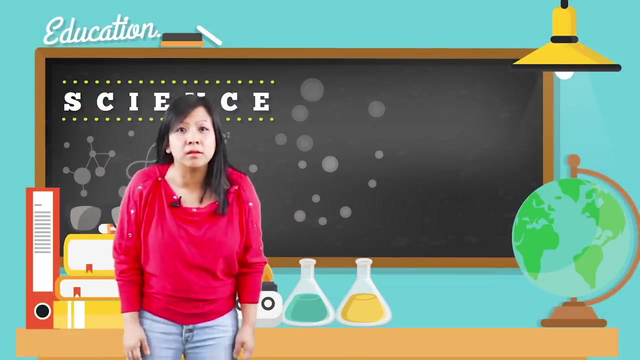 ice cap will melt into the ocean, And then the ocean level will rise. Oh no, The water is rising. Oh, let's get out. So what will happen if we let the ice cap melt? Number one water from the. 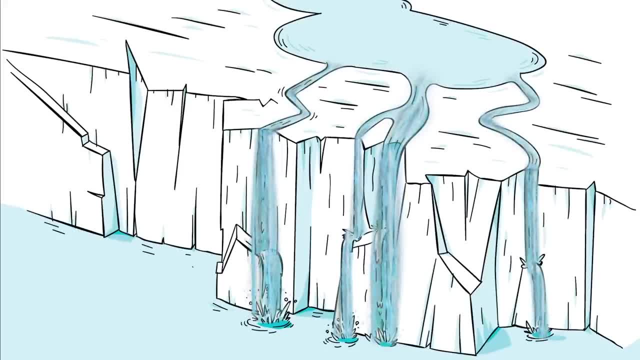 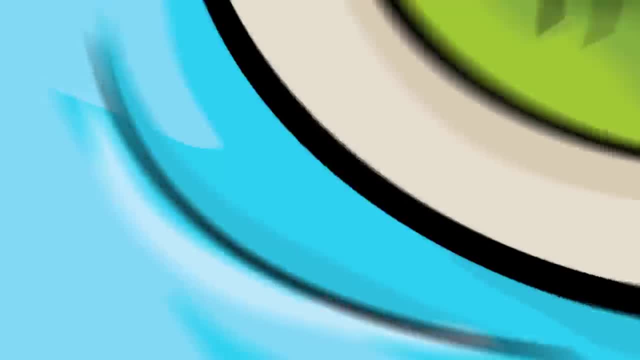 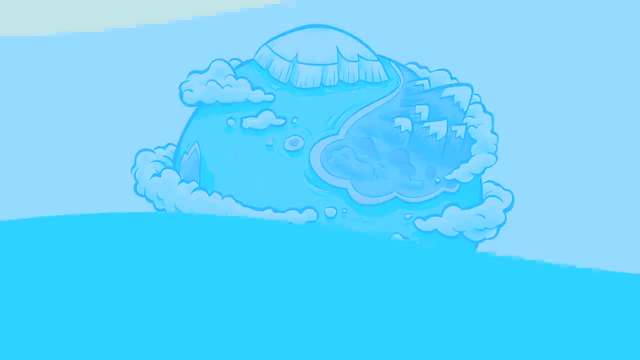 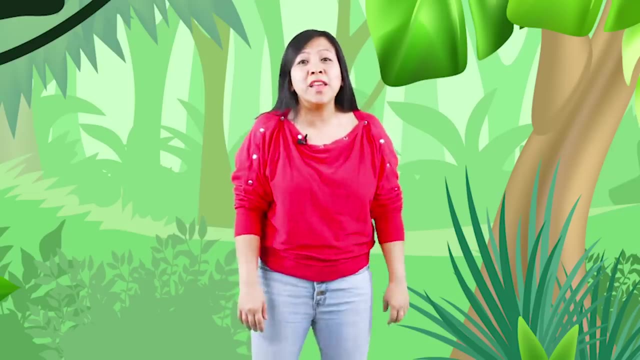 ice cap will drain into the ocean. Number two, the ocean level will rise. And number three, land around the coast and land at sea level will be covered. Whoa, That would be a lot of water, But don't worry, One of the things. 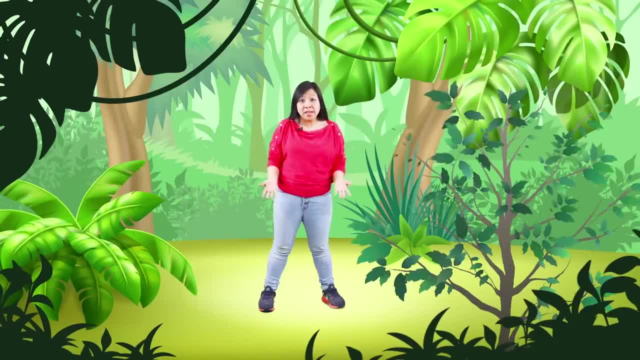 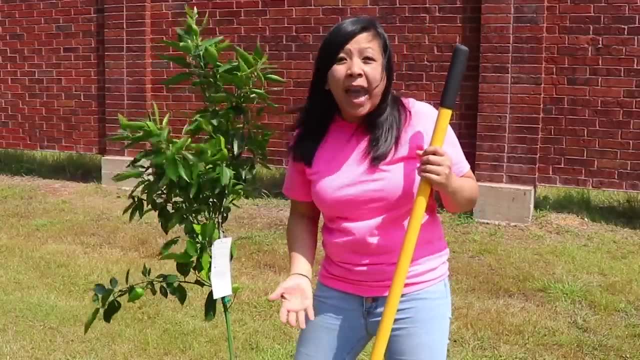 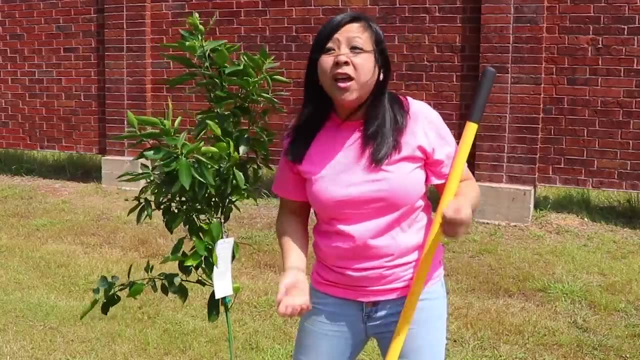 we can do is plant our own tree. Let's go So. planting trees like this one helps both the ice cap and the rainforest. This tree over here will help convert carbon dioxide to oxygen, just like all the trees in the rainforest. It's something that 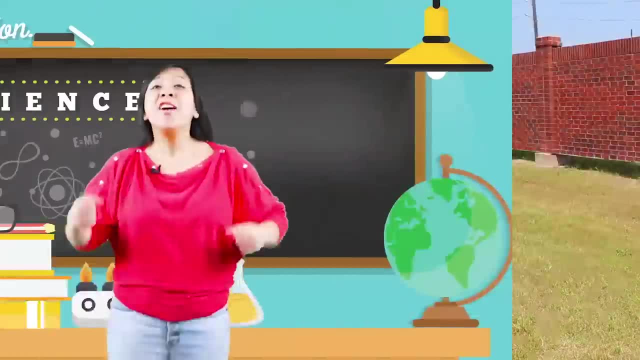 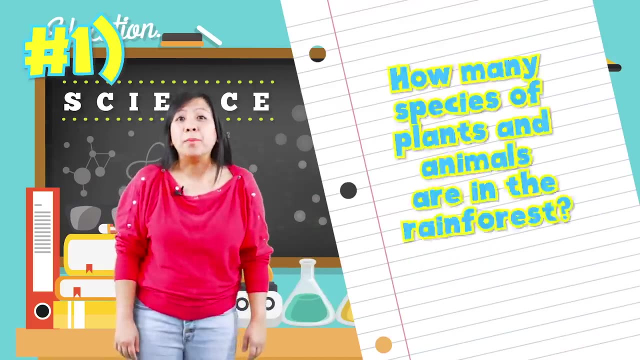 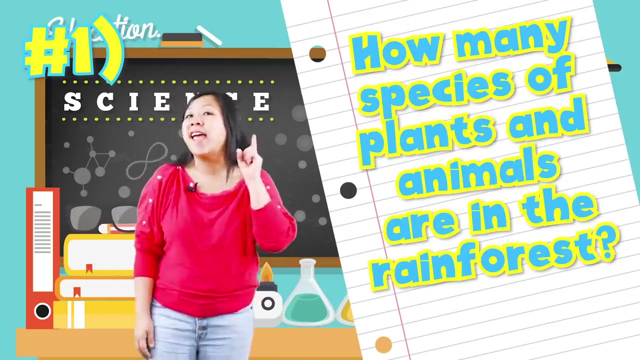 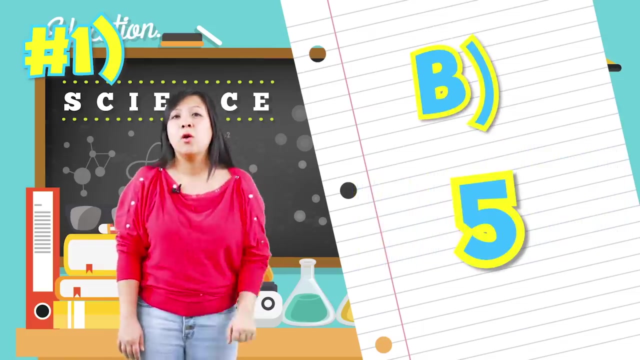 everyone can do, even you. Thanks for helping me plant a tree. now it's time for a pop quiz. Number one: many species of plants and animals are there in the rainforest. is it a- 30 million? is it b- five or is it c? zero plants and animals in the rainforest. 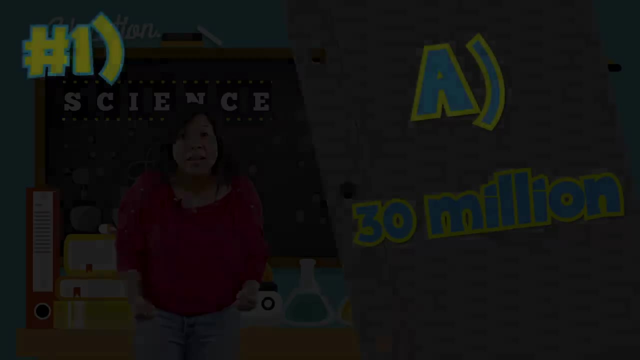 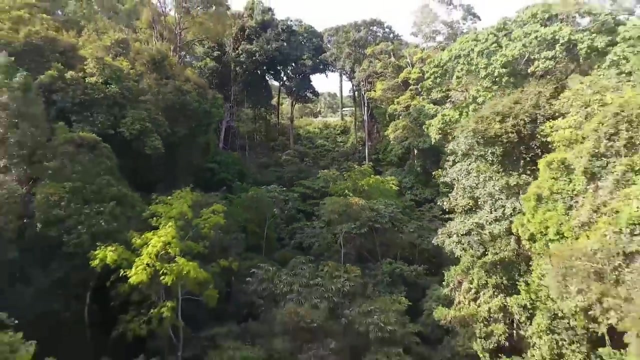 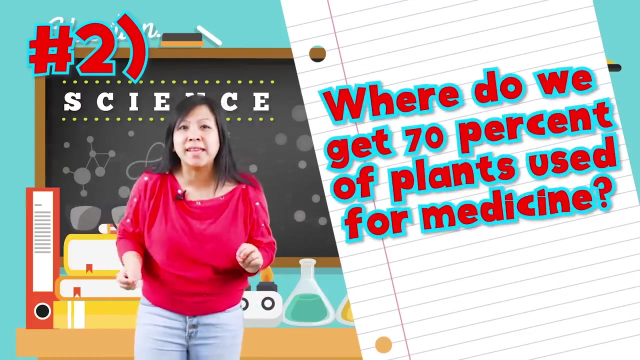 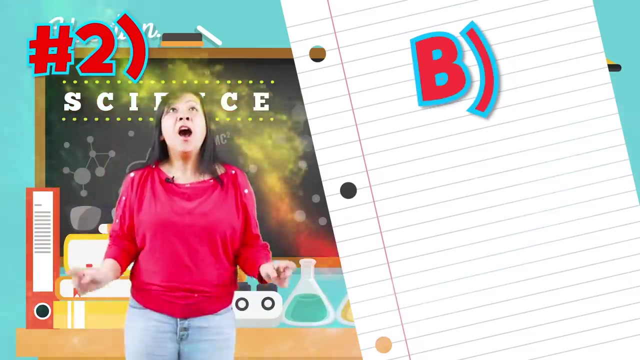 did you guess it? it is a 30 million different plants and animals that are in the rainforest. that's a lot. question number two: where do we get 70 of plants we use for medicine? is it a the rainforest, is it b the rainbow, or is it c ice? 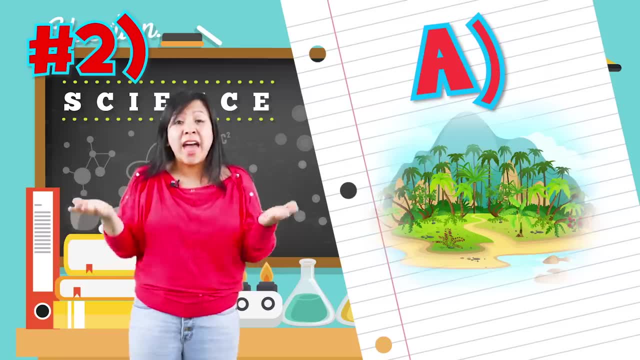 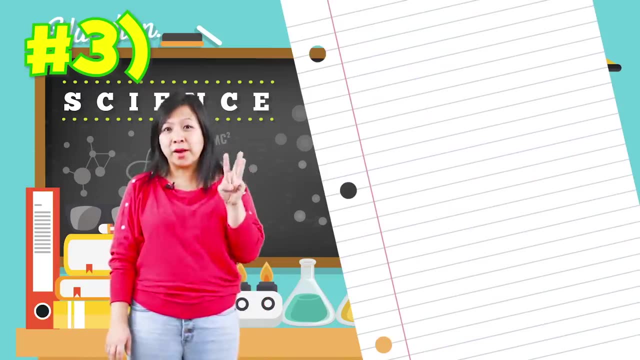 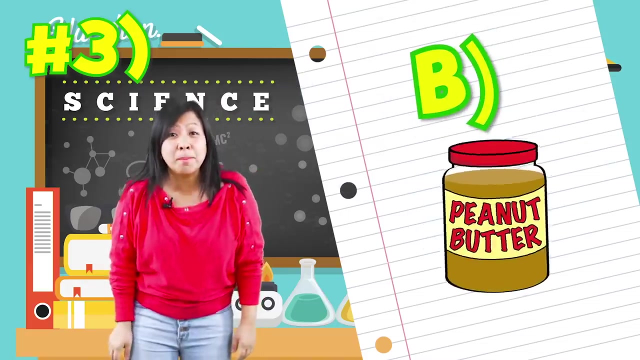 did you guess it? it is a, the rainforest. that is where we get 70 of our plants that we use for medicine. Question number three: How do trees clean the air that's around us? Is it A with hand soap? Is it B with peanut butter? I love peanut butter, They're so yummy- Or is it C? 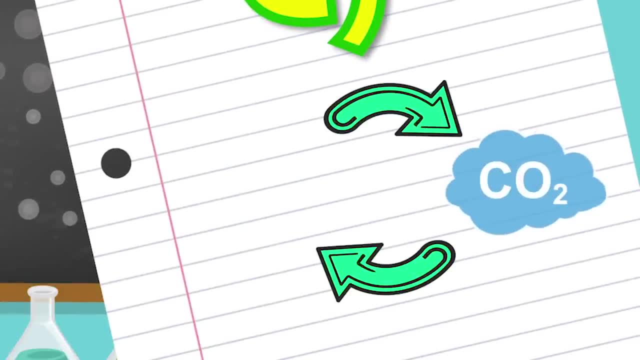 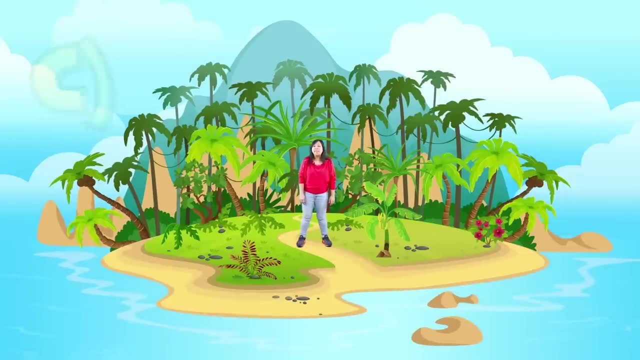 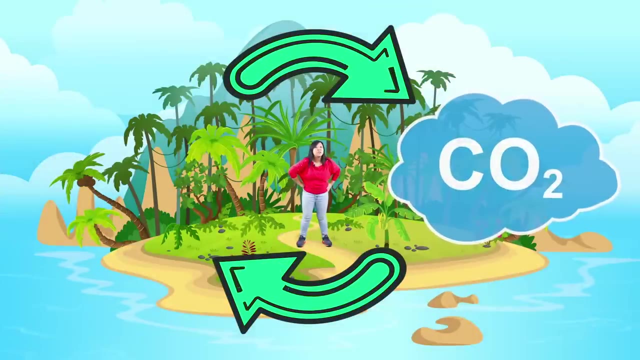 by converting carbon dioxide into oxygen. Did you get the right answer? It is C Trees help clean air by converting carbon dioxide- which is what we breathe out, which is the stuff that's not really good for our body- into oxygen, which is what we need to breathe. 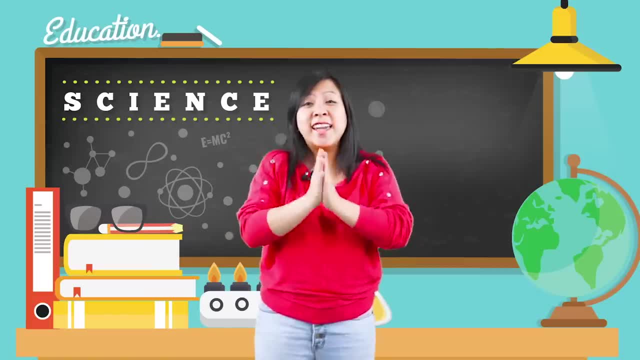 in to our body to survive. Congratulations, Good job, And if you didn't guess it all right, you can try again. Question number four: How do trees clean the air that's around us? Is it A with hand soap, Is it B with peanut butter, Or is it C? 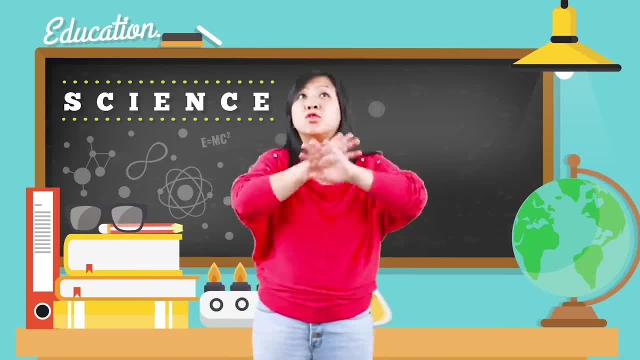 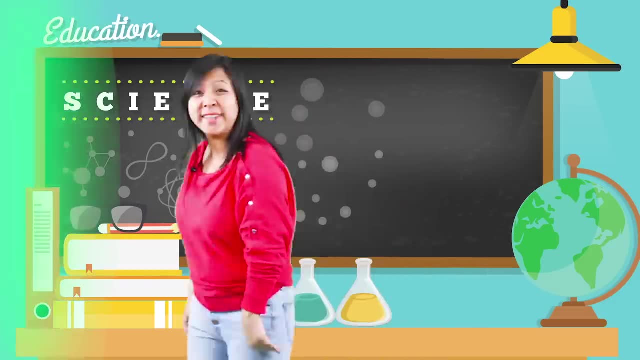 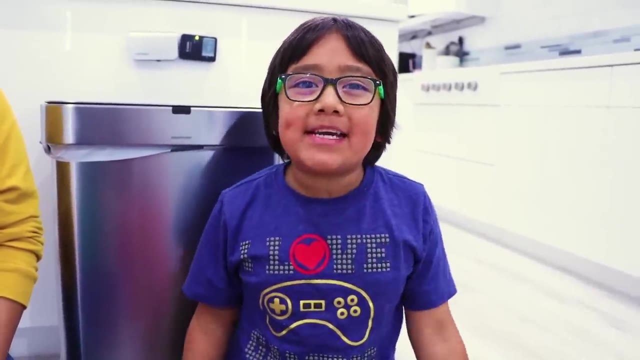 by converting carbon dioxide into oxygen. It is C. Try again next time. So now that we learned so much about ways to save the planet, let's go back and tell Ryan: Let's go. I hope you guys learned a lot of ways to save the planet. Bye, Remember, always stay happy and rise. 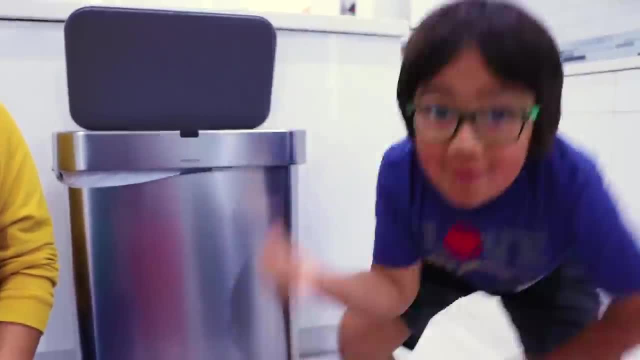 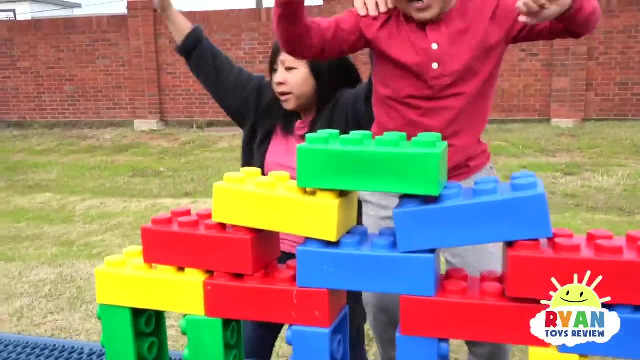 up. Bye, I'm gonna go save the planet more. Just one more piece. Yay, Oh yeah, We did. What's going on? What's going on? Oh no, the earthquake. Whoa, I gotta go. 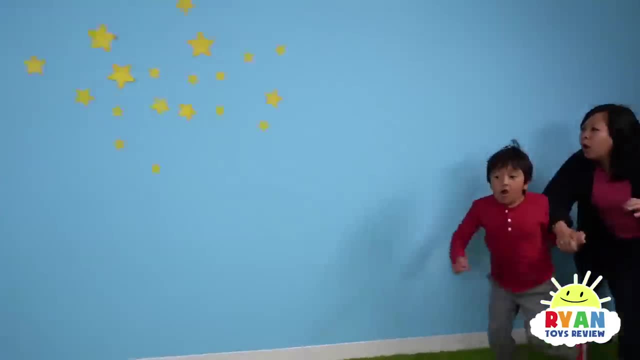 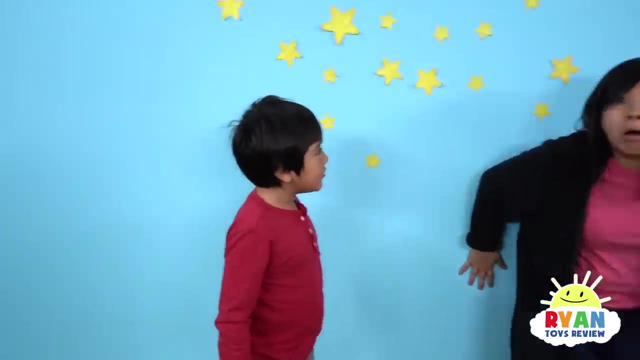 Okay, okay, Whoa, whoa. it's still shaking a little bit. I know that was a strong earthquake, Mommy, but what causes earthquakes? Good question, and what is an earthquake? right, I'm gonna explain it to you, okay. 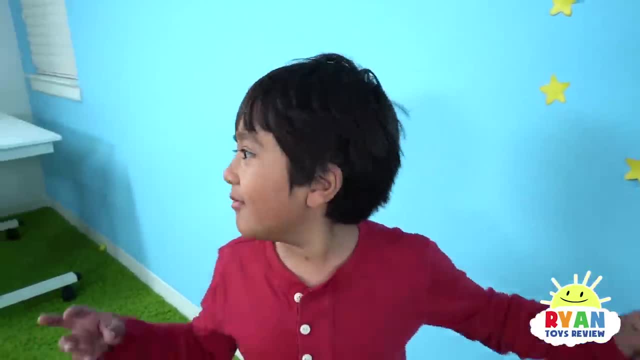 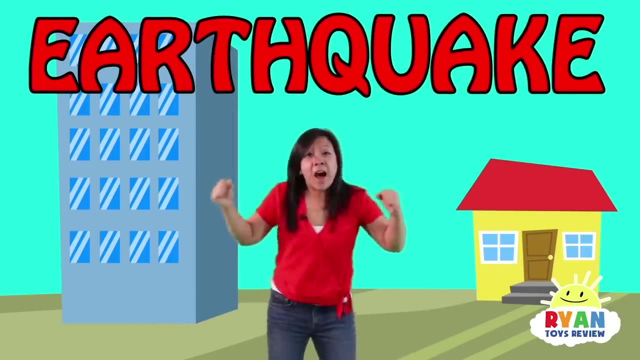 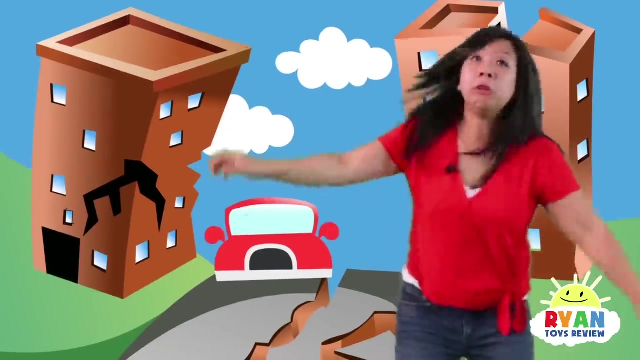 Be right back. Whoa, Where'd Mommy go? Wait, Whoa, hi there. Did you know that earthquake means there's a sudden violent shaking of the ground? But what makes the ground shake? Is it because I'm jumping up and down? 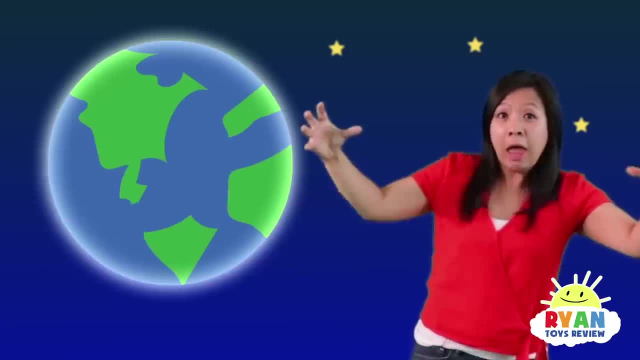 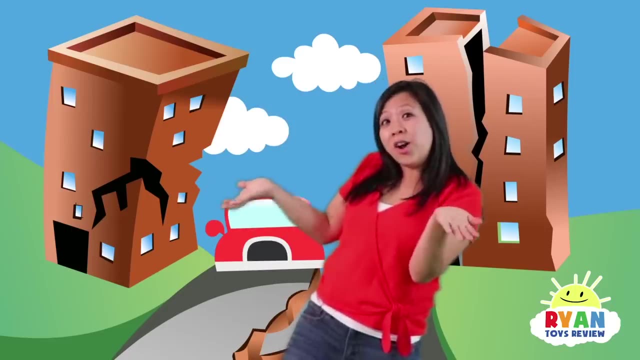 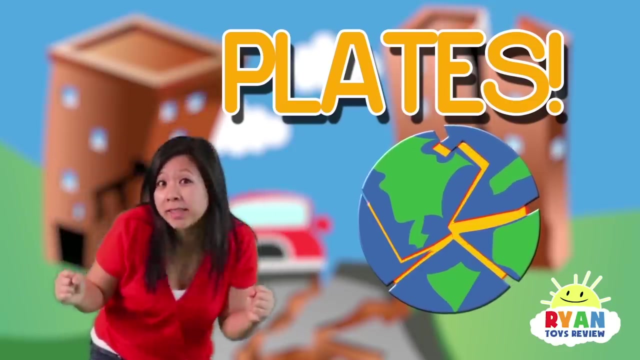 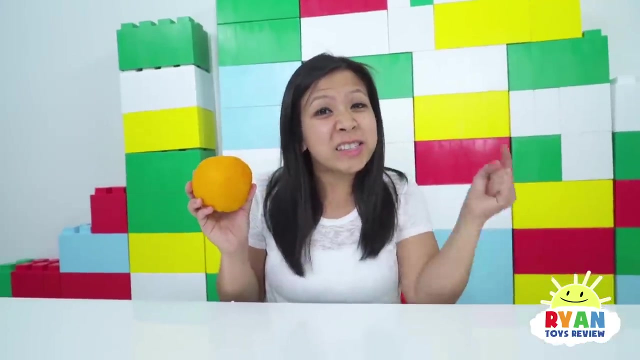 Or is it because the earth is growing bigger and bigger and bigger? Whoa? Or is it because the earth is made of plates that slide around on top of hot molten magma? Yes, that's right. The earth is like this orange. 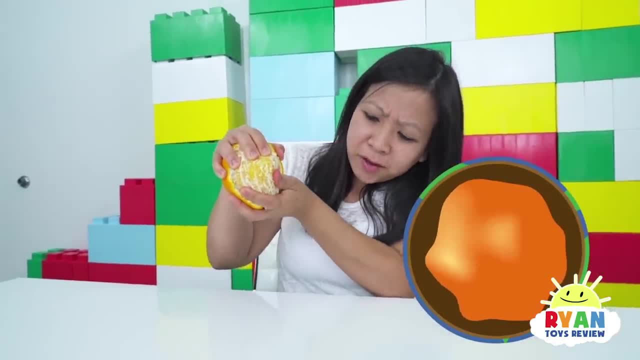 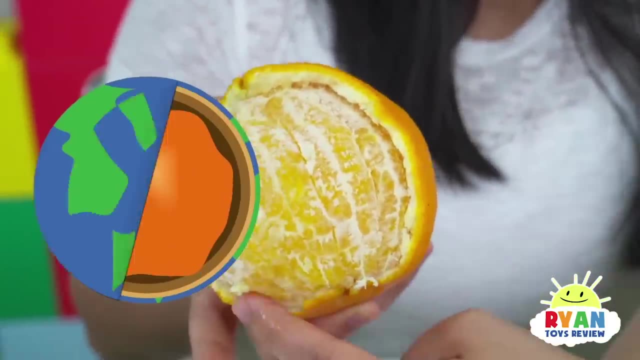 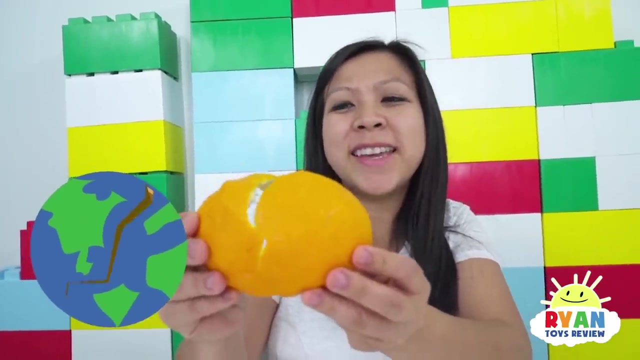 On the inside it's squishy and full of fluid- Whoa. On the outside, the orange peel is like the earth's crust: Whoo, Whoo, Whoo. The earth's crust is broken up into what we call tectonic plates. 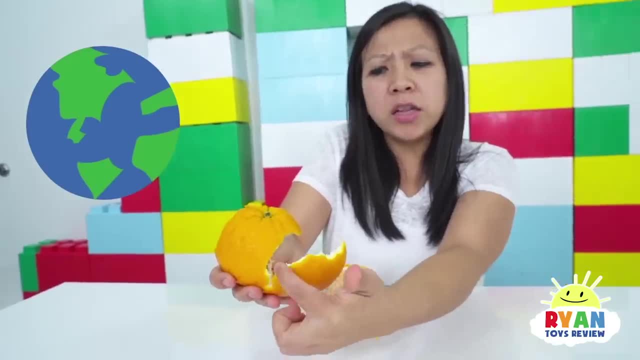 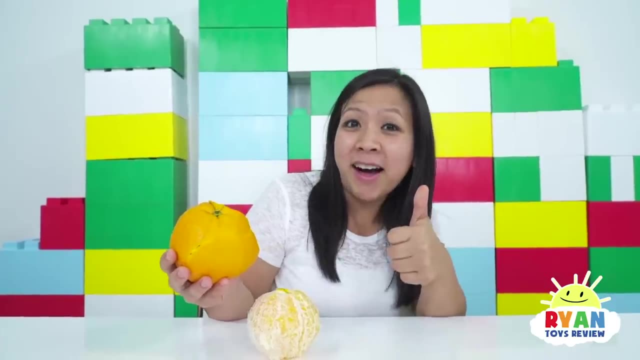 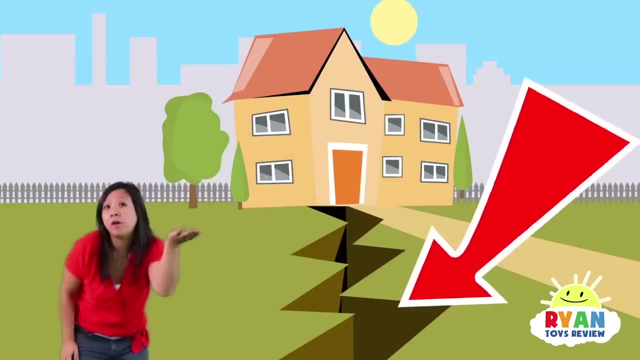 Whoa, look, they go back together All along. the cracks of the tectonic plates are where earthquake happens. Pretty cool, huh? Did you know? the place where earthquakes happen are called faults. There are three different kinds of faults that makes earthquake happens. 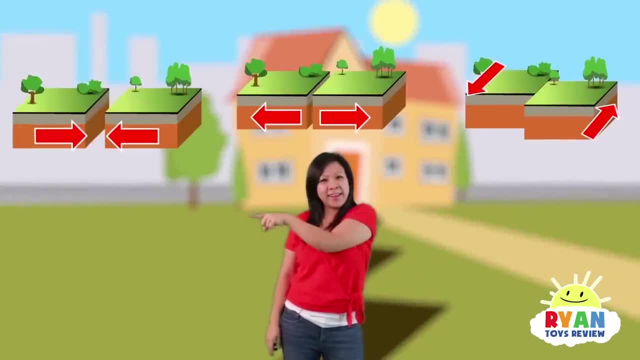 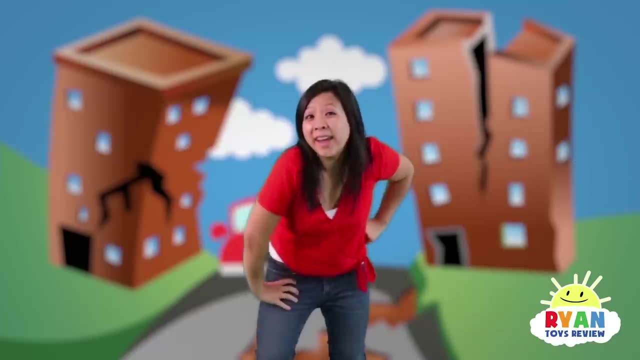 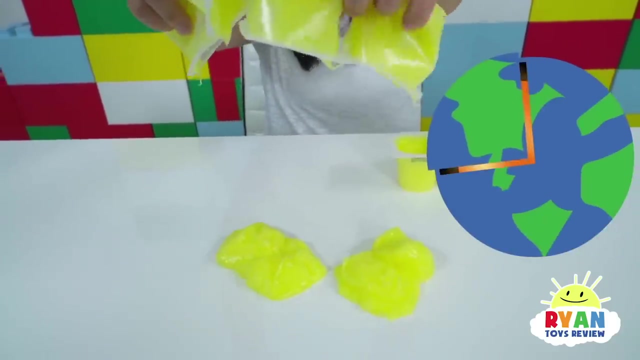 One, two, three. We are going to demonstrate how all these happens. Are you ready? Let's pretend these puddings are like the inside of the earth. The pudding is like the magma. Look how jiggly they are- Whoa. 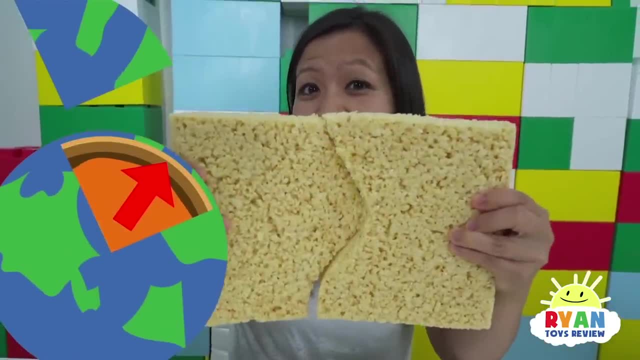 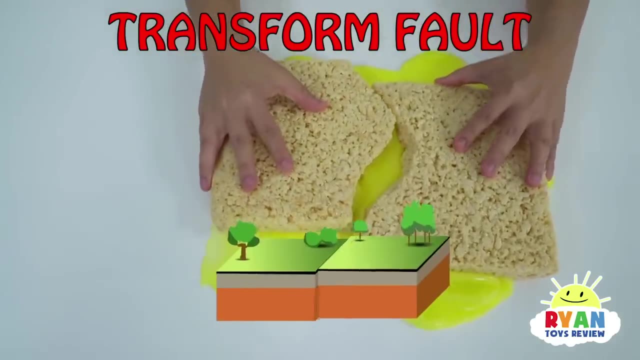 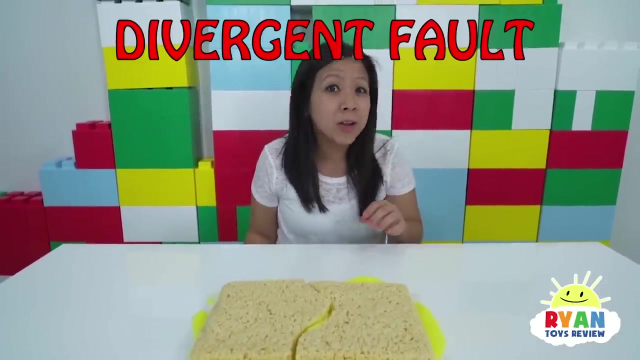 The Rice Krispies treats are like the earth's crust. The first type of fault is a transform fault. This is a transform fault. This means that the plates slide and slide past each other just like this. The second type of fault is called a divergent fault. 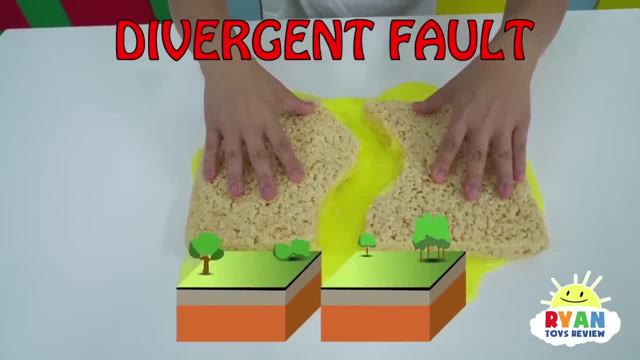 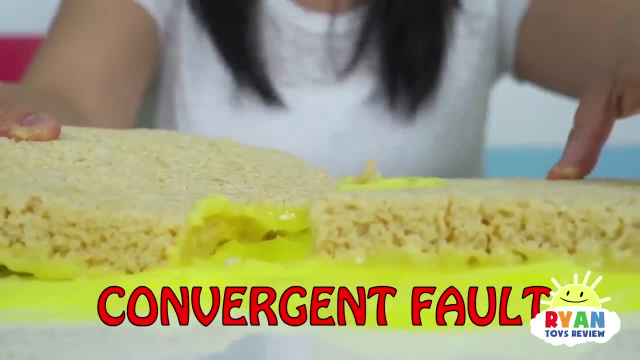 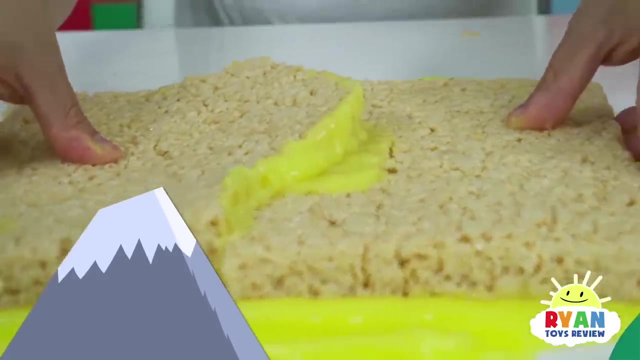 This means that the plates pull away from each other. Look, And the third type of fault is called a convergent fault. This means that the two plates push together. Whoa, This is how mountain and hills happen. Whoa. So those are the three kinds of faults. 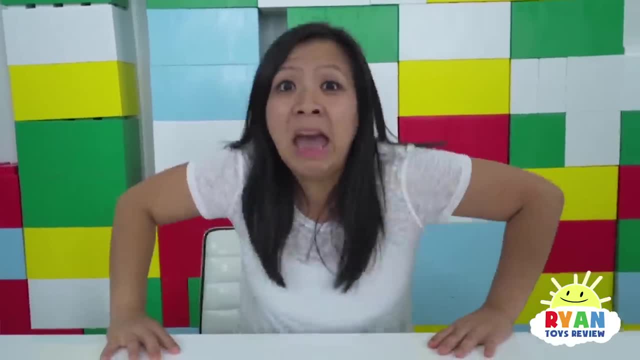 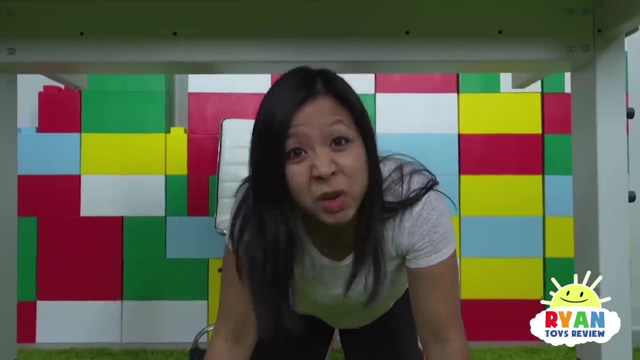 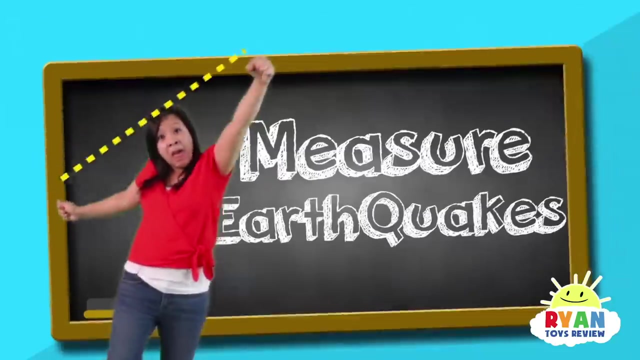 that cause earthquakes? Whoa, What is that? Whoa, Whoa. Did you guys feel that That was a real earthquake? I wonder how big that one was. Did you know that you can measure earthquakes? They get score on how strong they are. 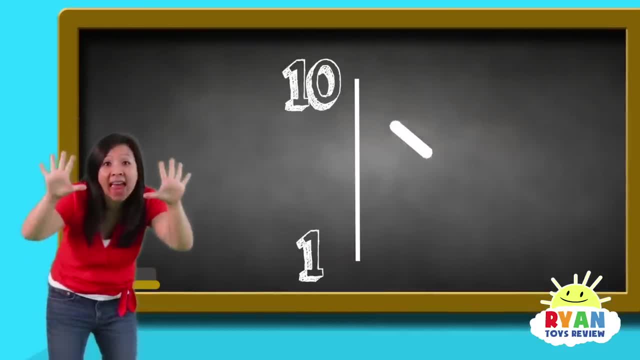 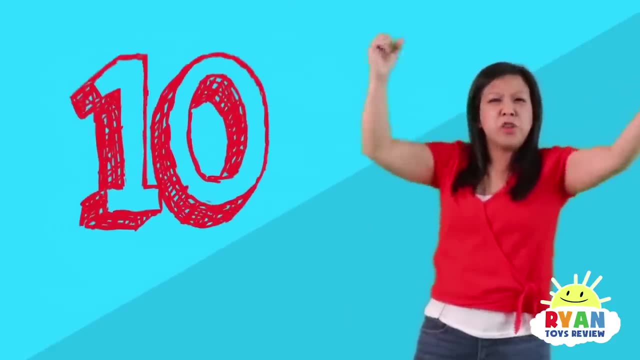 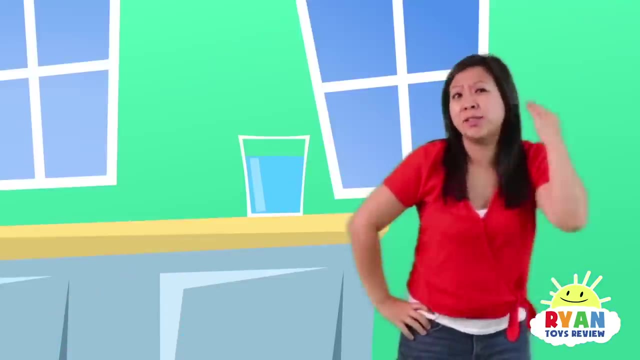 And they go all the way up, All the way to 10 on what is called the Richter scale. The bigger the number, the stronger the earthquake. Whoa, So an earthquake that measures a 2.5, whoa, whoa. is smaller and it doesn't cause as much damage, But an earthquake that measures an 8.5,. whoa whoa is smaller and it doesn't cause as much damage, But an earthquake that measures an 8.5, whoa, whoa, whoa. 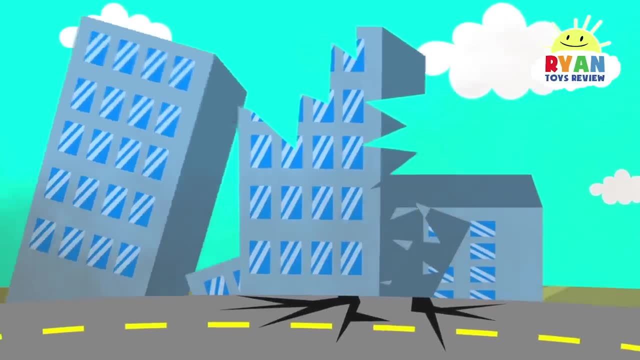 is smaller and it doesn't cause as much damage, But an earthquake that measures an 8.5,. whoa, whoa, whoa is smaller and it doesn't cause as much damage, But an earthquake that measures an 8.5, whoa, whoa, whoa. 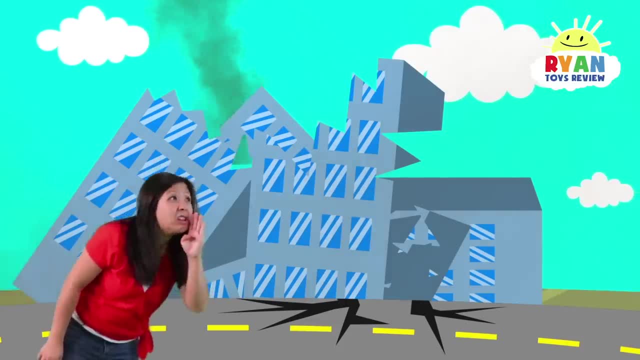 is smaller and it doesn't cause as much damage. And such a large earthquake can cause an 8.5,, but it doesn't cause as much damage. So what is an earthquake in real life? Let's go and check out an earthquake. 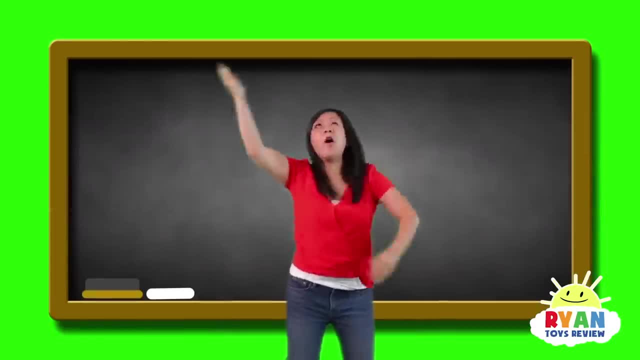 Whoa, Whoa, Whoa, Whoa. Do you guys see That is a lot of damage. So now that we have all this amazing knowledge on earthquakes, it's time for a pop quiz. Are you ready? Question number one: why do earthquakes happen? 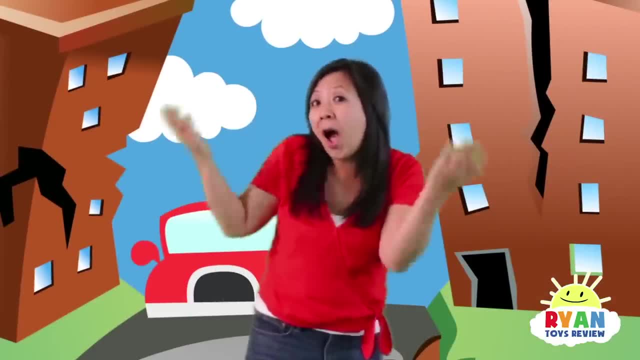 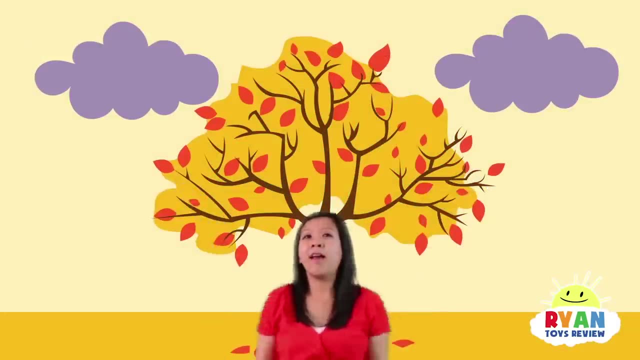 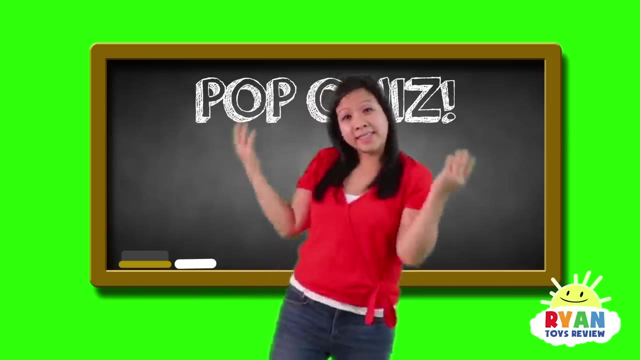 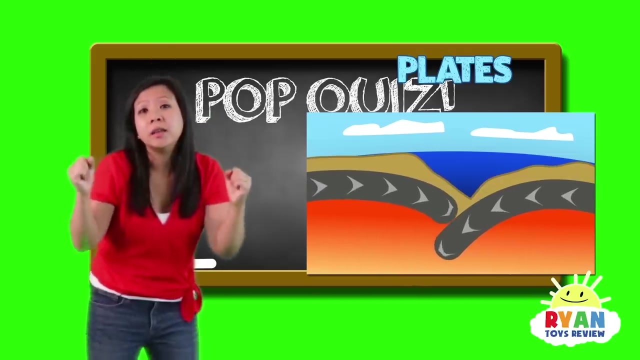 A. is it because the seasons change? Yeah, Why does an earthquake happen? Why do earthquakes happen? A- Is it because the season changed? B? Is it because the earth is so bored Or is it because? C? Earth is made of plates that slide around on top of hot, molten magma.